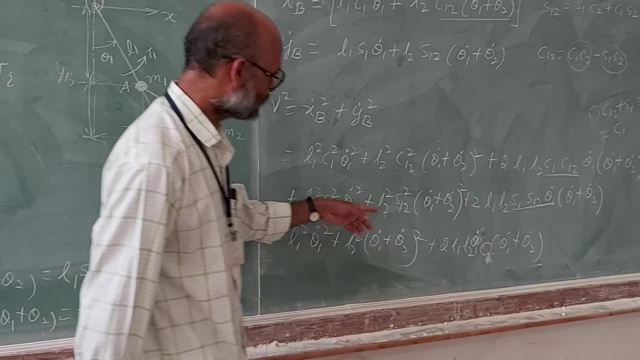 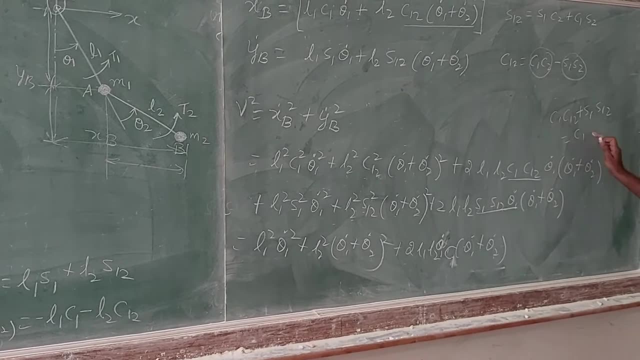 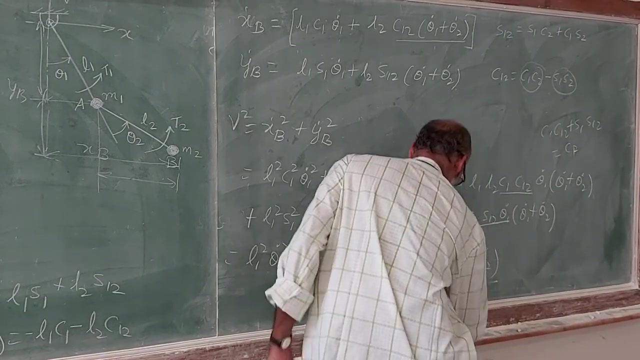 C1, C12, plus S1, S12.. I have written this as C1, but it is actually C2.. If you figure out, you get this as C2.. And that C2, we will write here. So you have 2, L1, L2, theta. 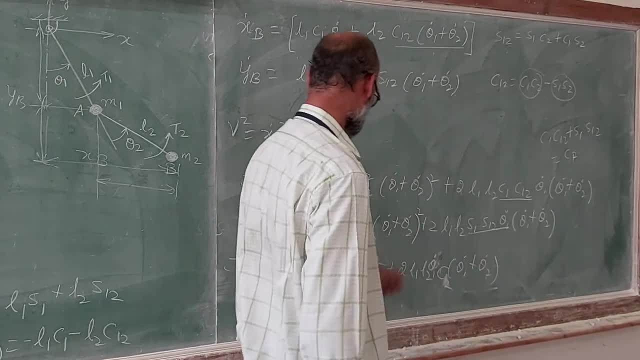 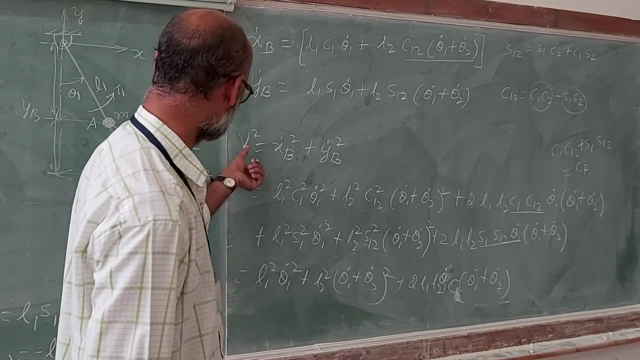 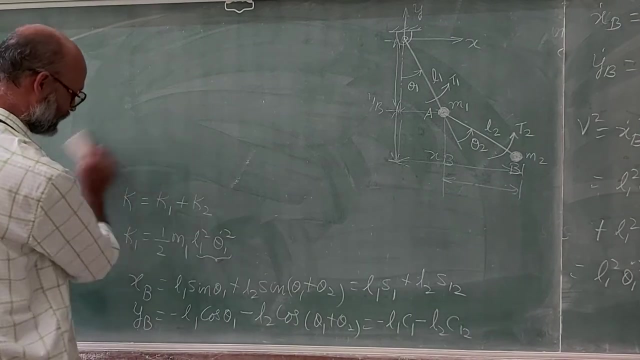 1 dot, C2, theta 1 dot plus theta 2 dot. This was square, Please see. whatever you have written square, This is square of that. So this is the equation for velocity of this. Now to write the kinetic energy for this K2.. So what is this K2?? K2 is half m2.. This: 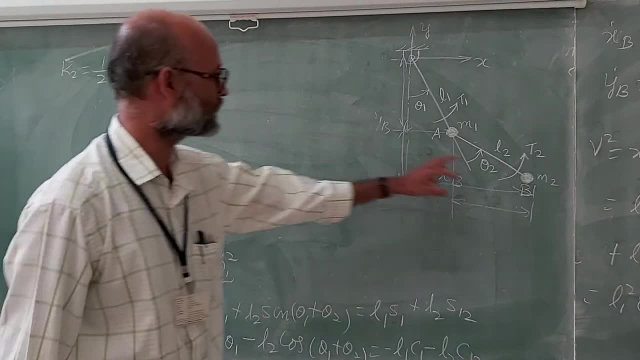 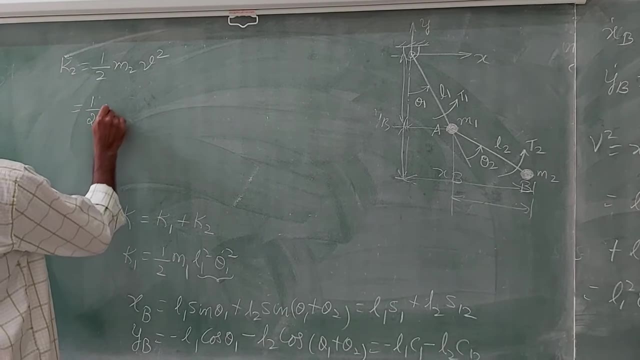 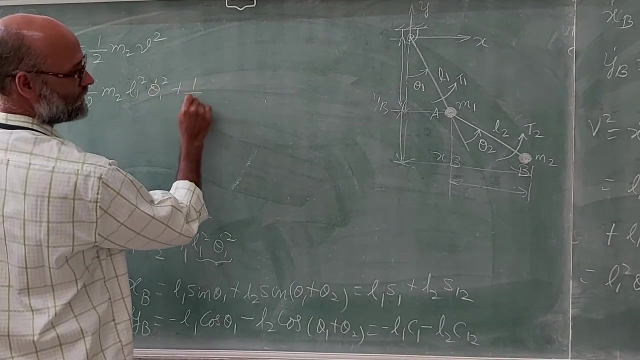 is V square. That is the total kinetic energy for the second mass. But V square is that equation. We just substitute that equation. This is half m2.. We just use that equation. This is L1 square, theta 1 dot square plus half m2, L2 square. 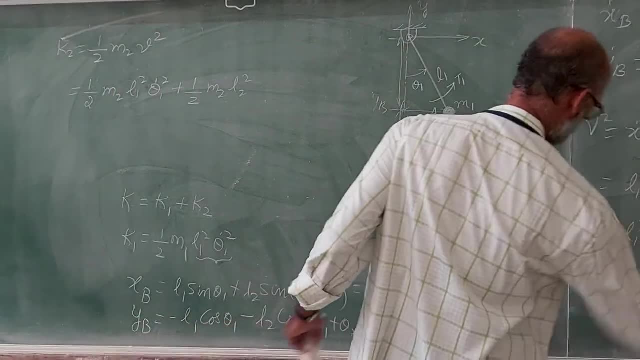 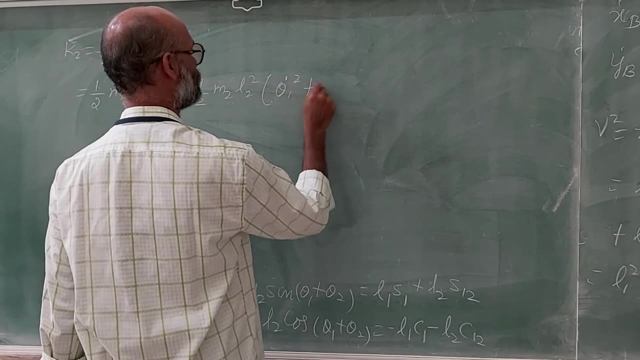 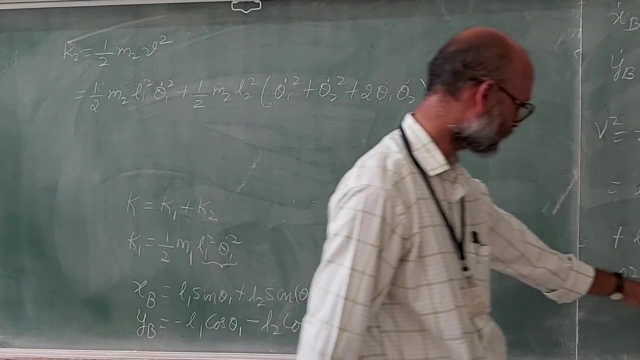 That I will expand. whatever the equation is there, This one is a plus b plus b. This way we just expand that. So if you expand that, that will be theta 1 dot square plus theta 2 dot square plus 2. theta 1 dot- theta 2 dot. That is the expansion for this term And of 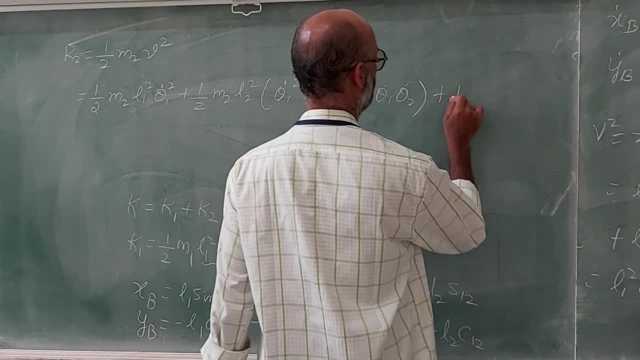 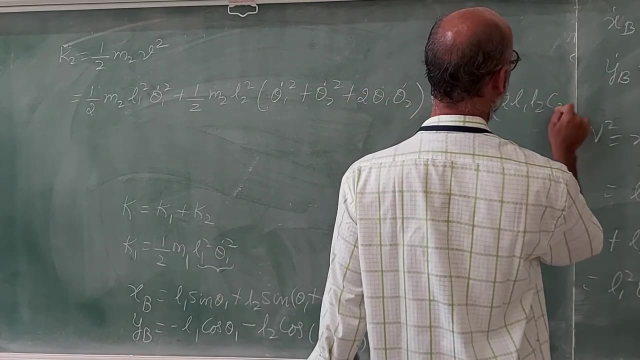 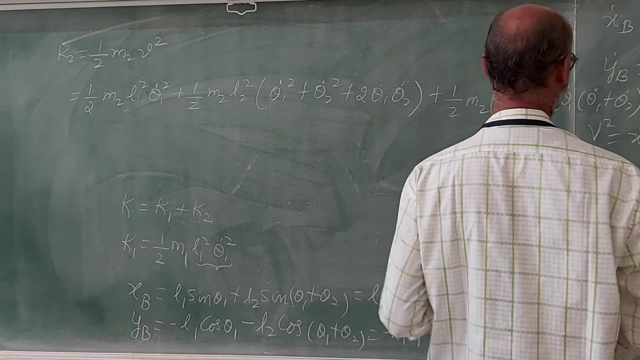 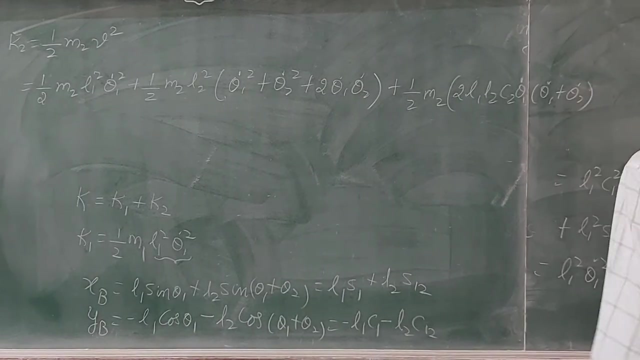 course we added m2.. So now you can see that I have 2 m2 there, plus you know that half m2, into 2 times You have L1, L2, c2, theta 1 dot multiplied by theta 1 dot plus theta 2 dot. So this: 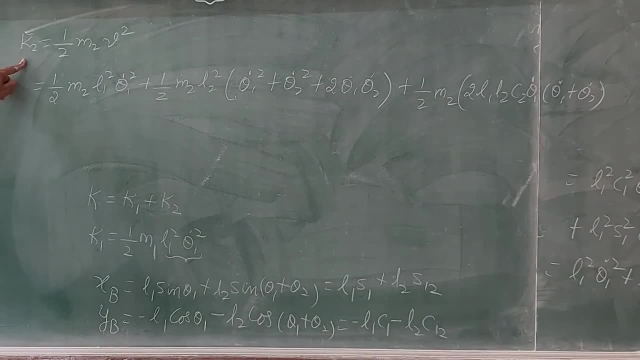 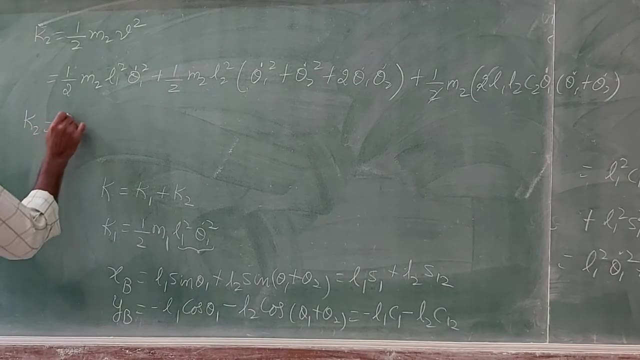 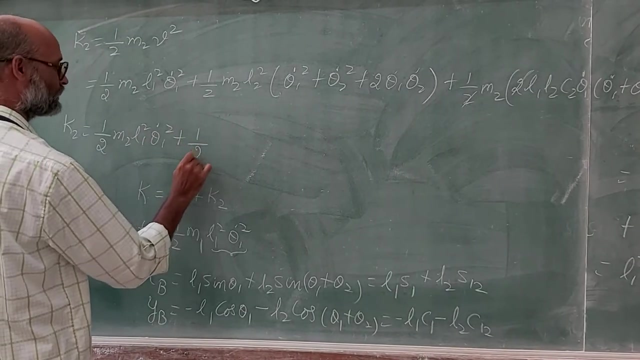 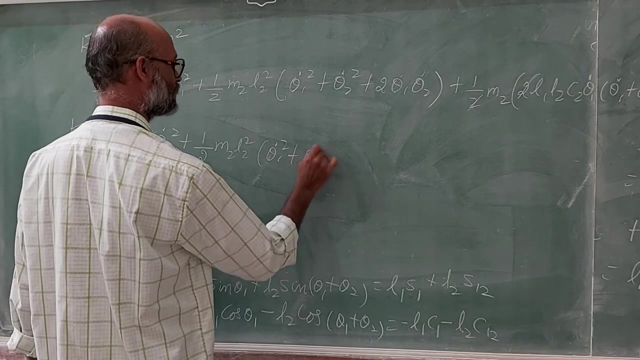 is the equation for K2.. And you can just simplify this: This: 2 m2 square theta 1 dot, you can just take it out So totally table will be half m2 l1 square, theta 1 dot square plus half m2 l2 square. you have that theta 1 dot square plus theta 2 dot square plus. 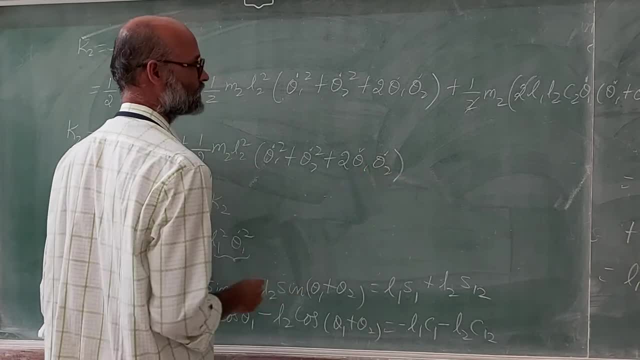 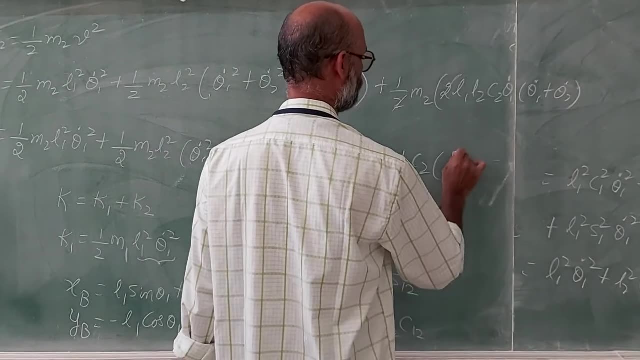 2: theta 1 dot plus theta 2 dot plus. you have this as m2, l1, l2, c2, you have theta 1 dot square plus theta 1 dot into theta 2 square. There is expansion of this theta 1 dot into. 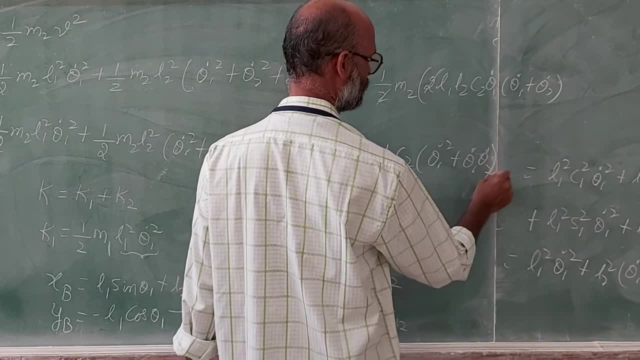 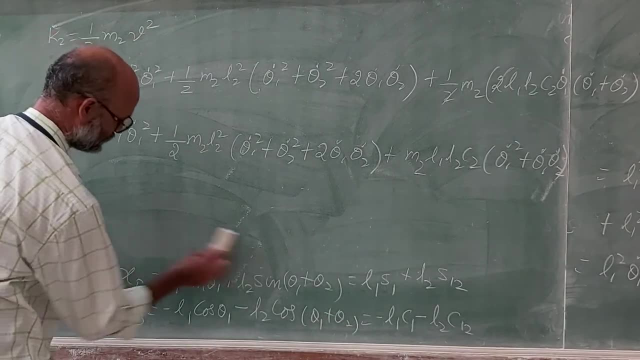 theta 1, it is theta 1 dot. square theta 1 into this. this is theta 2 dot. So that is your k2.. Now we can write total kinetic energy for the system. So let us write that. 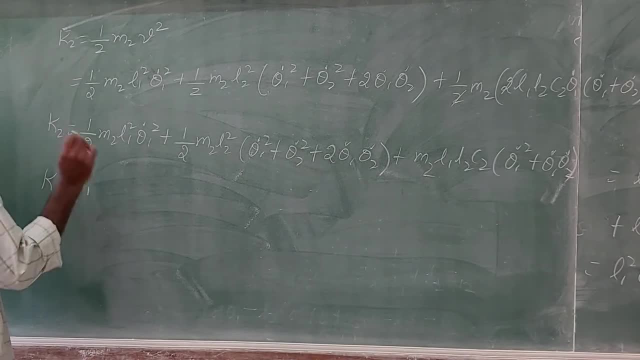 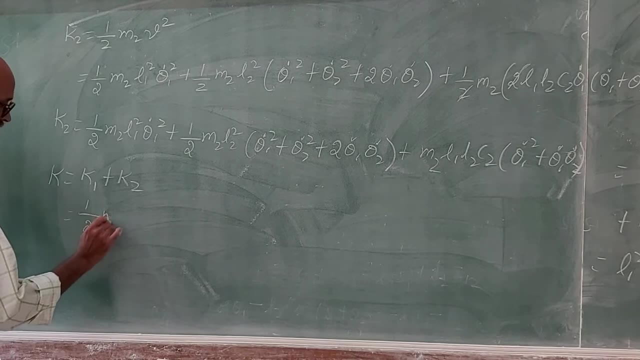 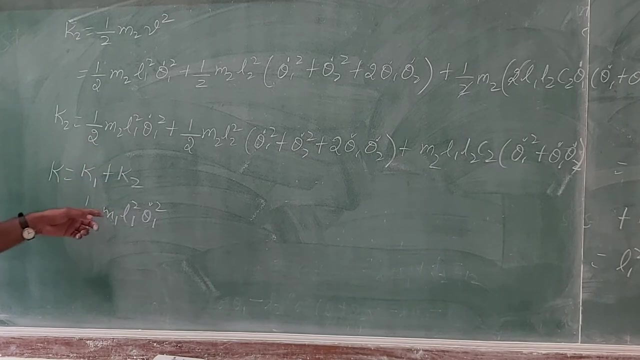 So total kinetic energy is k. this is consisting of kinetic energy at the first mass plus kinetic energy of the second mass. What is k1?? This is r, m1, l1 square, theta 1 dot square. that is k1, which is not there in the board, but you can figure out. you have written that. 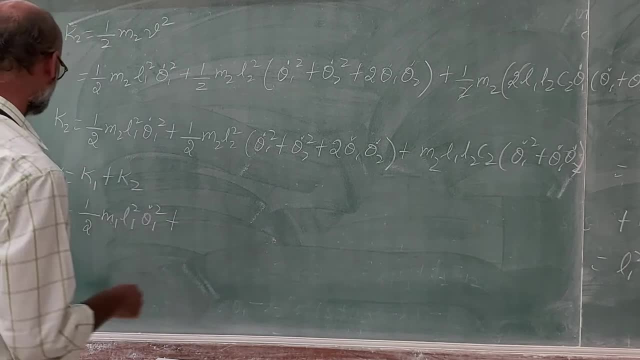 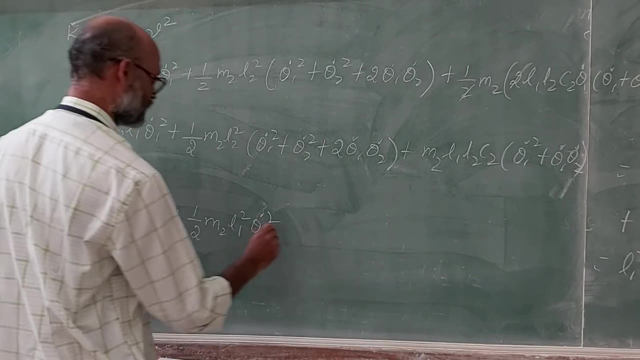 plus whatever board term is there, that is your kinetic energy of the system. So half m2 l1 square theta 1 dot square plus theta 2 dot square plus theta 2 dot square, you have this as m2 l1 square theta 1 dot square plus theta 2 dot square plus theta 2 dot square. 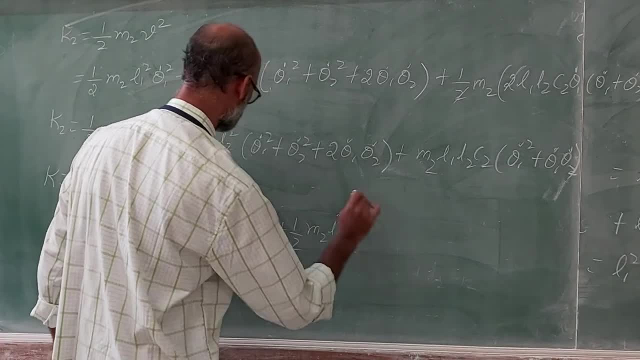 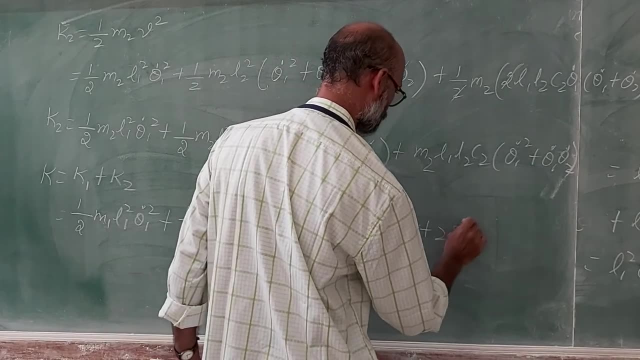 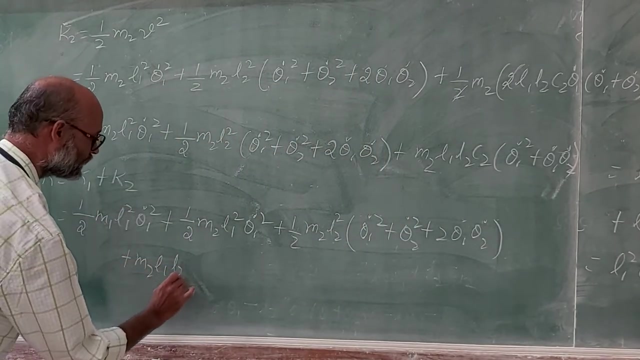 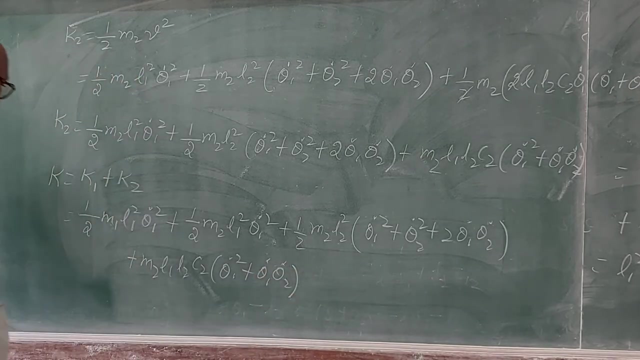 half m2 m2 square, you have this as theta 1 dot square plus theta 2 dot square plus 2 theta 1 dot. theta 2 dot plus the last term. you have m2 m1 m2 m2. theta 1 dot square plus theta 1 dot into theta 2 dot. 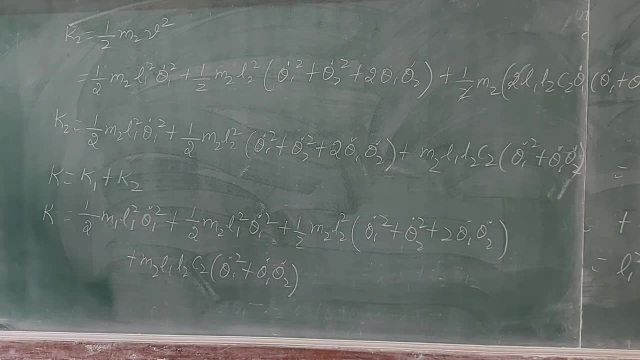 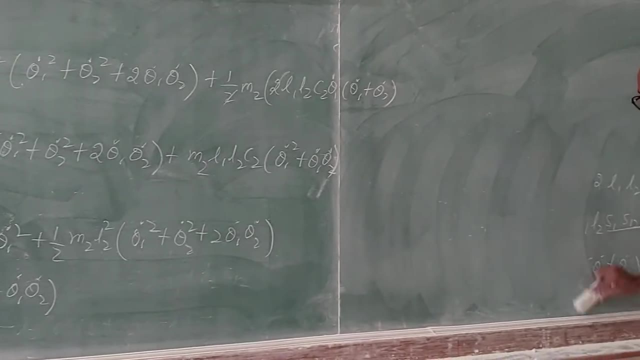 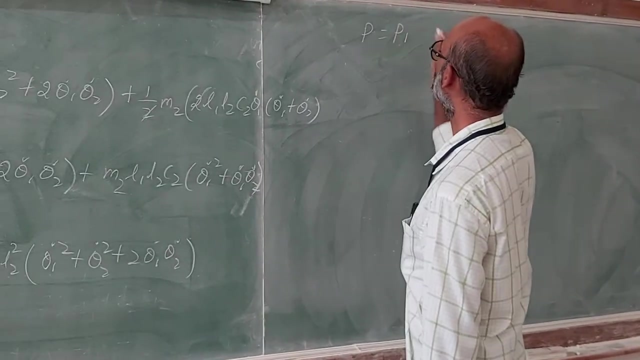 and this is the expression for kinetic energy of the system. now we evaluate what is the potential energy for the problem. potential energy is due to elevation, so let us write that potential energy is given by p. it is also, I have to count, with p1 plus p2, so what? 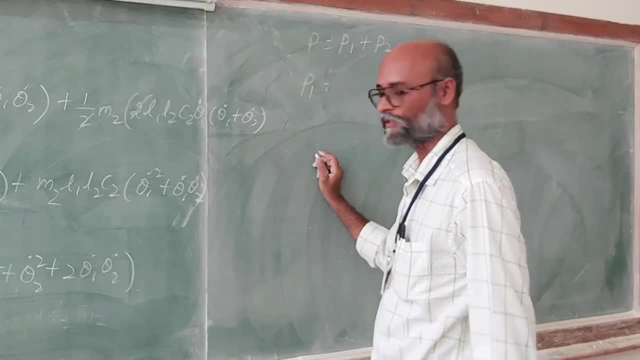 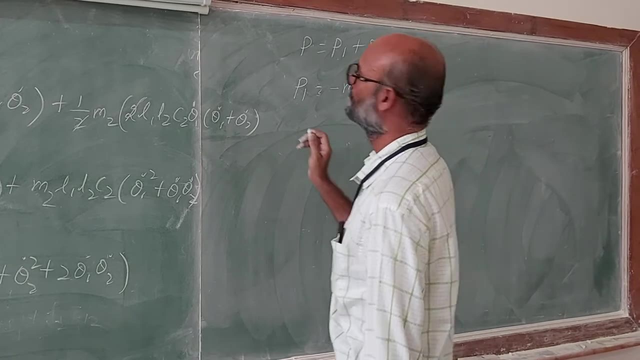 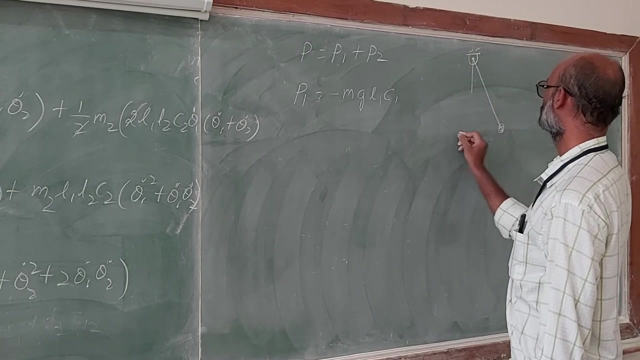 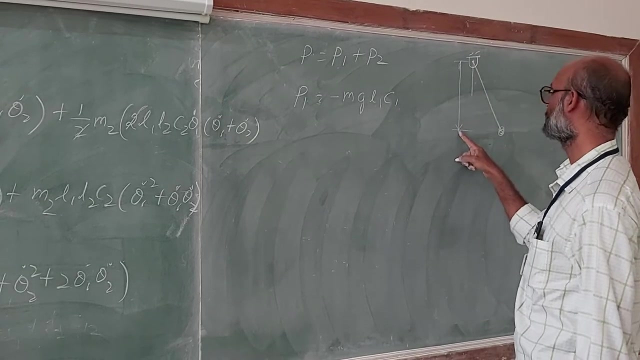 is p1. if you look at that, that is the potential of the first mass. so that is minus mg l1, m1, c1, meaning if you look at the problem, the fixation point is this: this is the first mass and taking this, this is mgh h is nothing but l1 cos theta. this is your m1, similarly. 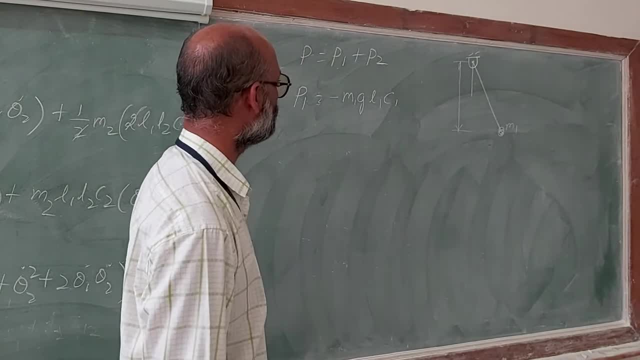 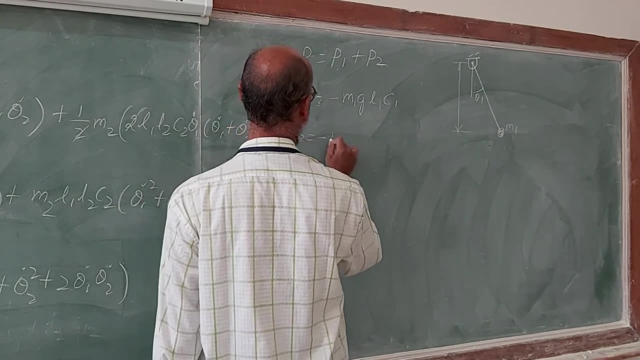 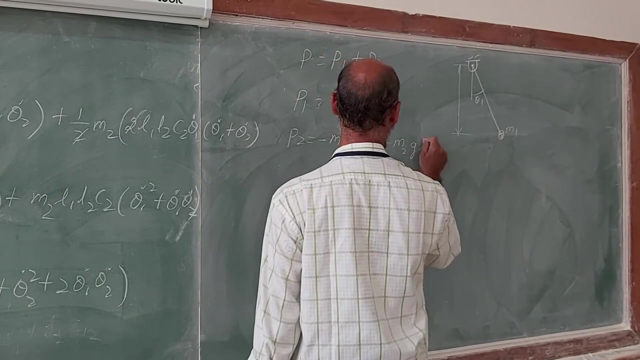 whatever, this is m1. I have derived m1, g, l1, c1, so this is your theta. now, what about p2,? this is minus m2, g, l1, c1,. this plus the next one minus m2, g, l2, c1, this is: 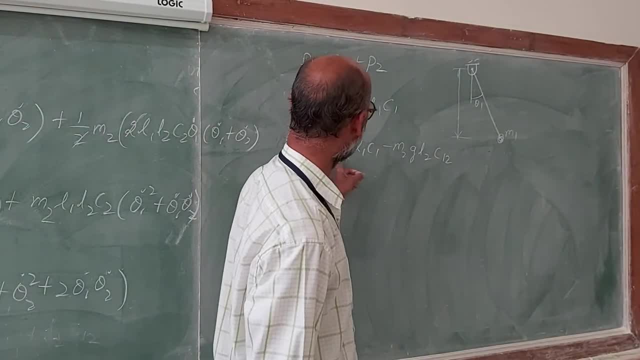 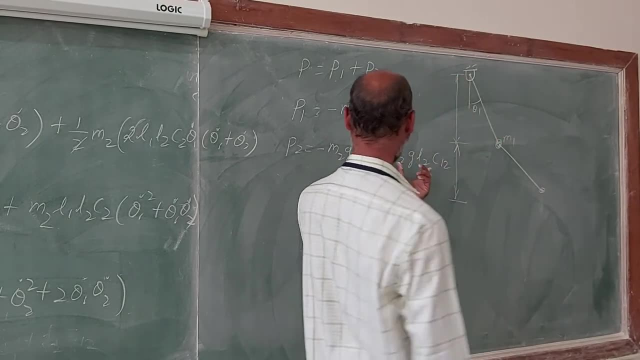 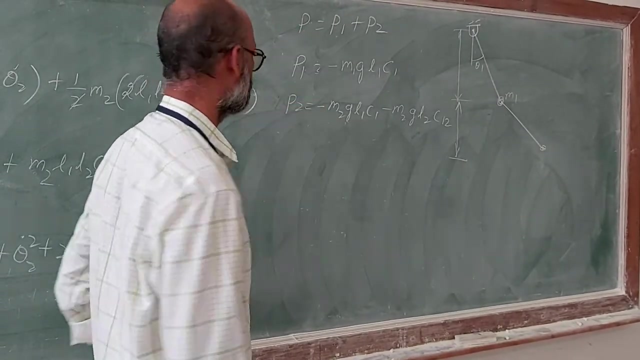 the potential. this term is nothing but this. this is elevation up to here. and if you want to take the second thing, this elevation is here, is this. whatever the term I have written here, it is this elevation. so you have p1, p2 combined together. you can just write what. 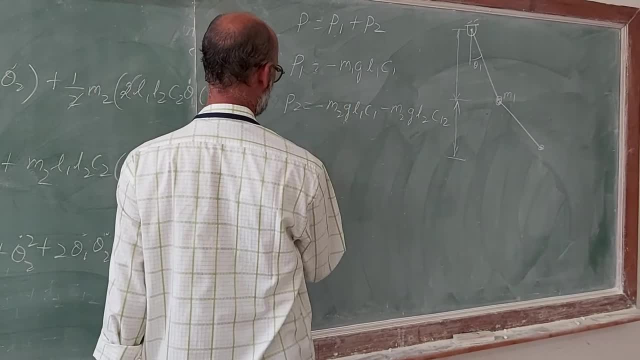 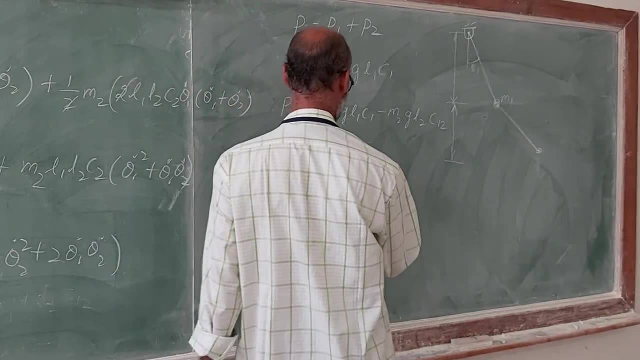 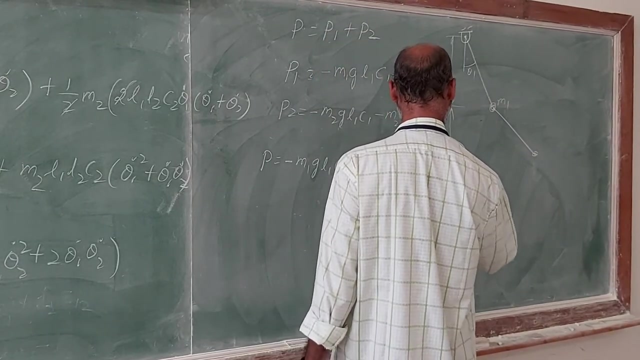 you want. So what is the potential energy? this is this plus this. this is minus m1, g, l1, c1, that is the potential energy plus mass, minus m2, g, l1, c1,, minus m2, g, l2, c1, so that 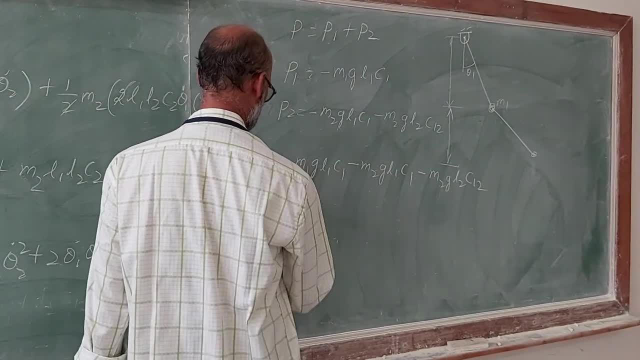 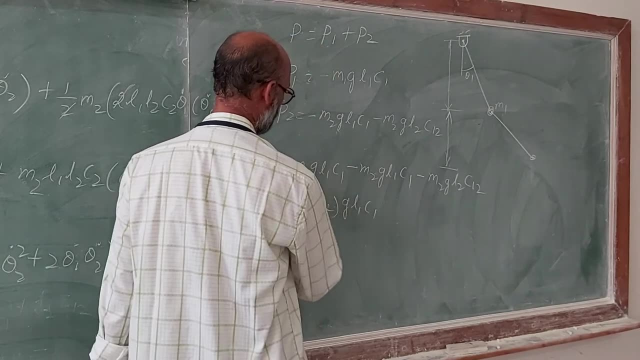 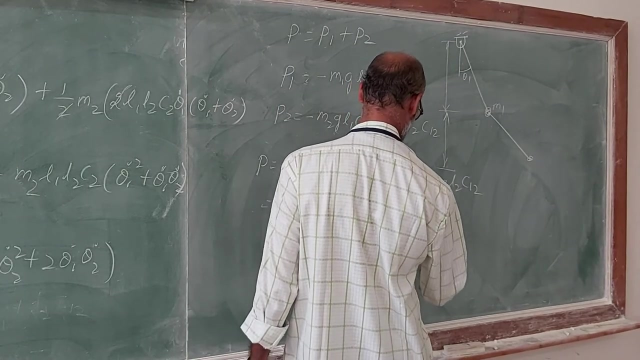 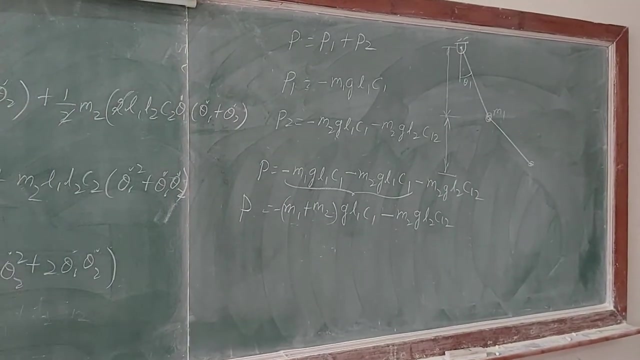 is the total. I can simplify this because this is common. you have m1 plus l2, it is minus m2, g, l2, c1, this is the expression for potential energy of the system. you have got kinetic energy of the system. you have got potential energy of the system. now you 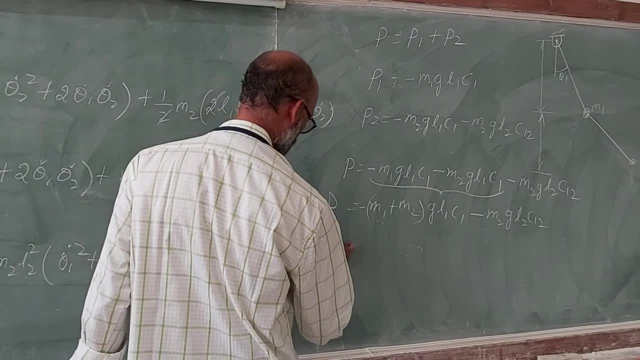 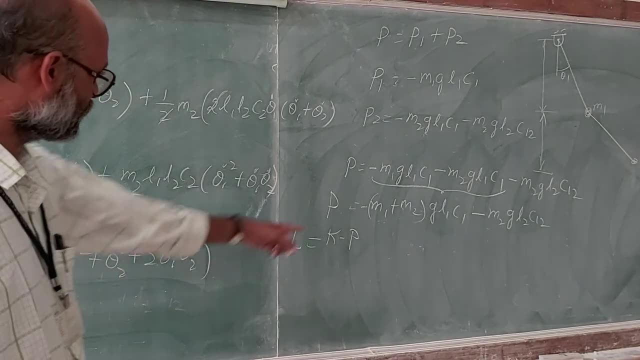 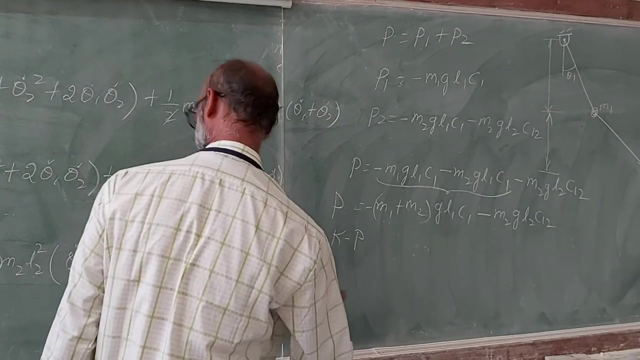 can write: what is the dendrogen for the problem? dendrogen for the problem is kinetic energy minus potential energy of the system. so this equation minus that equation, this is the dendrogen. now, if you infer this equation to what is the would be means that will explain. 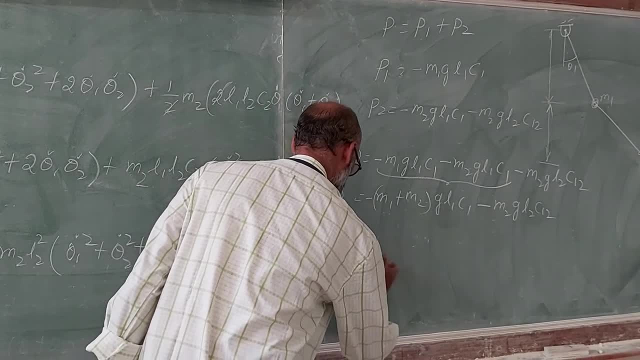 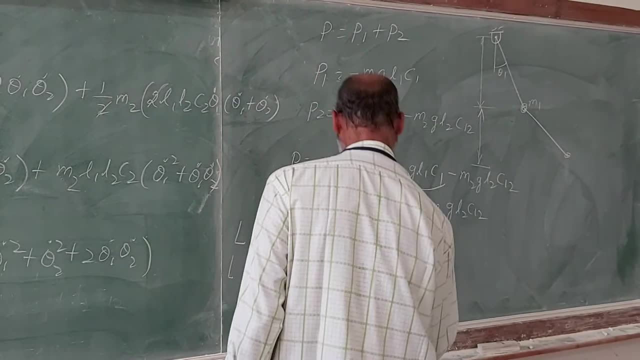 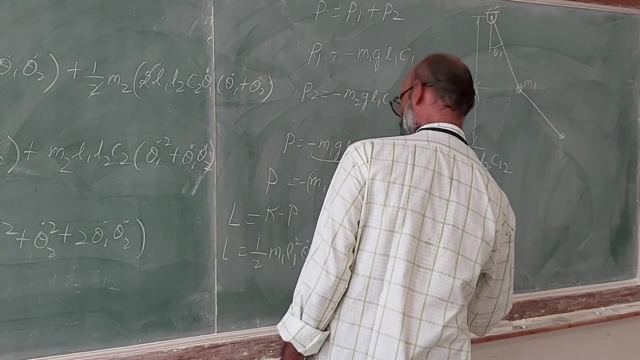 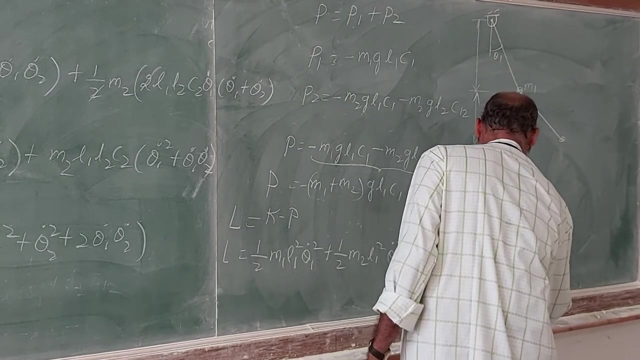 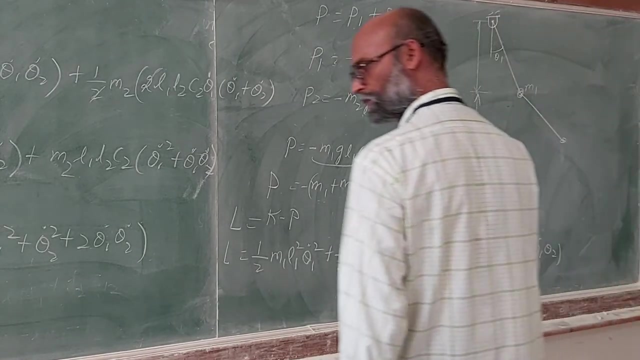 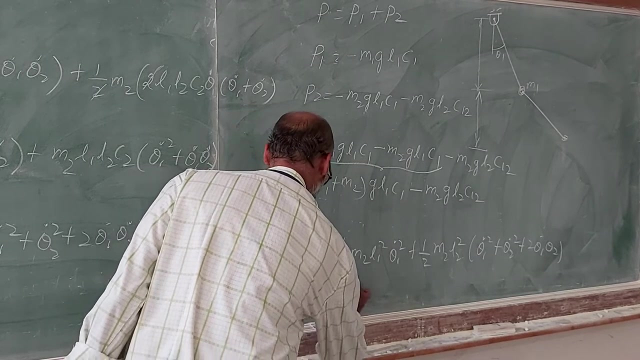 it, you will get theahr potential energy after encompasses dendrogen for the system or will be: Yes, square plus theta 2, dot. square plus 2- theta 1 naught, theta 2 naught. and we have plus m 2, l 1, l, 2, c 2- theta 1, naught. square plus theta 1, naught, theta 2, naught. this is kinetic energy. 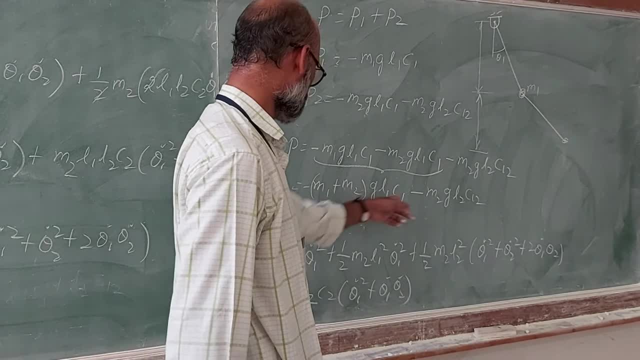 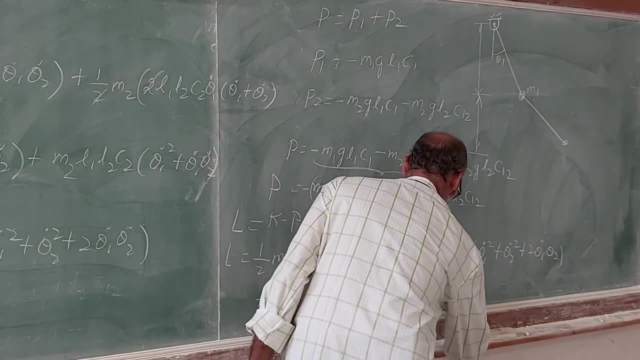 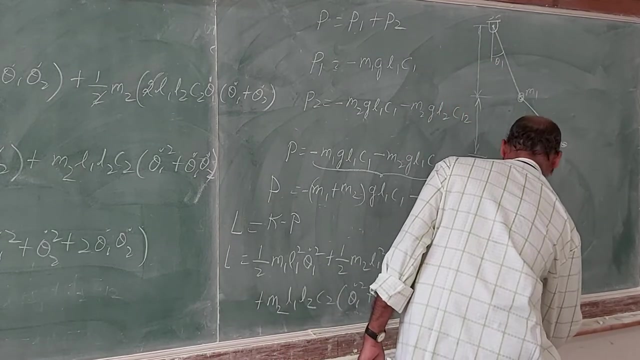 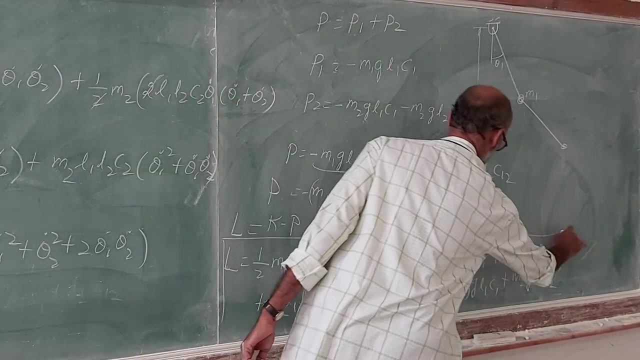 just, I have picked up this equation: minus of minus, everything becomes plus because it is minus potential energy. this is: this becomes plus. this also becomes plus plus l 1 plus l 2 g, l 1 c 1 plus l 2 g, l 2 c 1. this is your lagrangian. it is very, very important in evaluating. 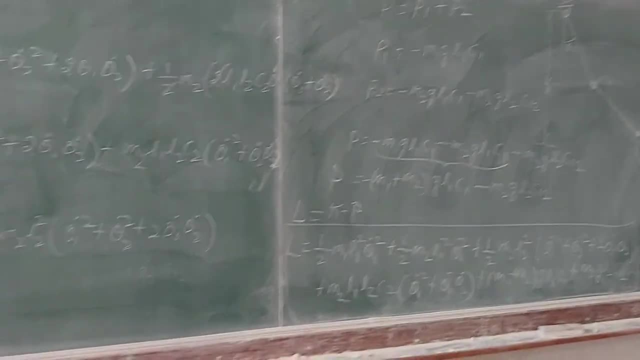 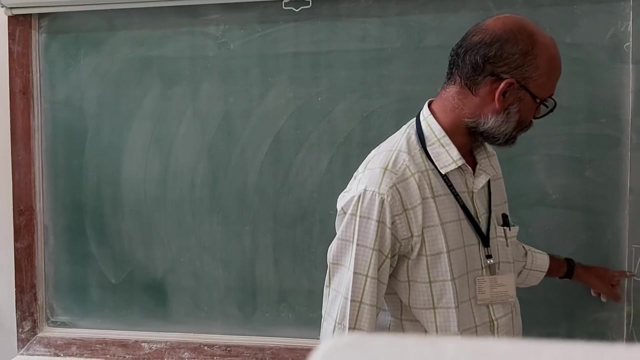 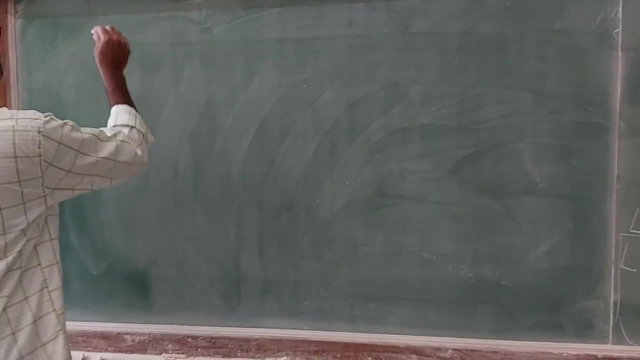 your extensions of motion. so we have to take equation forward: lagrangian. so this is the equation for lagrangian. so using this equation we will get equations of motion. so the lagrangian equation first. we will get del l by del theta 1 dot. please. 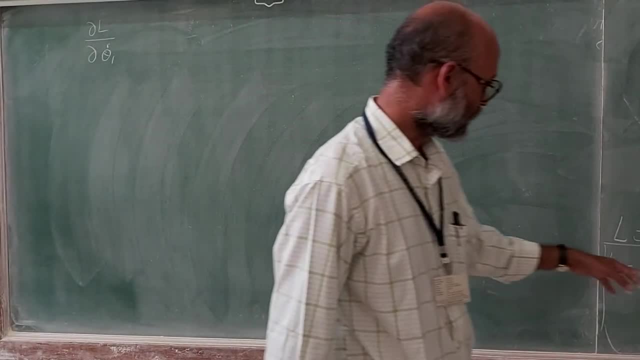 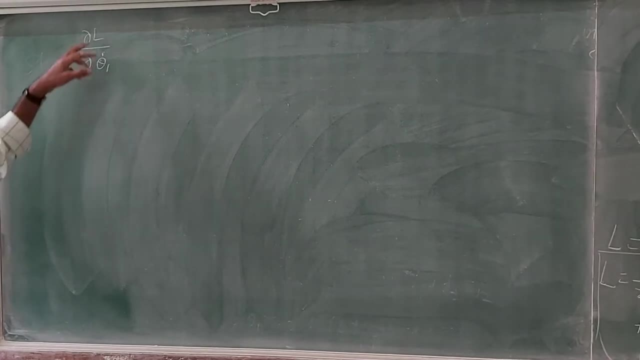 see the generalized coordinates of the coordinates of theta 1 and theta 2. so first we need to get equation, one equation for theta 1, another equation for theta 2. so let us write for first for theta 1. so first evaluate the lagrangian differentiate, this lagrangian with respect. 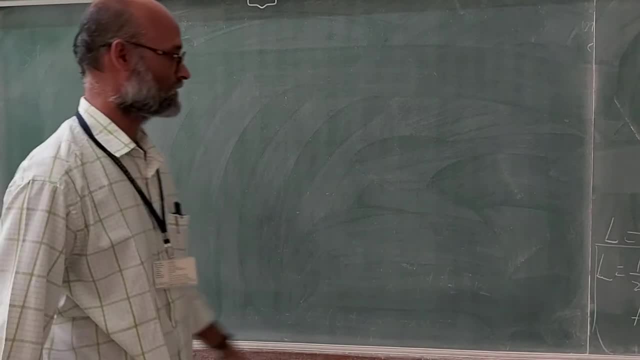 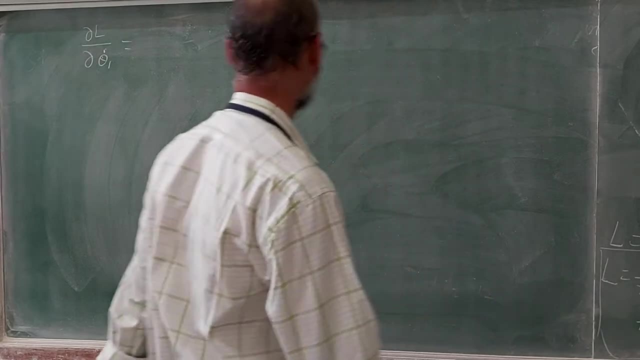 to theta 1 dot. when you do that, you can just take out: when you differentiate theta 1, naught square, this 2, theta 1, naught 2 will get cancelled. so this will be delimited. you have m 1, l 1 theta 1. 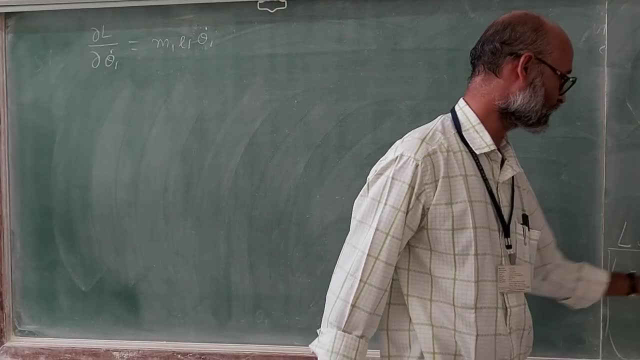 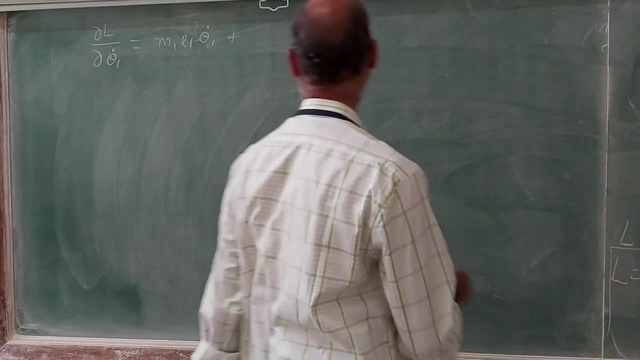 naught. that is the differentiation of this, this 2 and this 2 will vanish. so theta 1 naught the means. similarly to the second term, this half will vanish because of this. again, you have m 2, l 1 square. this is square, ok, so this is theta 1 and this is theta 2, so this: is theta 1 and if you look at here again, you have this m 2 l 2 square theta 1 dot plus m 2 l 2 square theta 1 dot. that is the differentiation of first term. there is no differentiation for this. this 2 and this 2 will get cancelled. you have m 2 l 2 square theta 2 dot. this is dot. you have plus m 2 l 2 square theta 2 dot. because differentiation of this, this 2 and this 2 will get cancelled. you have m 2 l 2 square theta 2 dot. this is dot. you have plus m 2 l. 2 square theta 2 dot. because differentiation of this, this 2 and this 2 will get cancelled. you have m 2 l 2 square theta 2 dot. this is dot. you have plus m 2 l 2 square theta 2 dot. 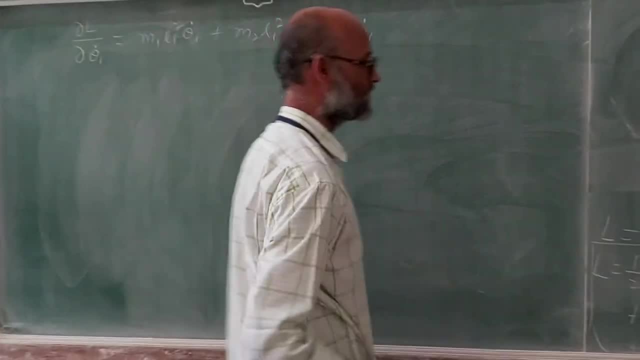 because differentiation of this, this 2 and this 2 will get cancelled. you have m 2 l 2 square theta 2 dot. this is dot. you have plus m 2 l 2 square theta 2 dot. because differentiation of this theta 1 dot. That is the differentiation of first term. There is one differentiation for. 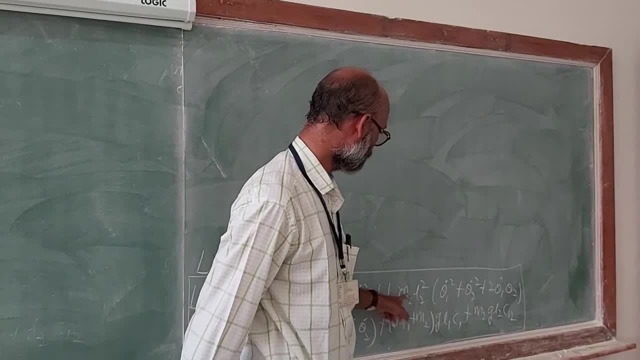 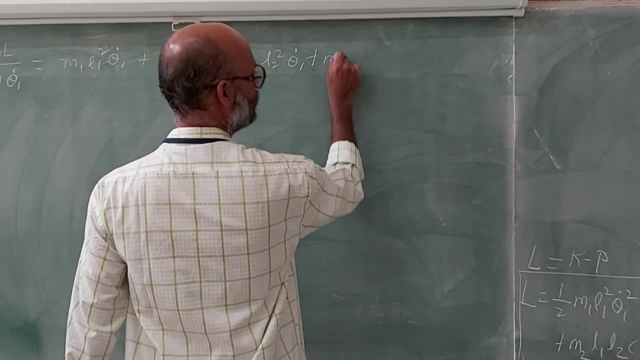 this, This 2 and this 2 will get cancelled. You have m 2 l 2 square theta 2 dot. This is dot. You have plus m 2 l 2 square theta 2 dot Because differentiation of this: this: 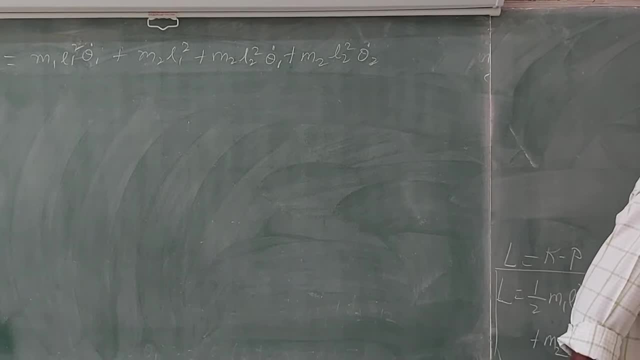 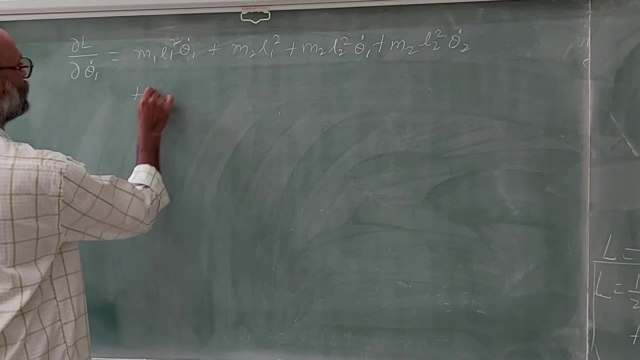 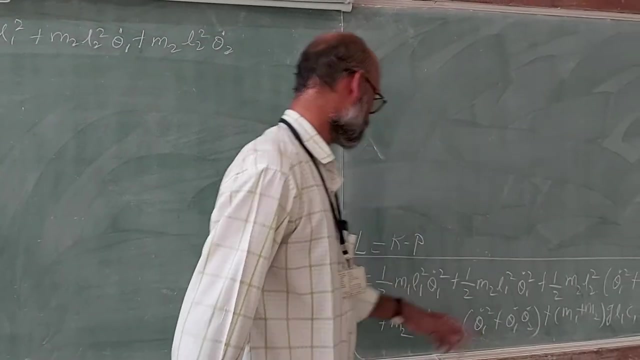 2 and this 2 will vanish. Differentiation of theta 1 dot is 1.. So we get that equation for the first term And then, if you look at this second term, the second line plus, you have m 2, l 1, l 2, c, 2.. Of course, differentiation of theta 1 dot square is 2 theta 1 dot. So. 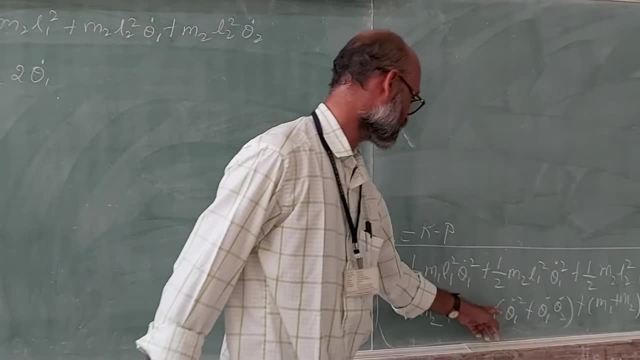 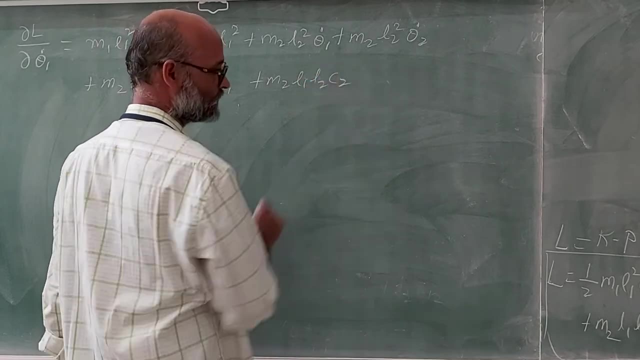 that is 2 theta 1 dot. That is the differentiation for the first term. If you take the second term, you have simply plus m 2, l 1, l 2, c, 2 theta 2 dot. That is the differentiation for. 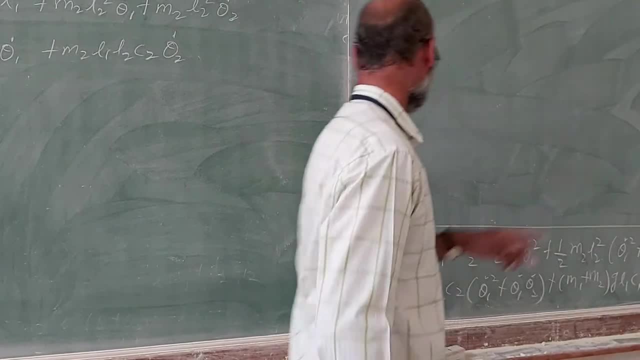 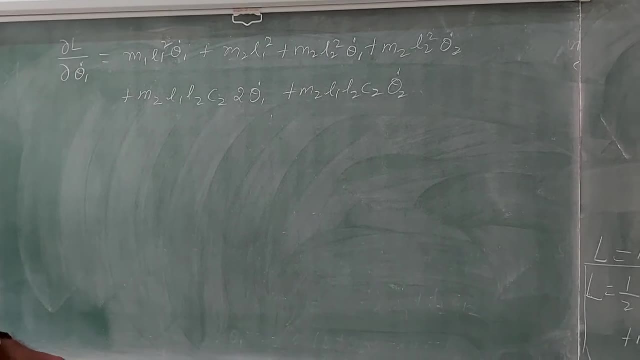 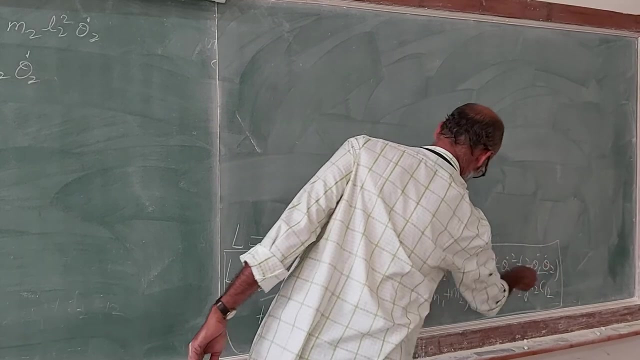 this term here. So we have this equation as delta by del theta 1 dot. So hope you understood Differentiation of this term, this term, this term, this and this 2.. That will lead to this equation Now. 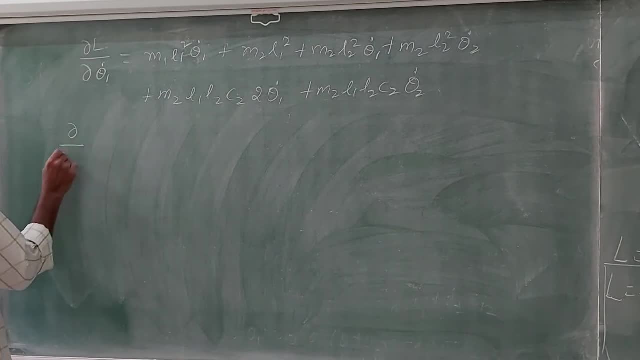 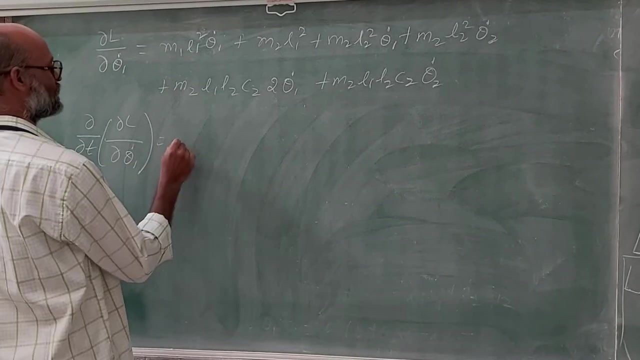 this is respect to theta 1.. We need del by del t of del, l by del theta 1 dot. The next step is evaluation of this. This equation we need to differentiate with respect to t, So that is the major concept here. So if we differentiate this, this is m 1, l, 1 square. 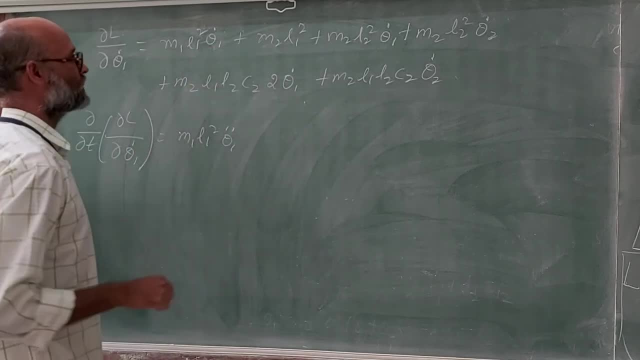 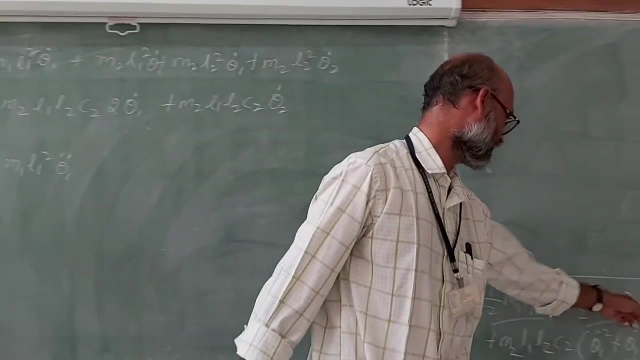 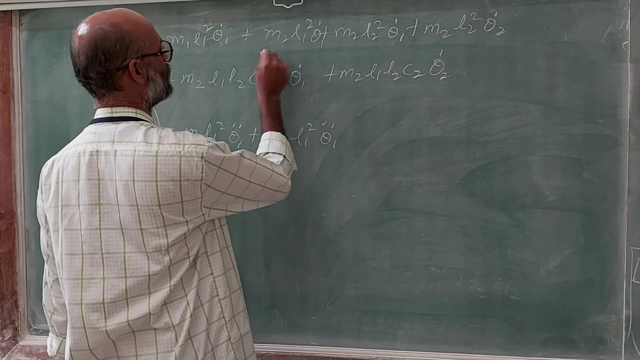 theta 1 double dot. Theta 1 dot becomes theta 1 double dot here. So this is- I think I missed out that one Theta 1 dot we get here. That is the differentiation for this second term. So we have plus m, 2, l, 1 square, theta 1 double dot. That is the differentiation. 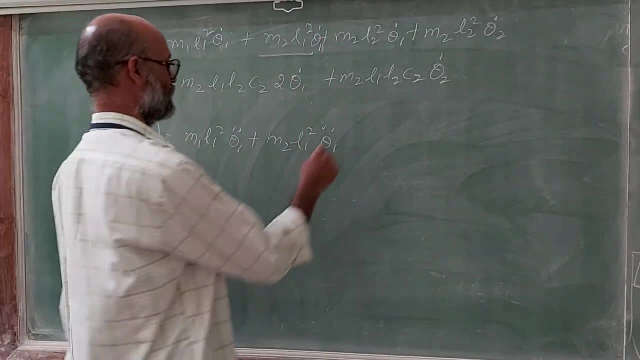 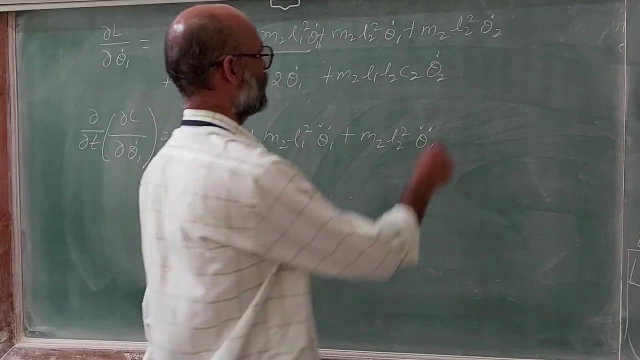 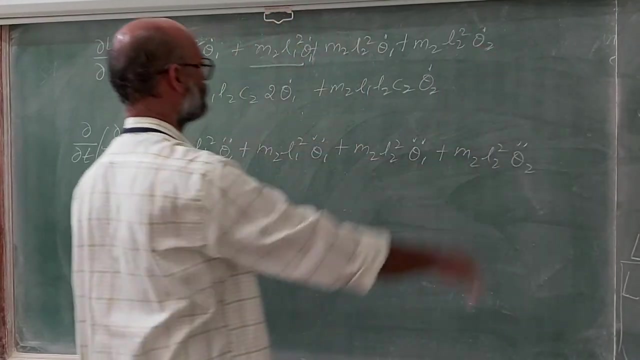 here. So we have this equation for this second term, and plus m 2 l 2 square theta 1 double dot, That is the differentiation of this third term. Again, m 2- l 2 square theta 2 double dot, That is the differentiation of the third term, Plus m 2 l 1- l 2.. These two I will write. 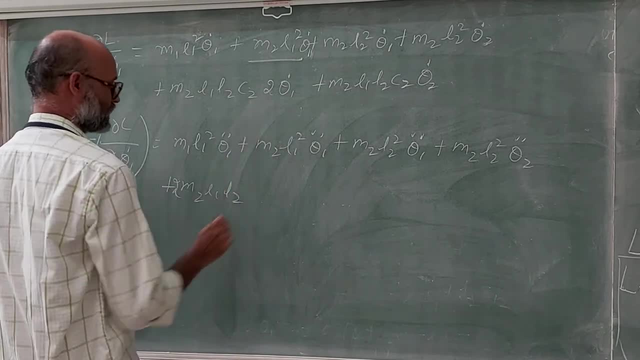 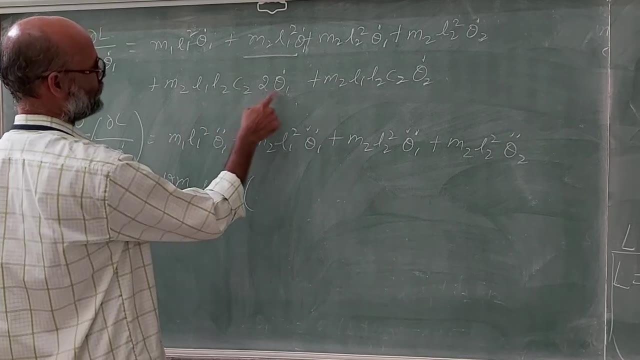 in the beginning. So these two we have product of two functions, That is, c 2 into theta 1 dot, m 2, l 1, l 2 and c 2 into theta 1 dot. It is a product of two functions We need. 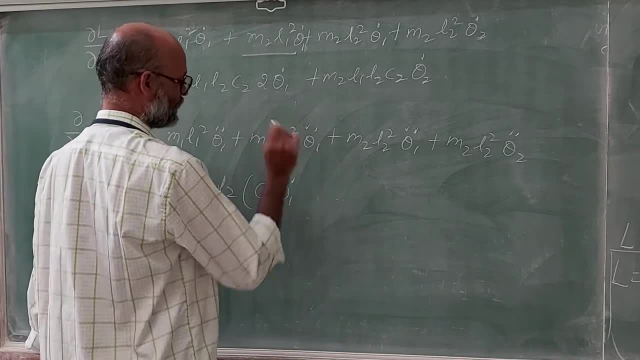 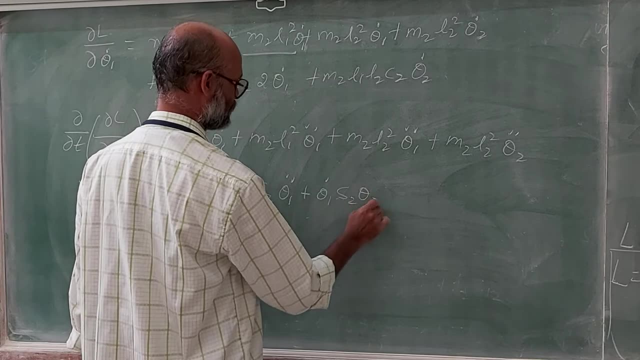 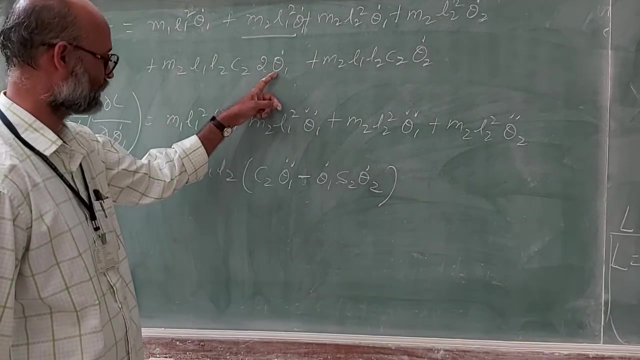 to differentiate this c 2. if you take this way, theta 1 double dot, Then plus you have that. if you take theta 1 dot like that, you get s 2 and theta 2 dot with a minus sign that I will put it over here. So that is the differentiation of c 2 into theta 1 dot. 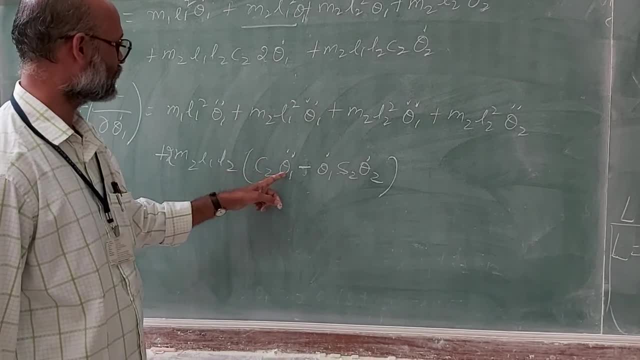 I kept c 2 as it is. Differentiation of theta 1 is theta 1 double dot and I kept c 2 as it is. I kept theta 1 dot. Differentiation of c 2 is s 2 into theta 2 with a negative sign. 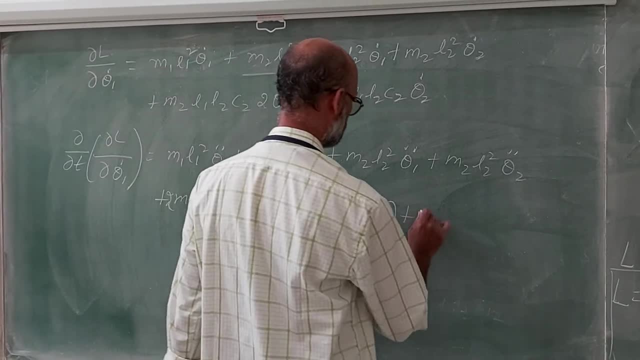 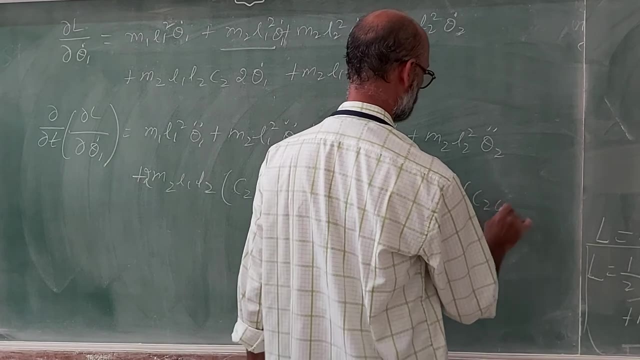 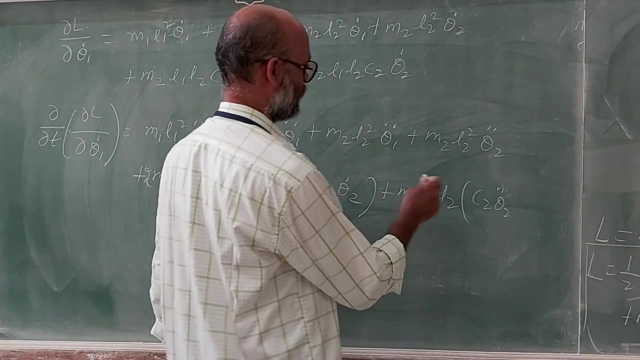 that minus sign, I have to put it here- Plus m 2, l 1, l 2.. Again we have differentiation of two terms. So c 2 I will keep, and theta 2 double dot. Differentiation of theta dot is theta 2 double dot And similarly, like previous thing, you have plus theta 2 dot. 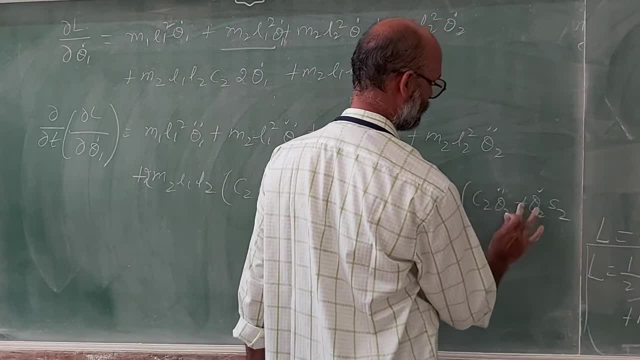 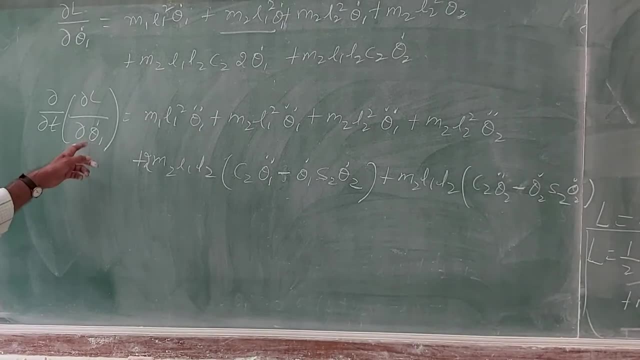 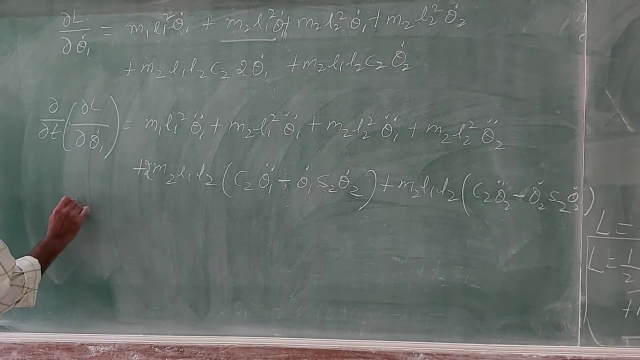 and differentiation of c 2 is minus s 2.. That minus, I will put it over here. And theta 2, differentiation of theta 2 is theta 2 dot. That is the differentiation for this equation. with respect to that, Just seen many things in simple simplification. 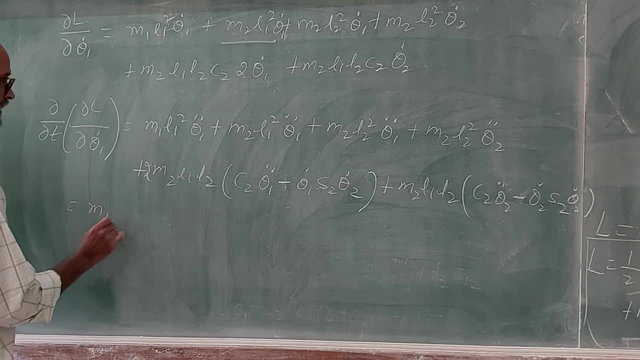 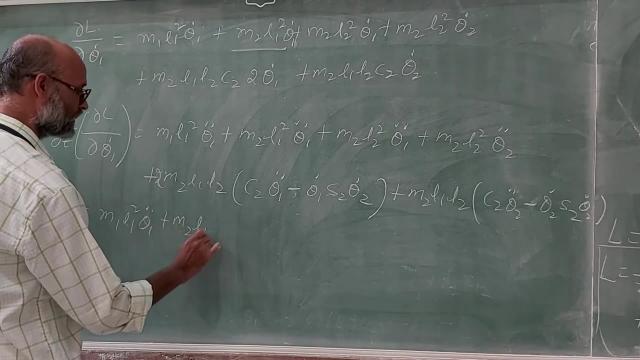 We will just do that. So we have m 1 l 1 square theta 1 double dot Plus m 2 l 1 square theta 1 double dot Plus m 2 l 2 square theta 1 delta 1 double dot Plus m 2 l 2 square theta. 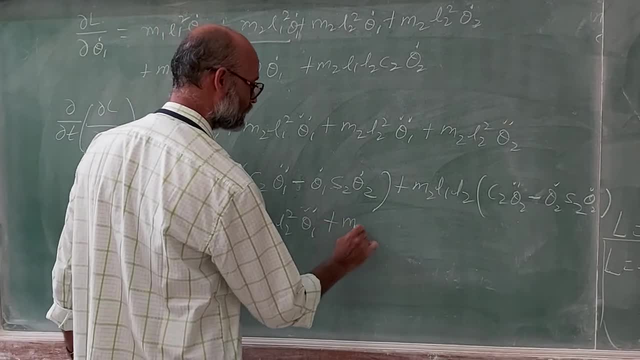 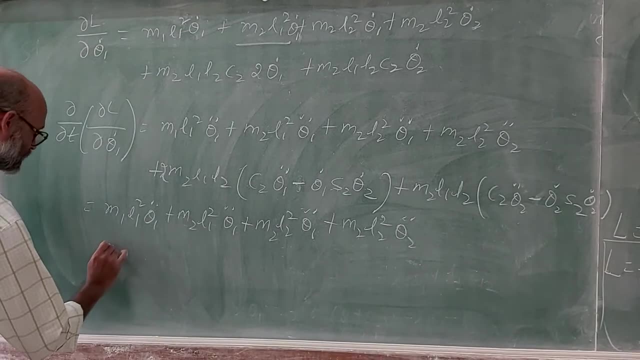 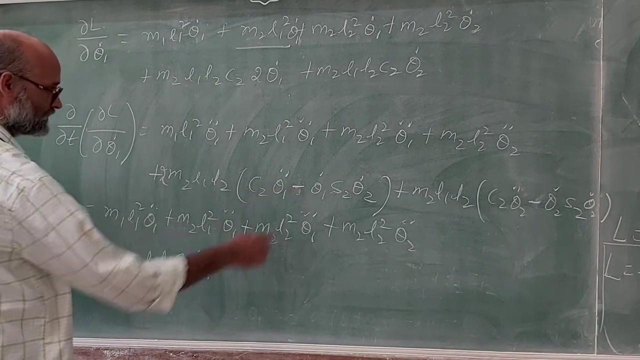 square- theta 1- double dot. plus m 2 l 2- square- theta 2- double dot. You can just expand this. we will get. what is that? plus 2 m 2 l 1, l 2 c 2- theta 1- double dot. I am expanding this. 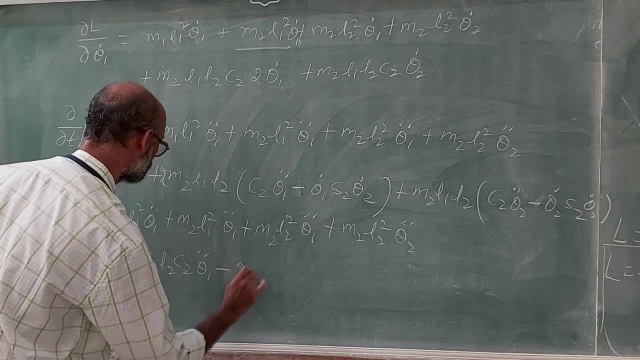 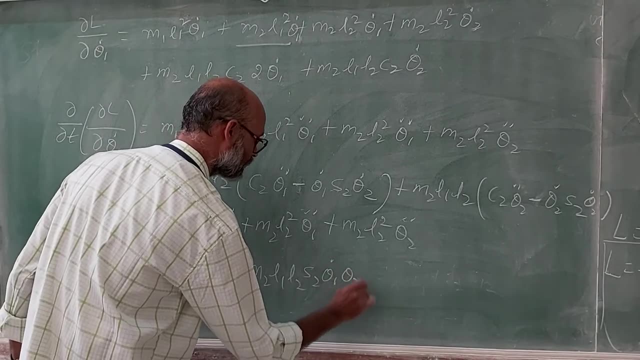 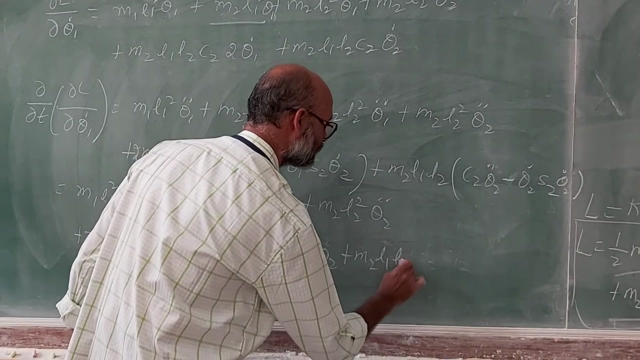 with a minus sign, you take this for minus 2 m 2, l 1, l 2. you have s 2 theta 1 dot, theta 2 dot. that is expansion for this and another 2 comes from this, plus m 2, l 1, l 2, c 2 theta. 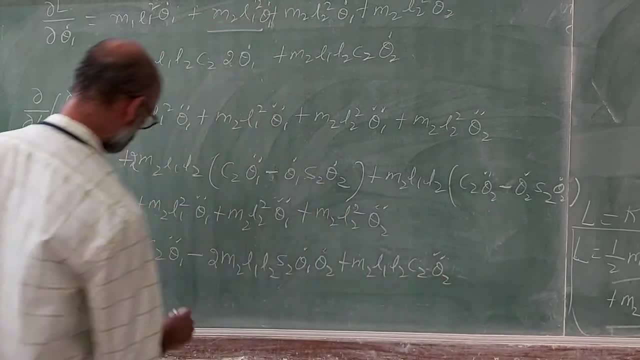 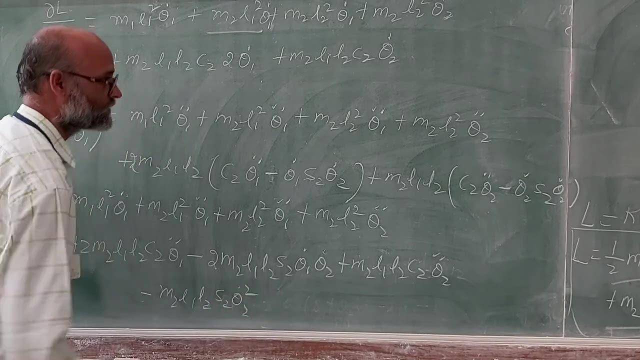 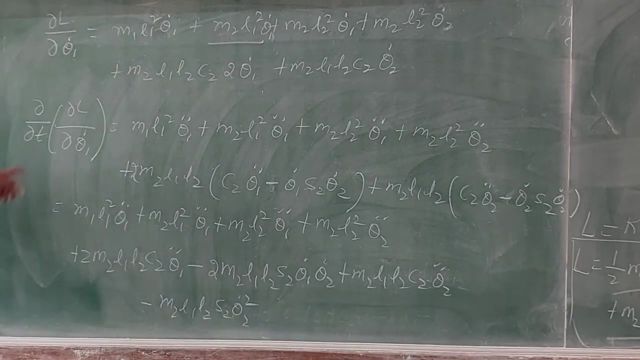 2 double dot. that is expansion for this and remaining thing minus, we have that m 2 l 1, l 2, s 2 theta 2 dot square. because theta 2 dot into theta 2 dot, we will get this theta 2 dot square. So this is your del l by del t respect to things we need to do. 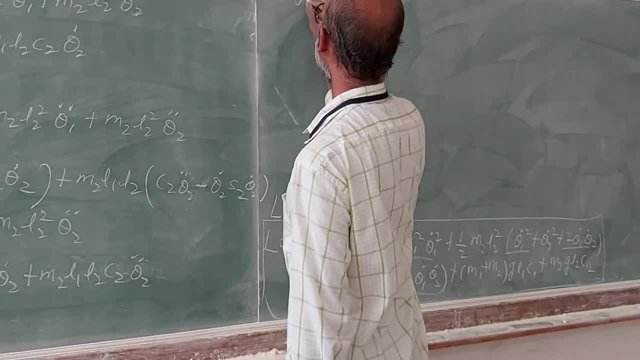 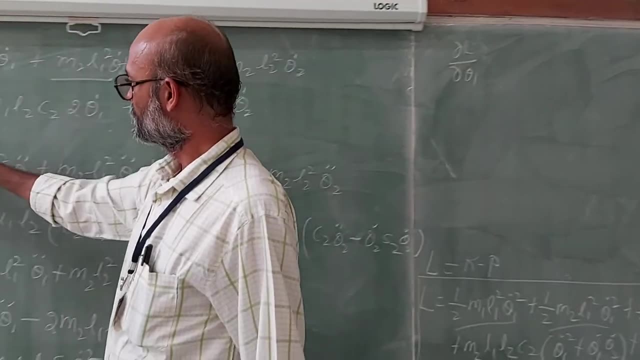 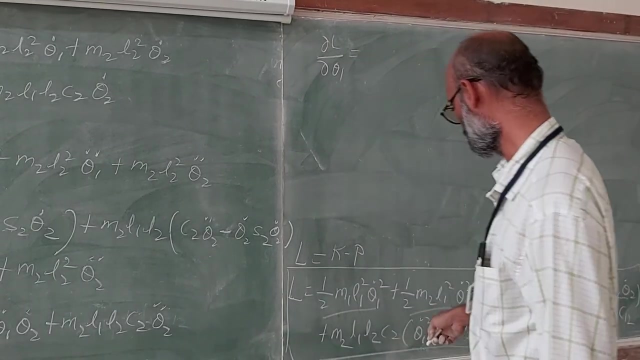 We need to do another one. we need to do another one: del l by del theta 1. this is the last term in your Lagrangian equation. first term is this and second term is this, what we obtained, and the third term is del l by del theta 1, only theta 1.. So let us differentiate this. 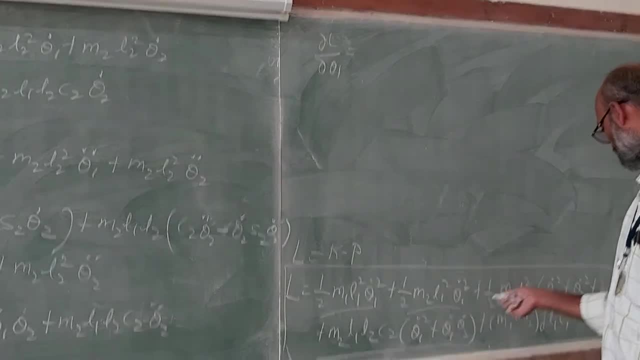 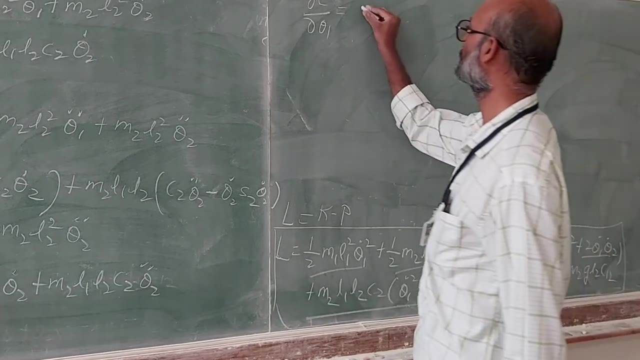 equation respect to theta 1. there is no theta 1 here, here, here, and you can see here, here also, there is no theta 1. theta 1 comes only in these two terms. we differentiate this respect to theta 1. we have m 1.. 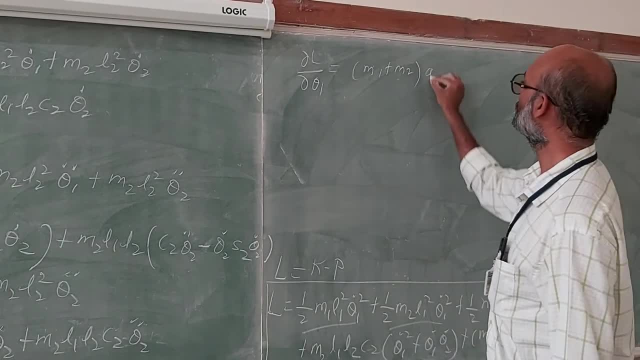 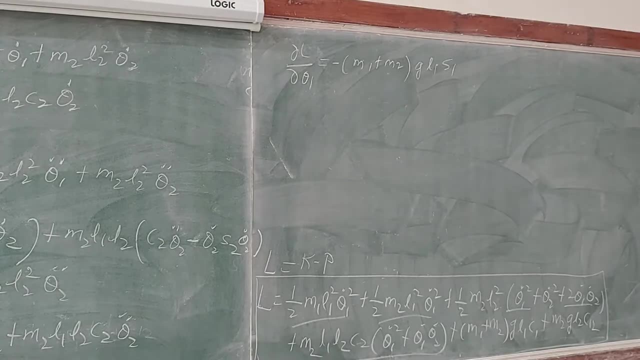 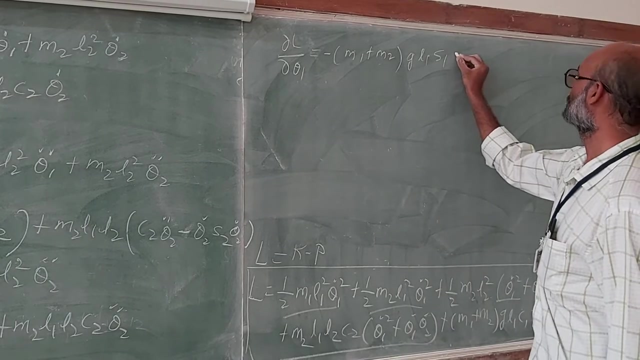 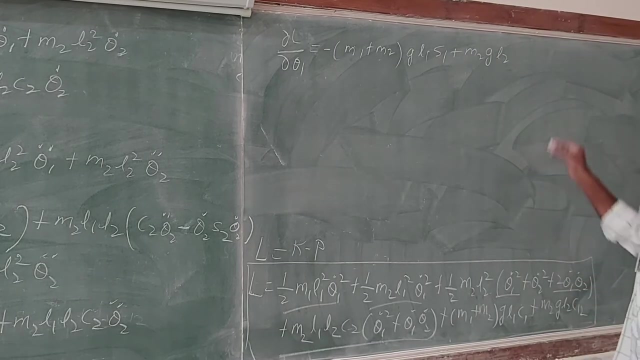 So we have m 1 plus m 2 here, whatever you have, your g l 1, that means differentiation of c 1 is s 1 minus with the minus sign, because differentiation of cos theta 1 is minus sin theta 1 and plus. here you have whatever that is plus m 2, g, l 2. differentiation of c 1- 2. 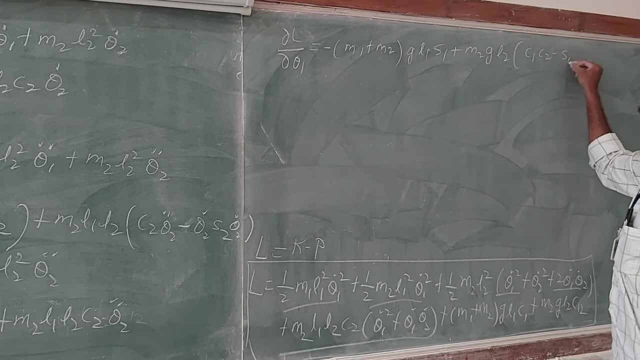 if you look at here: c 1 c 2 minus s 1 s 2, that is the expression of c 1 c 2 minus s 1 s 2.. So this is the expression for this. if you differentiate this, what are we going to get? 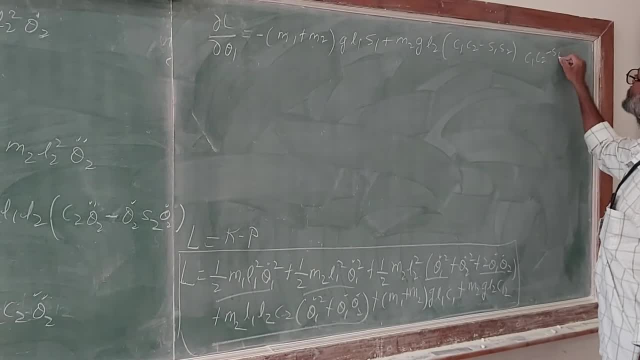 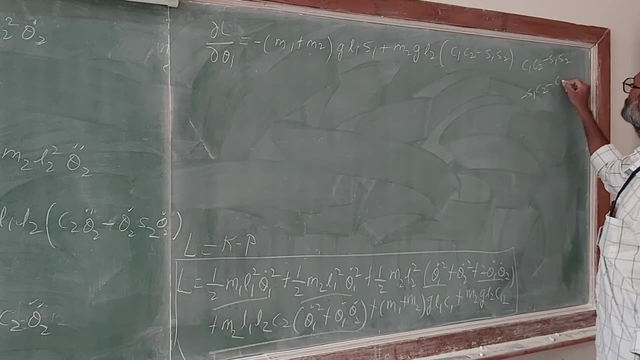 I just like separate this one c 1- c 2 minus s 1- s 2. if you differentiate this c 1, this is minus s 1- c 2. if you differentiate this, this will be c 1- s 2 if you take minus out. 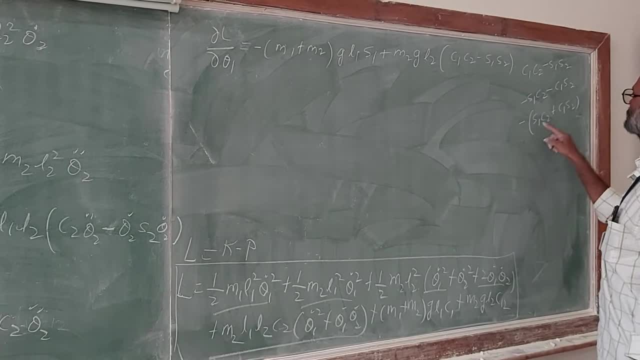 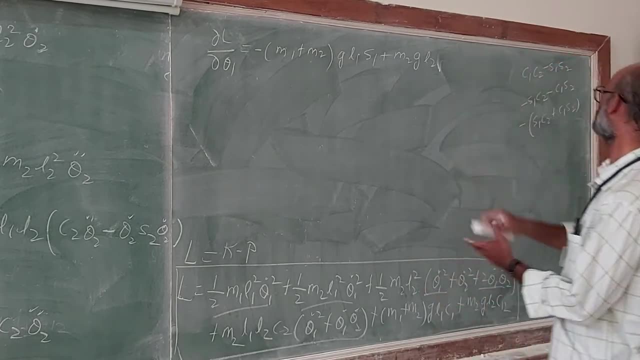 this will be s 1, c 2 plus c 1, s 2. this is nothing but s 1, 2. this one, c 1 2, with the minus sign this. I like this as if you look at this calculations what I have done, this: 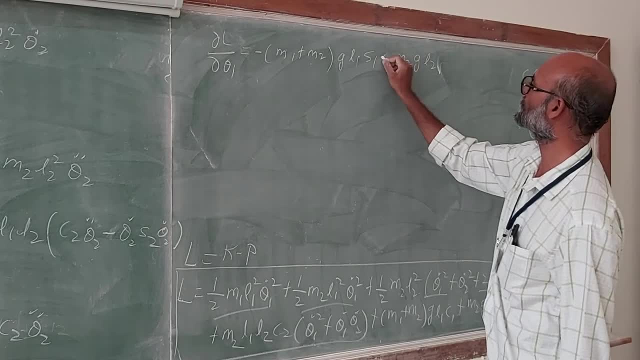 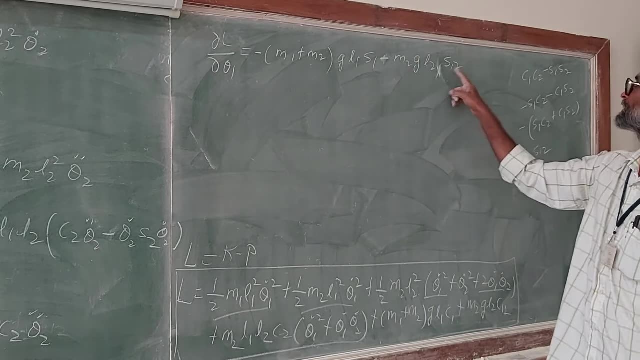 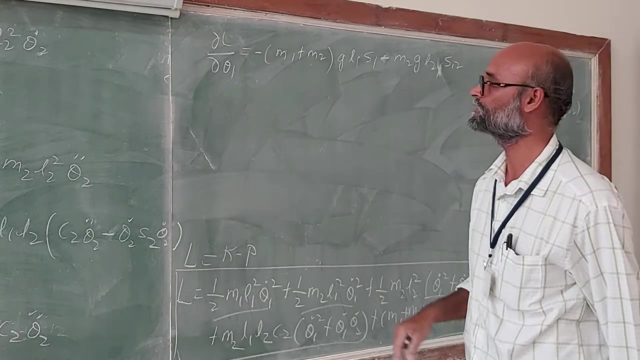 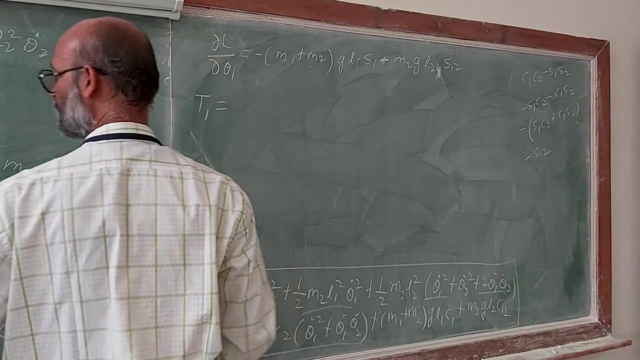 is minus of s 1. so this I take right. plus minus this is s 1. so differentiation of this term c 1, 2, will get you as minus s 1, 2. this is the small calculations for this. so this equation is: del l pi, del theta 1. now to obtain the first equation: t 1 is equal to what, please? 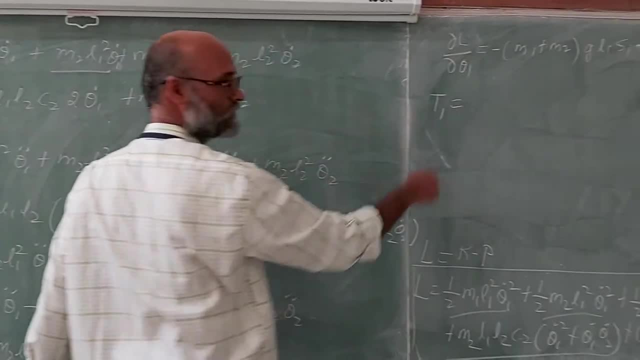 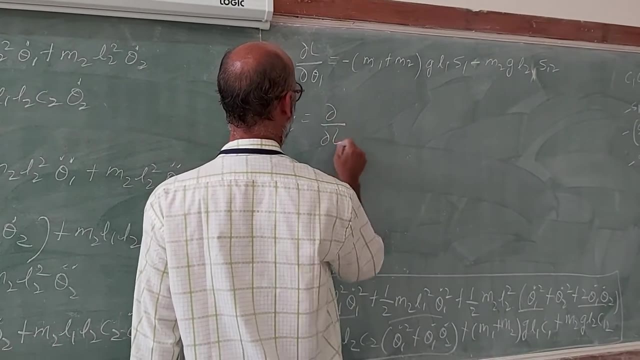 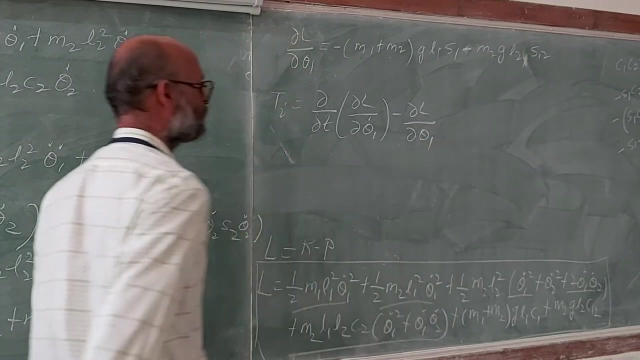 see this term minus. this term will give you the first equation for the del l pi del theta 1.. I will repeat for your case t i: this is del l pi del t of del l pi del theta 1 dot minus del l pi del theta 1, this is your Lagrange equation, so we obtain this term as well as. 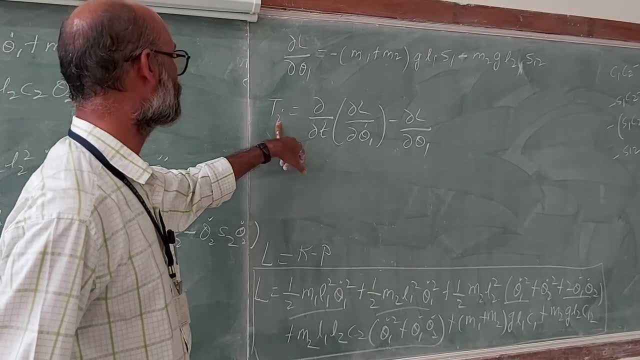 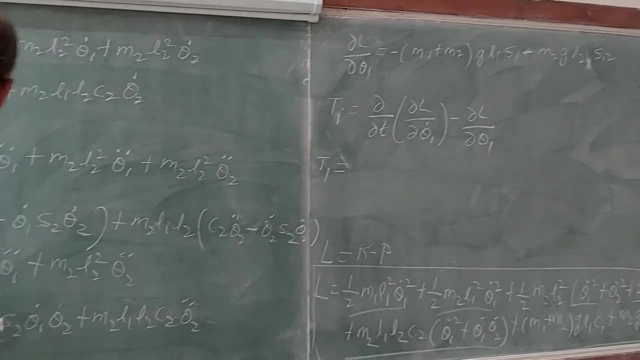 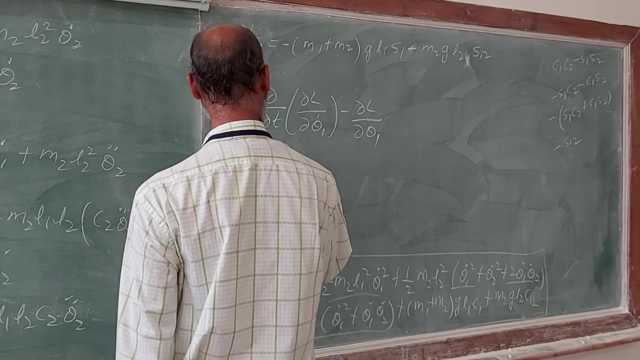 this term. we just combine this, now i becomes 1 because we are evaluating for the first mass. so this is t 1. so first equation t 1 is this 4 equation minus that equation. so what are we going to get? this is m 1 l 1 square, theta 1 dot square plus m 2 l 1 square. 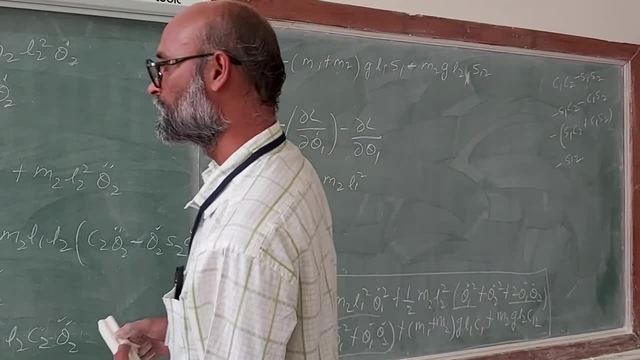 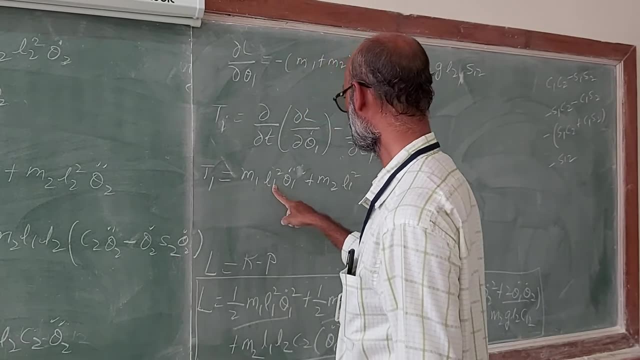 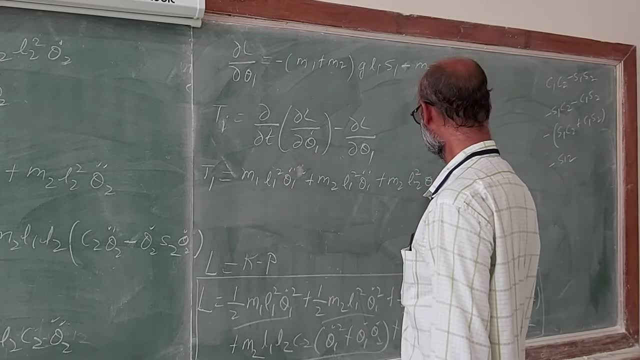 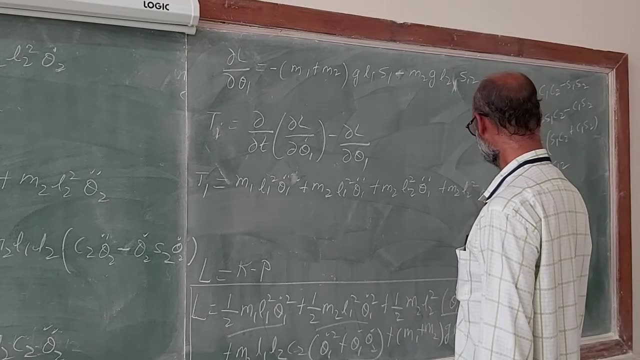 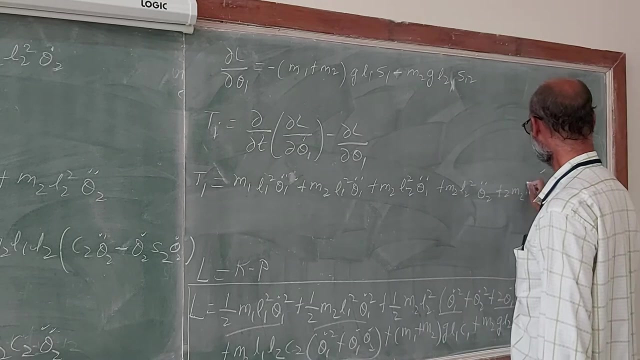 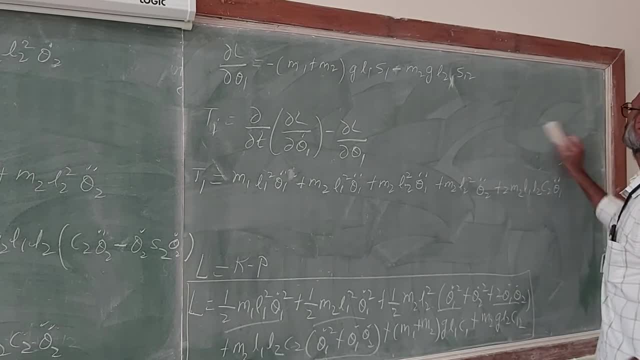 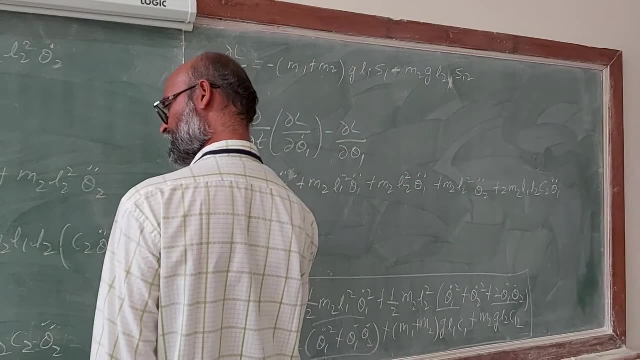 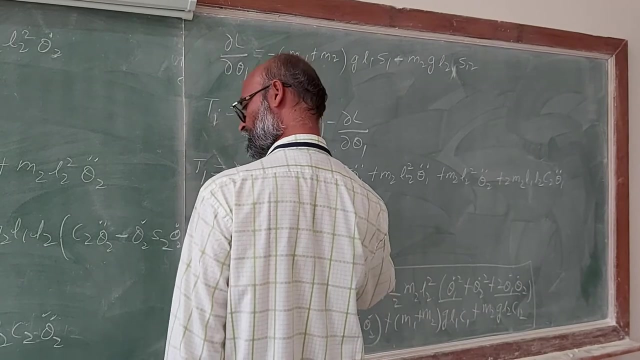 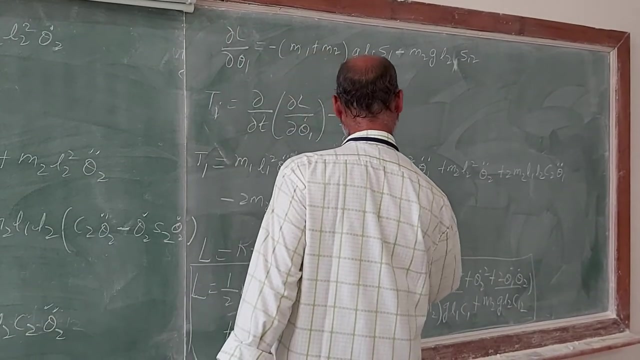 theta1 double dot. so that is 2 m2 l1 l2 c2- theta1 double dot, minus 2 m2 l1 l2 s2- theta1 dot- theta2 dot. so that is this term plus m2 l1 l2 c2- theta2 dot- theta2 double dot, so that 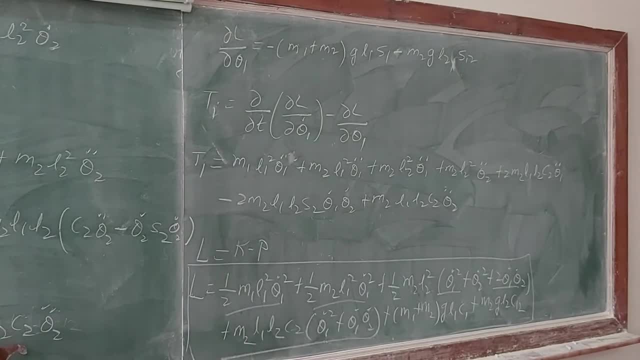 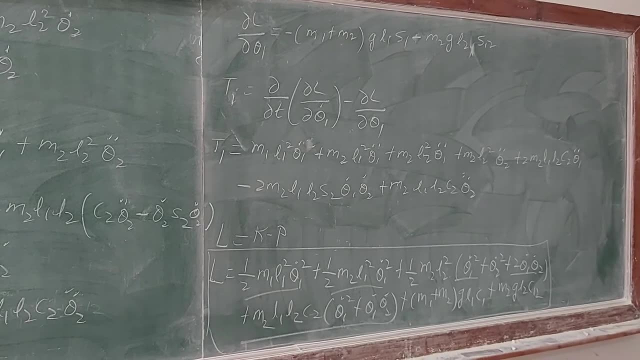 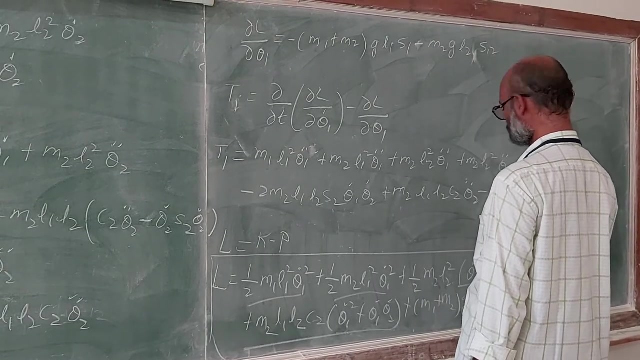 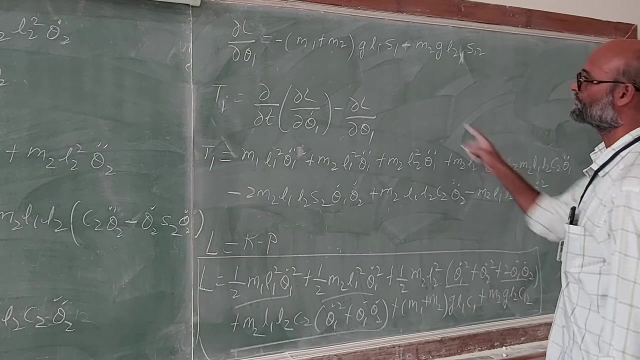 is this equation okay? and the final one: we have that minus m2, l1, l2, s2, theta2, dot square, this is this term: minus of minus these two becomes plus we have, and then this one plus. we have plus, and then this one plus, and then this one plus, and then this one plus, and then 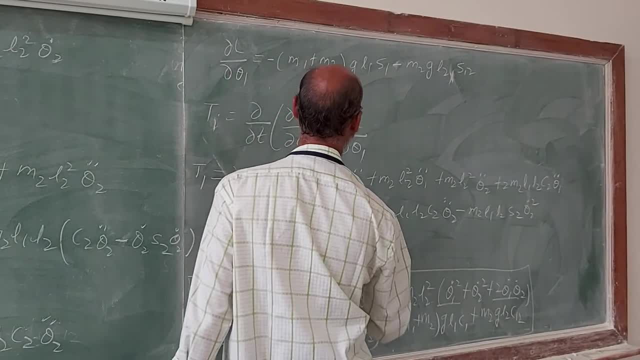 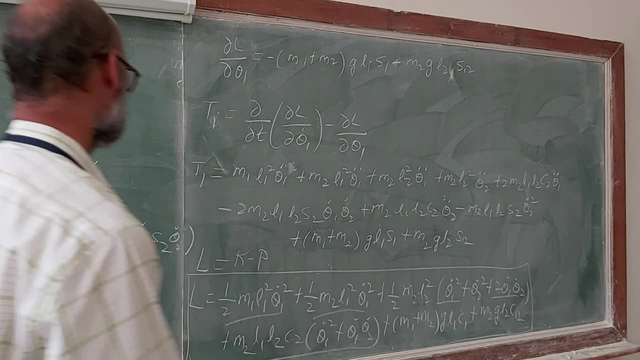 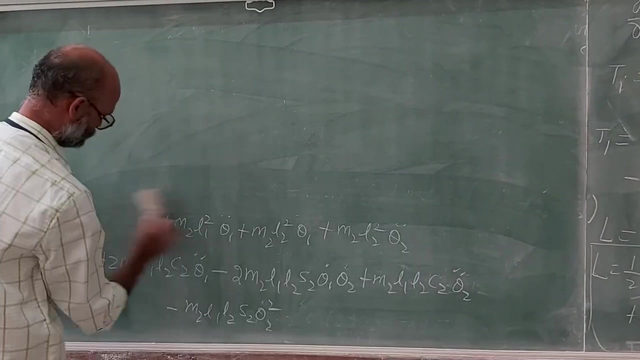 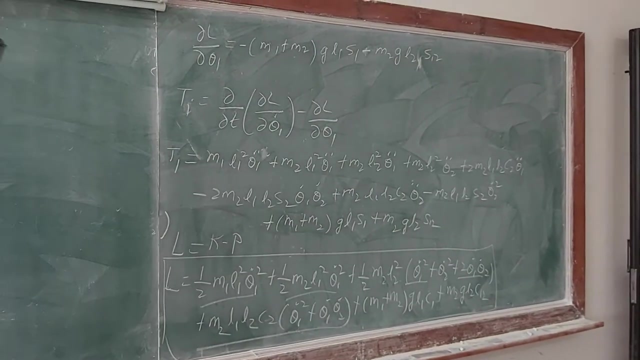 now this has m1 plus m2 g, l1, s1 plus m2 g, l2. this is the first equation. we will simplify that equation and then write it in a compact manner. so this is the first equation of motion. so we just simplify this. so, p1, we will try to pick up one double dot times theta1 double. 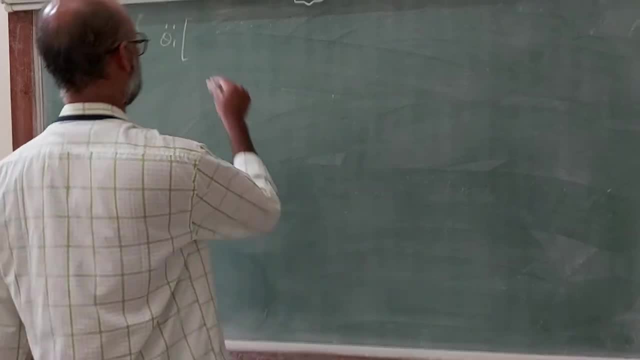 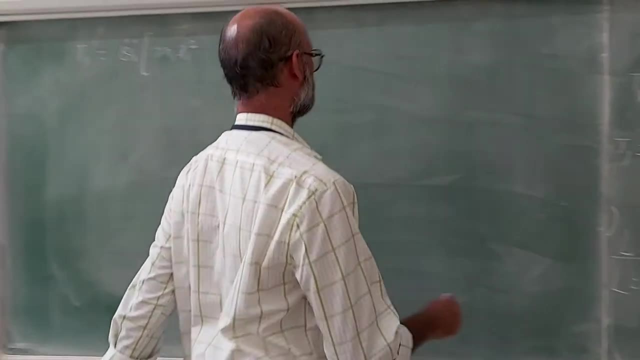 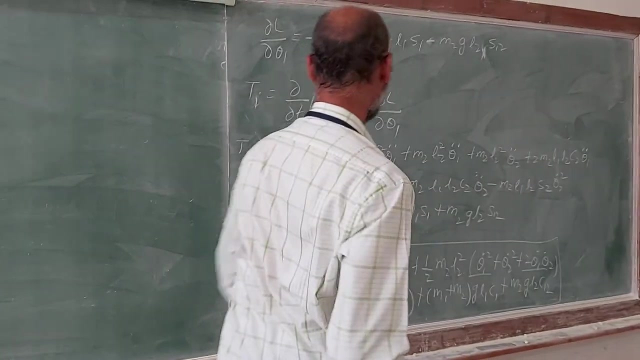 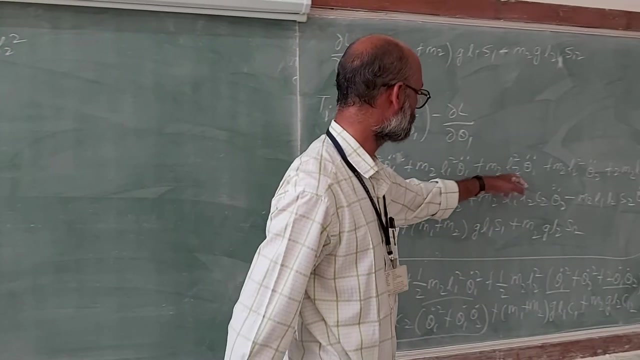 dot times: theta1 double dot times with group dot times. so we have that m1 l1 square, that is from the first term, and again we have plus m2 l1 square, plus m2 l1 square, that is from the second, third term. we have m2 l2 square, m2 l2 square. these are all theta1 double dot. 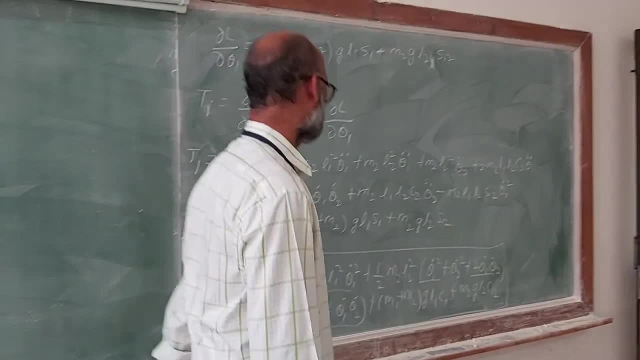 terms. so that is the third term. so we have again 2 m2 l1 l2 c2 plus theta1 double dot terms. so we have again 2 m2 l1 l2 c2 plus theta1 double dot terms. so we have again 2. 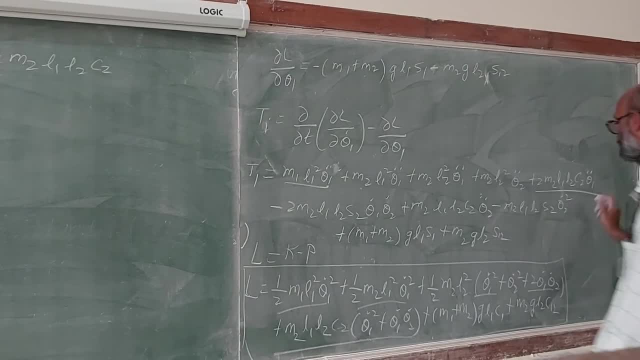 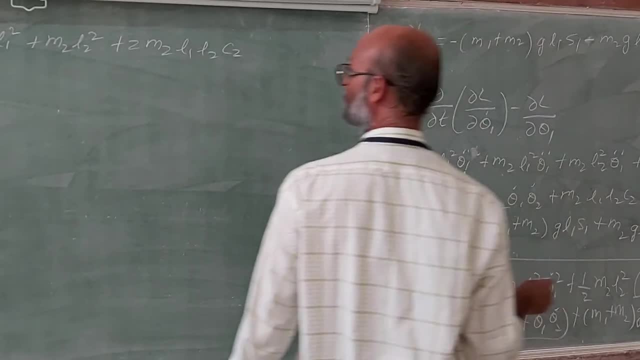 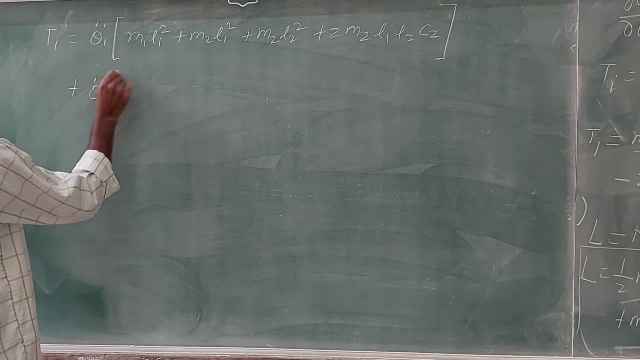 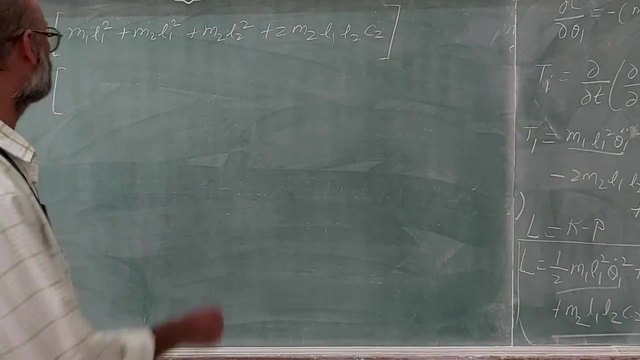 there is no theta 1 double dot here. also there is nothing. so those: this is your theta 1 double dot terms, plus write theta 2 double dot terms. so theta 2 double dot term. we have m 2 l 2 square, m 2 l square, the other one m 2 l 2 square. that is from this term theta 2 double. 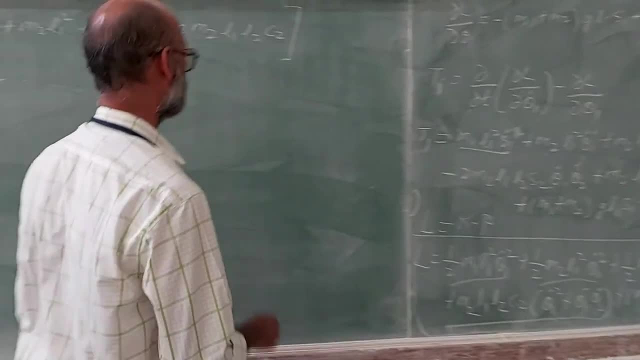 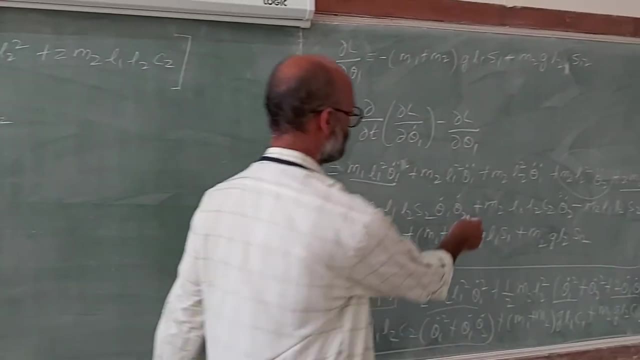 dot and we have another term: m 2, l 1, l 2, c 2, plus m 2 l 1, l 2, c 2. this is from this term, theta 2, double dot, and to resolve theta 2 double dot, that is, we have this term, so theta. 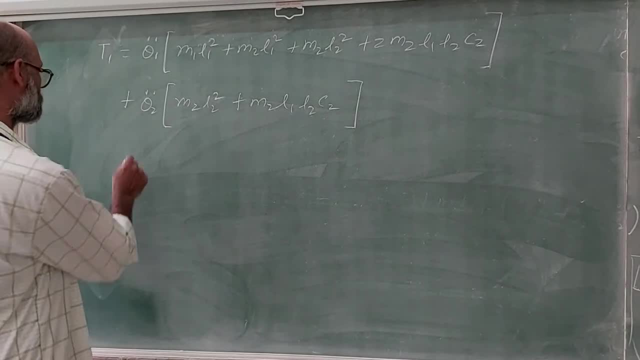 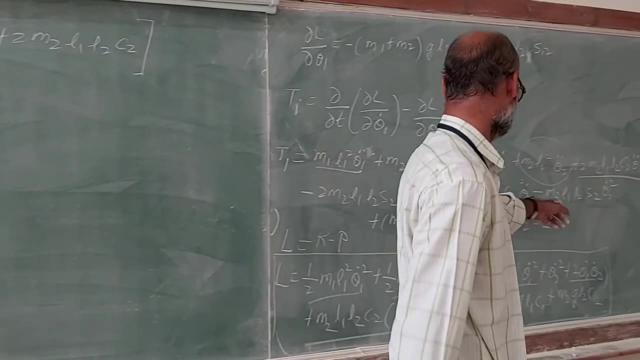 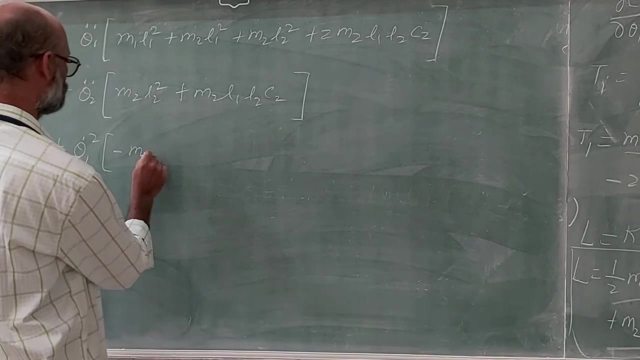 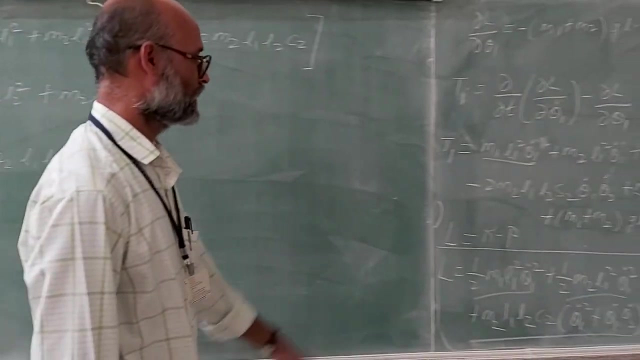 1 double dot. is there? theta 2 double dot plus, you have any theta 1 dot square term you can write here. so theta 1 dot square. we have this one, that is with the minus sign: theta 2 double dot. so you have minus m 2, l 1, l 2, s 2. so that is your theta 1 dot square term and you are. 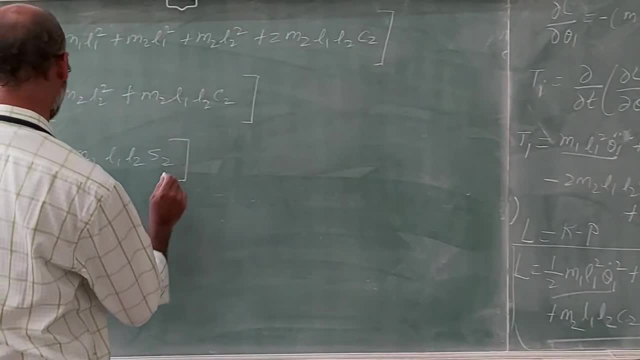 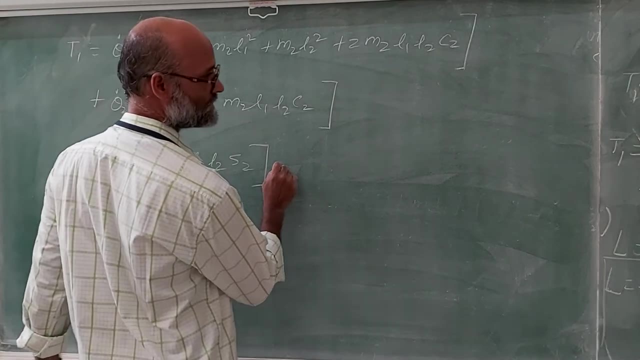 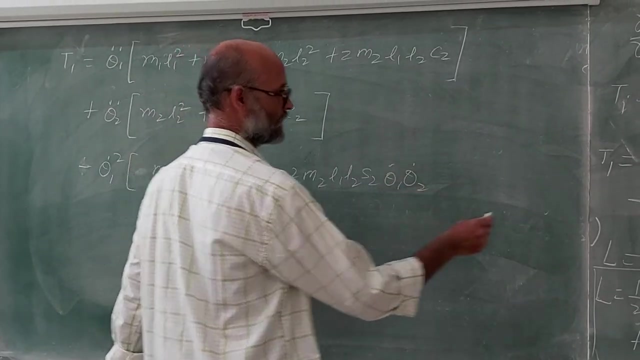 remaining with this term minus. I just write this as minus here so you do not get confused. same thing, I am writing minus. you have 2 m 2 l 1 l, 2 s, 2. theta 1 dot. theta 2 dot. that is theta 1 dot. theta 2 dot, that is your theta 1 dot square term. so this term is minus m. 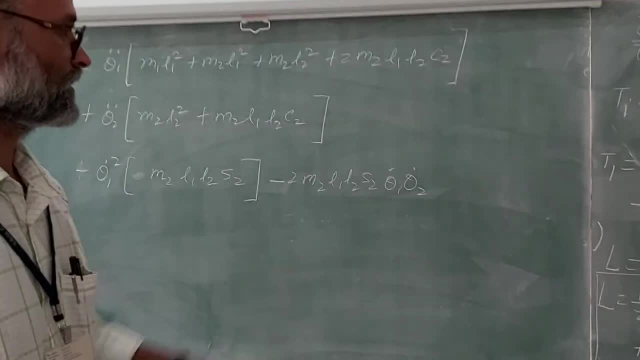 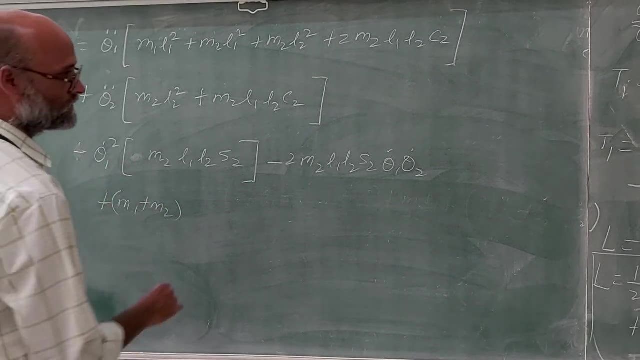 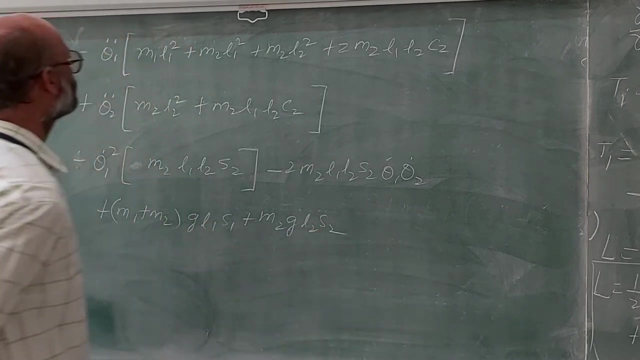 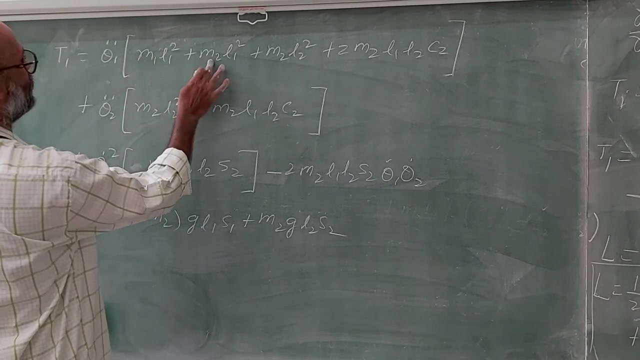 from this term, only that last potential terms are remaining, plus the two terms plus m1, plus m2 g, l1, s1, plus m2 g- l2, s2. this is the first equation of motion you have obtained. you can even combine this equation m1- m2 and then simplify further. but I will keep touching. 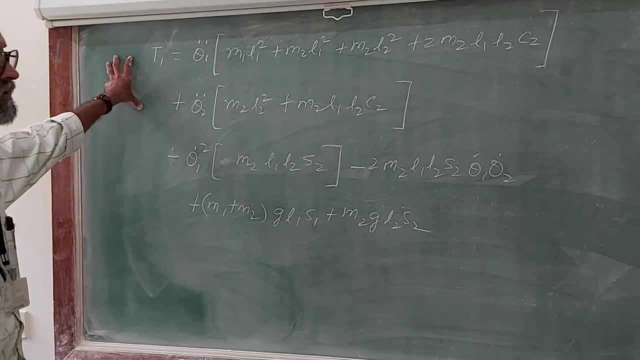 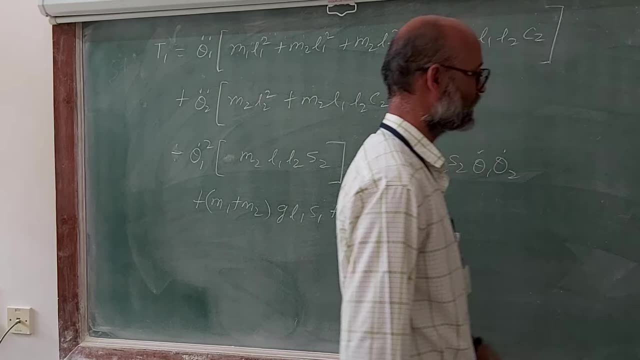 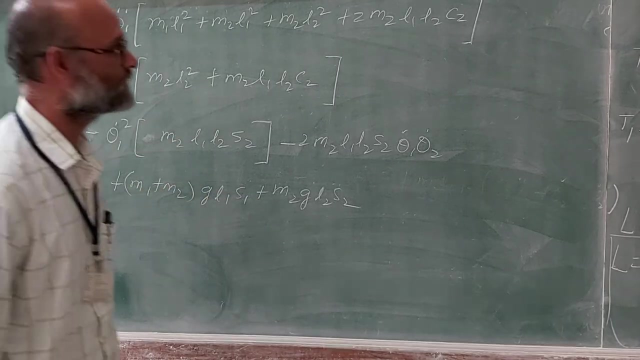 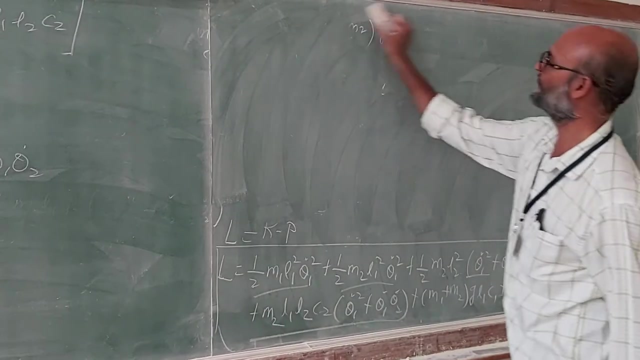 this. so this is the first equation of motion you have obtained. similarly, you need to proceed with the second mass using the same method. we will proceed ahead so we will derive the second equation. so to derive the second equation, we need to get the equation again for the 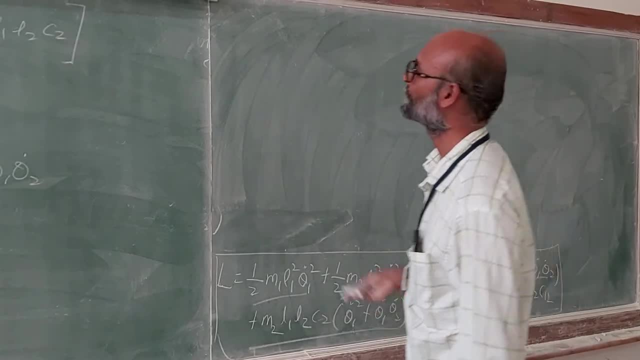 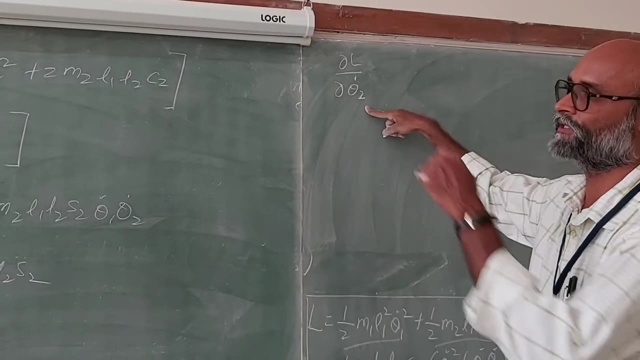 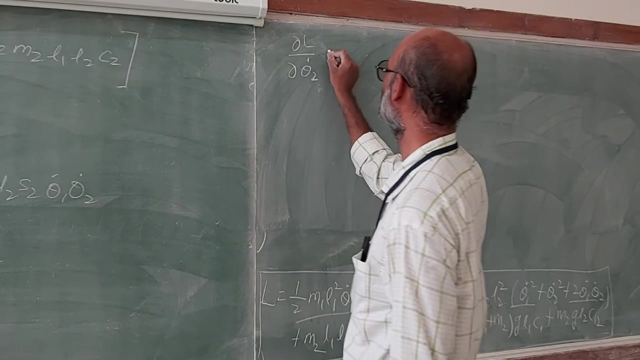 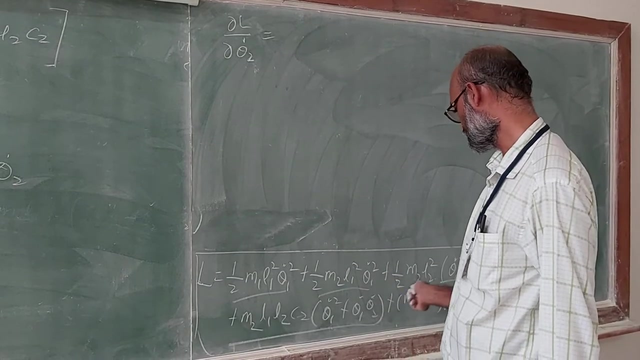 second mass. so we will do it here. so what is the first one? first equation of motion. now we need to take theta2 dot and what are the equations? we are going to use the same equation when you write theta2 dot. so we have this differentiation of this. there is no theta2, so we do not get any term differentiation of this theta2 term. 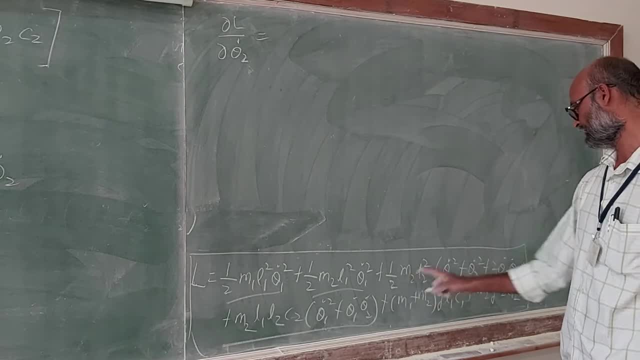 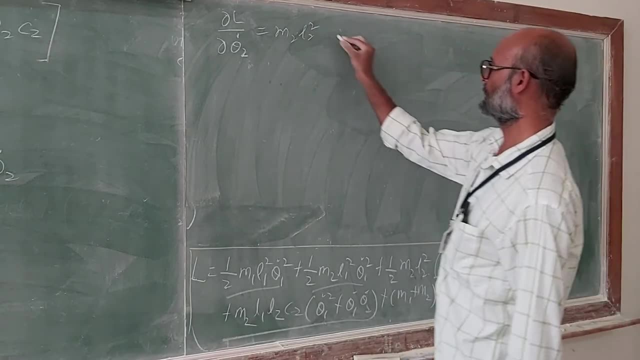 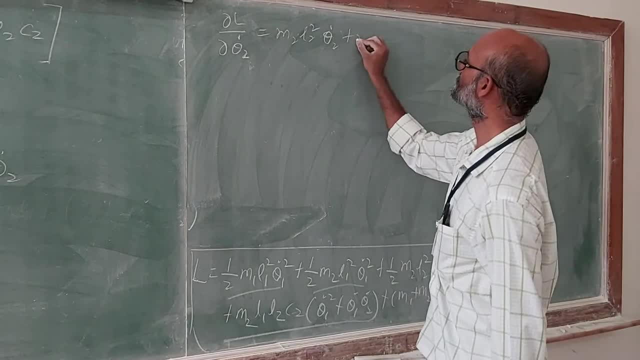 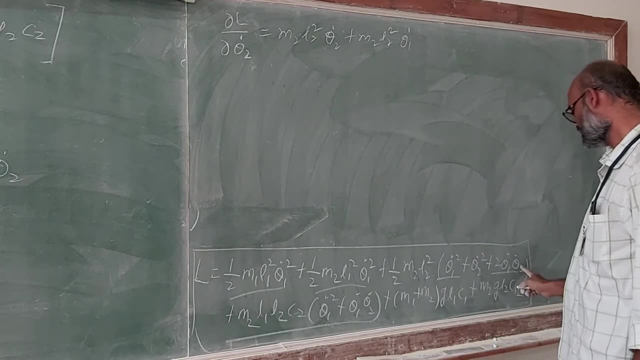 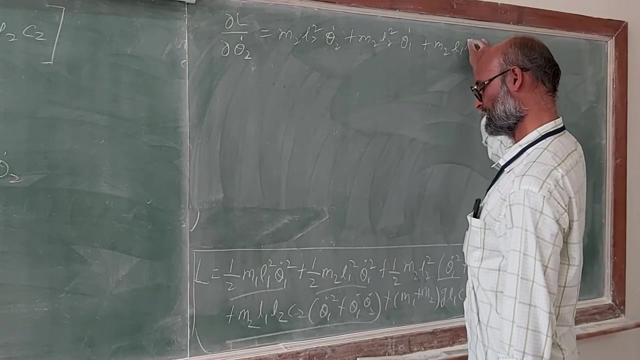 will vanish here. m2 a2 square. m2 l2 square- this is here and theta1 dot and this will get cancelled as theta1 dot, because differentiation of this is theta2 dot, then theta1 dot and simply go over here. plus you have m2l1 l2- c2- the definition. again. this is gonna be used. 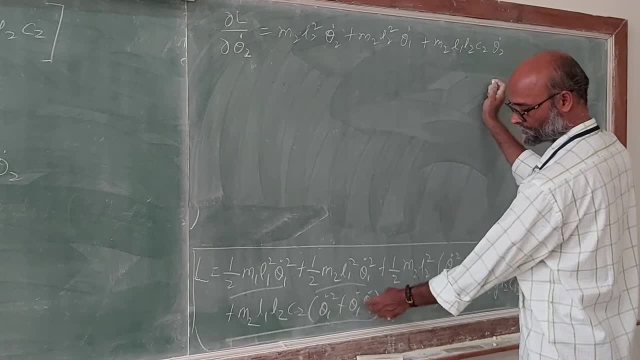 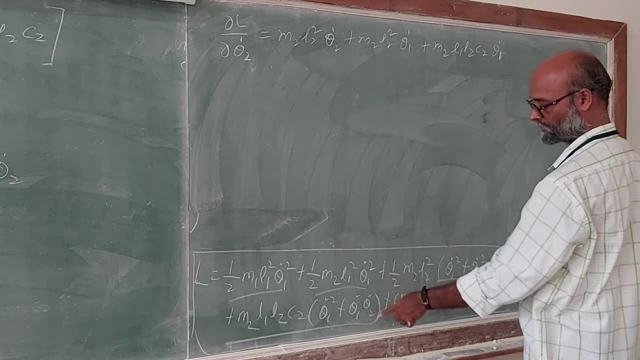 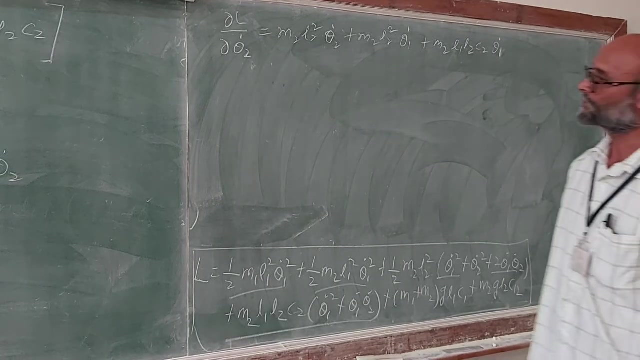 theta2 dot. differentiation of this term is theta 1 dot will remain as this dot. theta 2, because we differentiate with respect to theta 2, this will come 1, so we will get only theta 1 dot. so these three are the terms for theta 2 dot. so next thing is you need to figure out what. 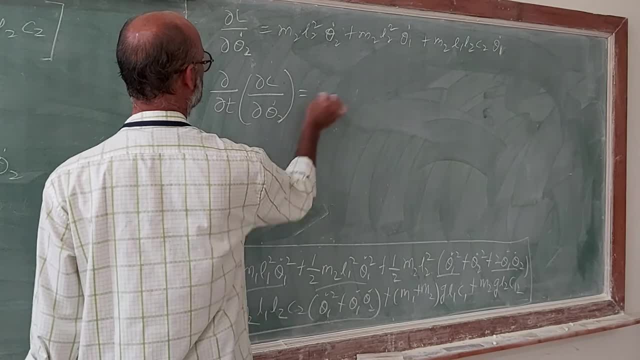 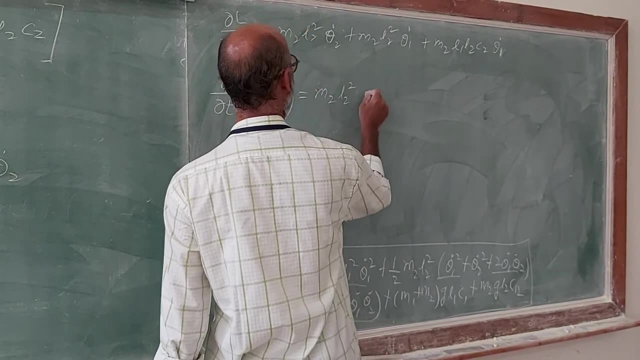 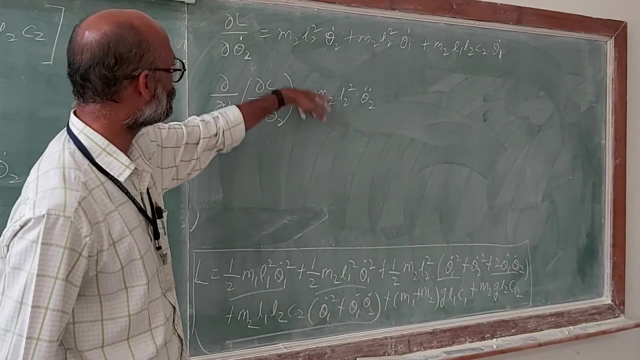 is del l by del theta 2 dot. so we need to differentiate this equation with respect to time. so that is simple: m 2 l 2 square theta 2 double dot. that is, with respect to time. we have done so this equation with respect to time: cross term: m 2 l 2 square theta 2. 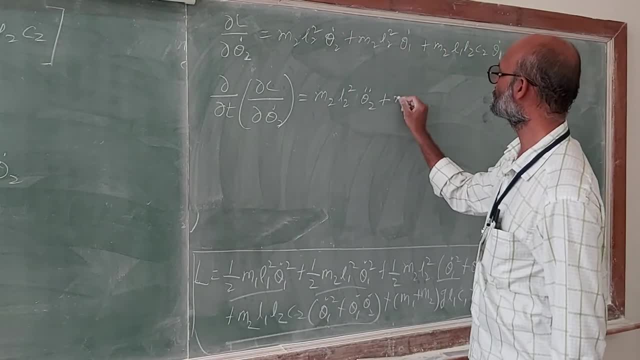 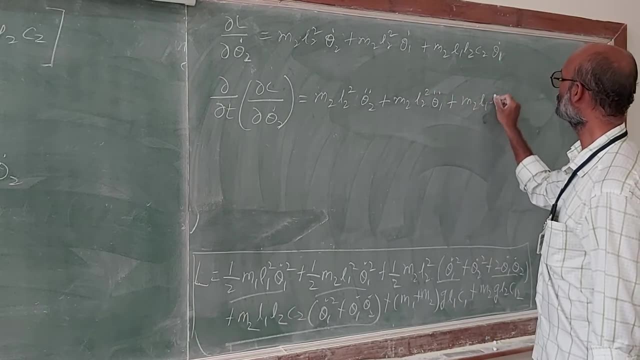 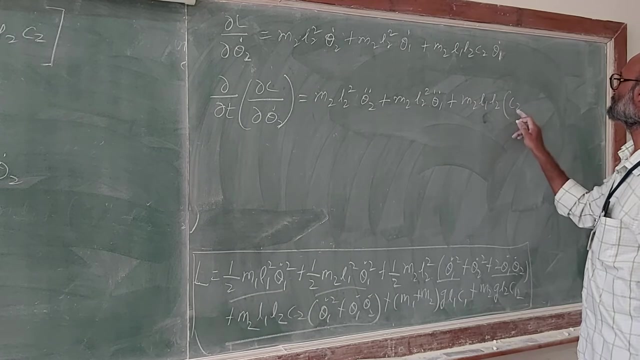 double dot and plus differentiation of this: m 2, l 2 square theta 1, double dot plus we have m 2 l 1, l 2. this is product of two functions, so I will use a small bracket here. c 2- differentiation of this is using product rule c 2. 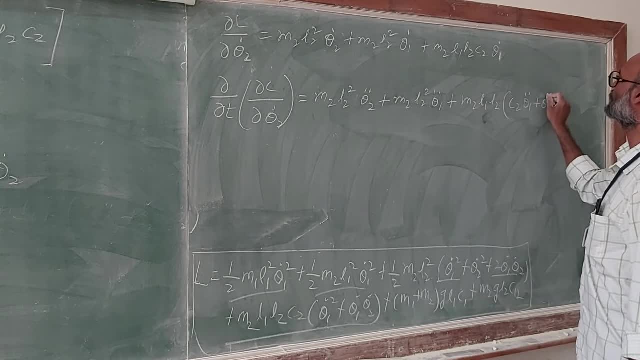 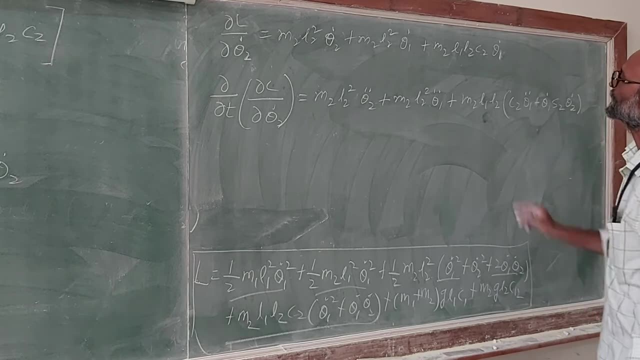 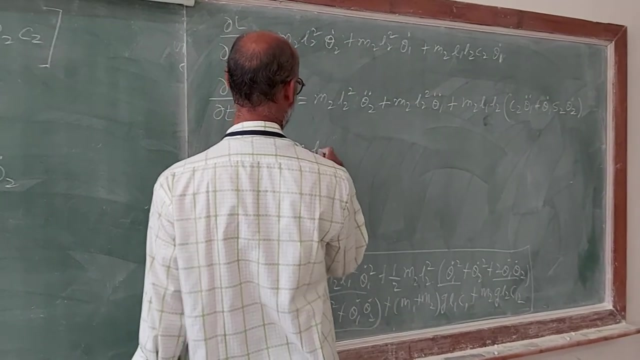 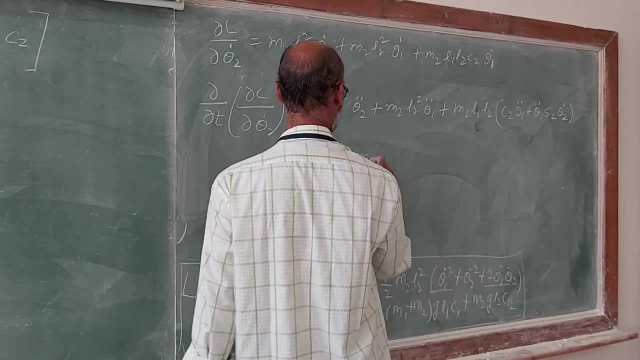 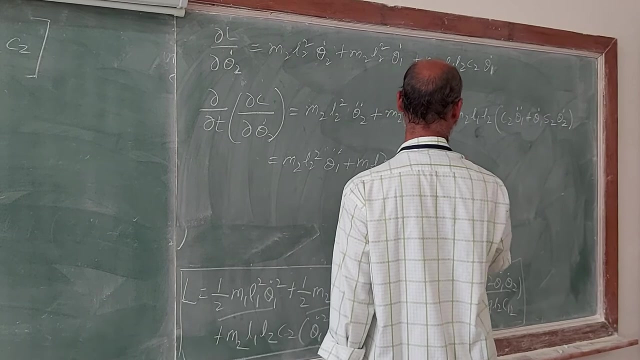 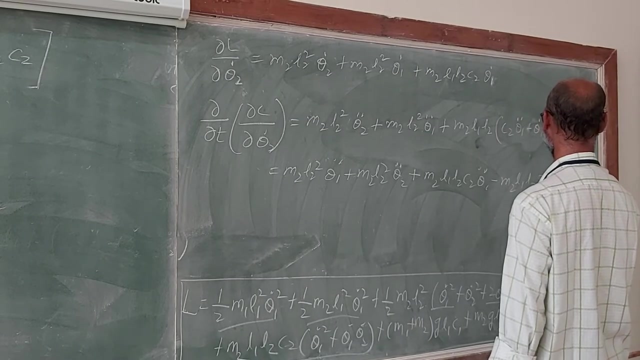 theta 2. I am writing this term plus plus. m2 l2 square theta 2, double dot plus. I will just expand this: m2 l1 l2 c2 theta dot, double dot. that is the first term, minus m2 l1 l2 s2 theta. 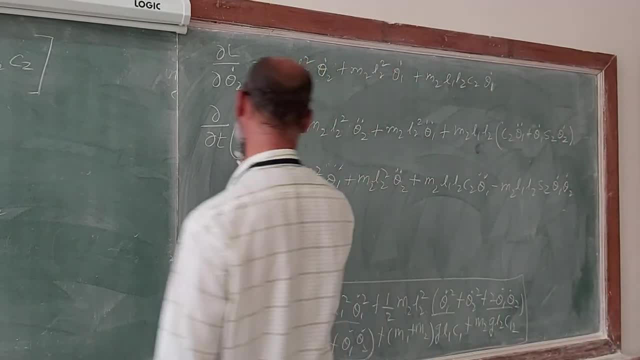 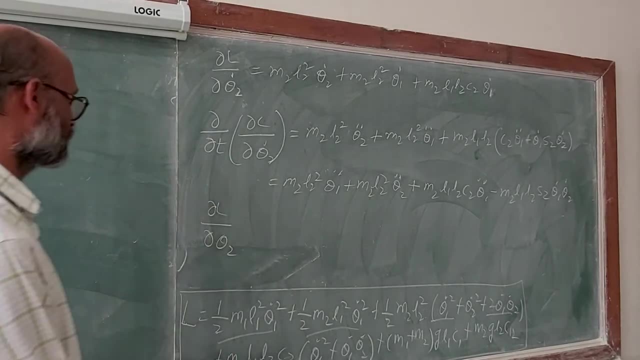 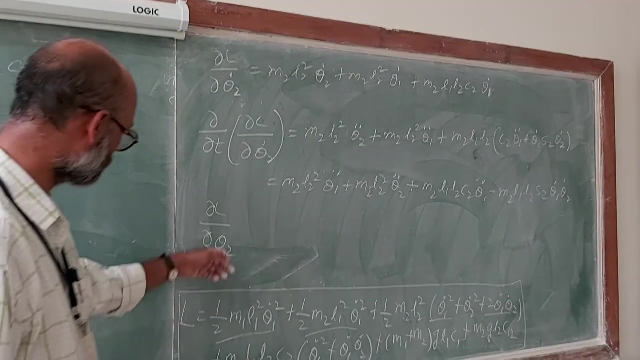 per dot theta 2 theta. This is: this is del y del t. Now we have the final term del y del theta 2.. That is the last differentiation we need to do to get the second equation. So this is the first equation. Second equation: we need to differentiate only with respect. 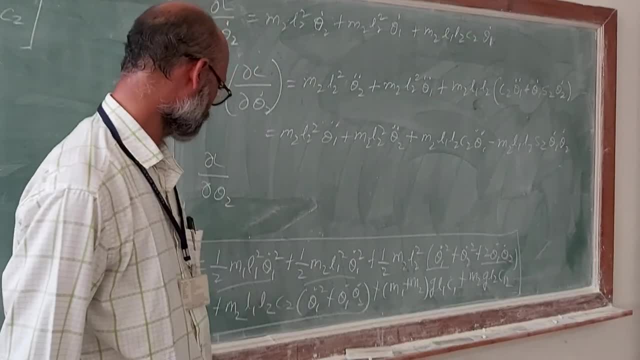 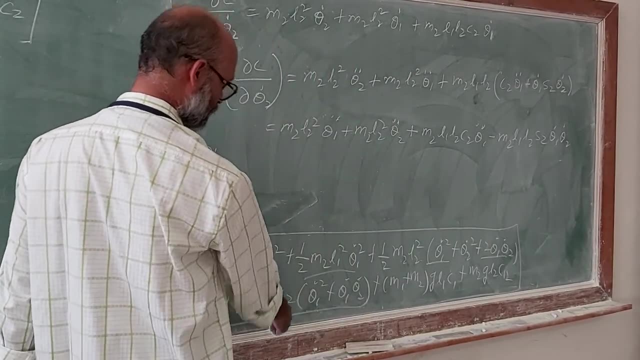 to theta 2.. You can just see, here there is one theta 2 here. You just see that there is no theta 2 over here. The all theta 2 dots are theta double dot. Only theta 2 is here and the last. 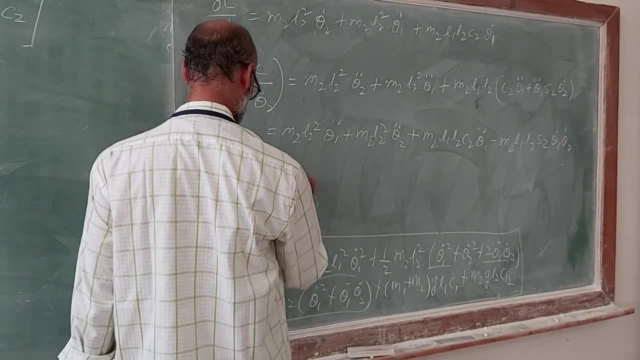 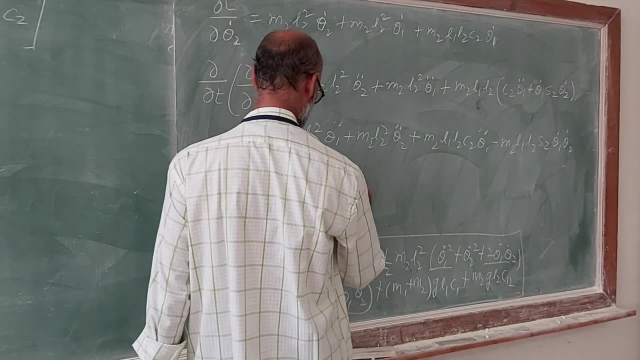 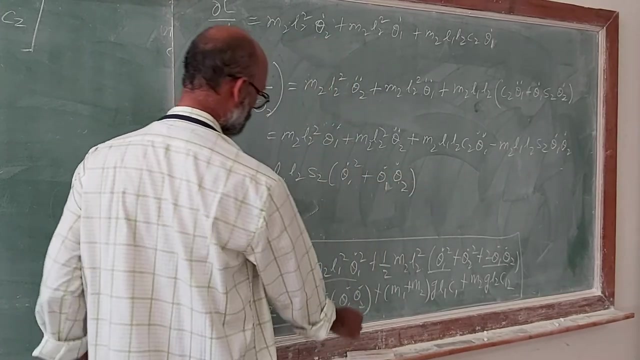 one. So what we have here this is m2, l1, l2.. Definition of this is minus s2.. So you will remain with the two things as it is: theta 1 dot. theta 2 dot, These two terms. 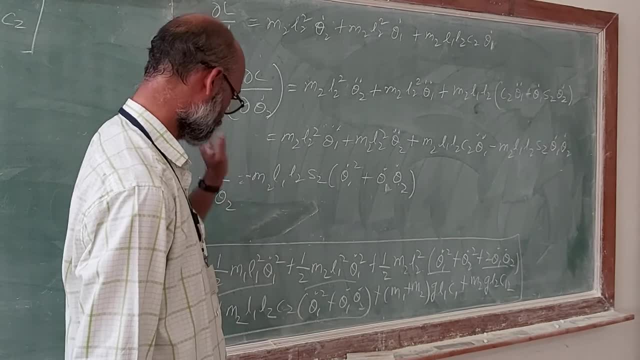 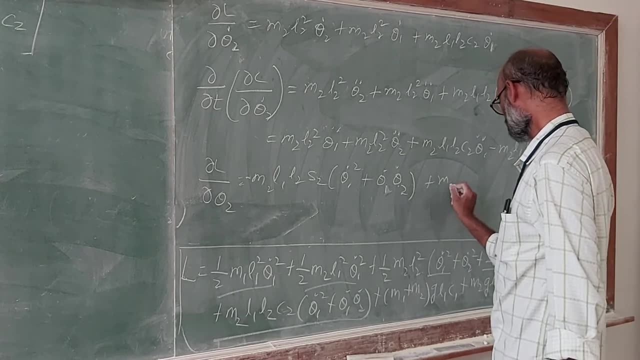 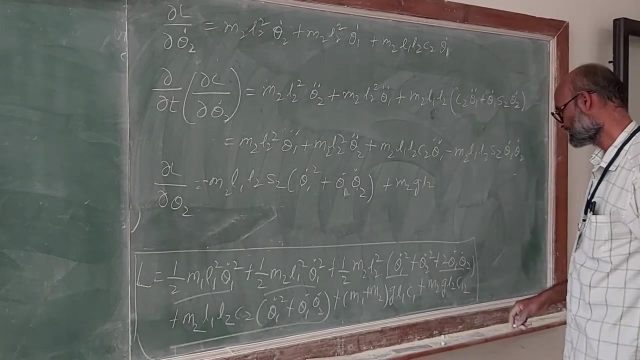 I have kept as it is. Definition of this is: C2 is minus s2.. And again, you do not have s theta 2 here, you have theta 2 over here, So we have that y plus- I use this- plus m2, g, l2.. Definition of c1: 2, I think I have. 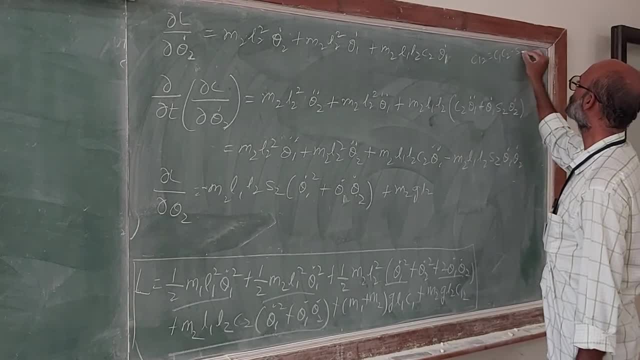 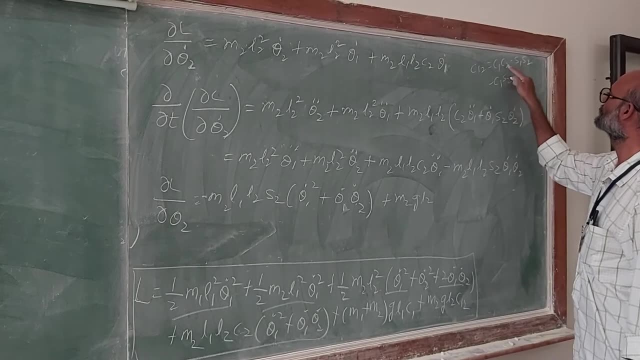 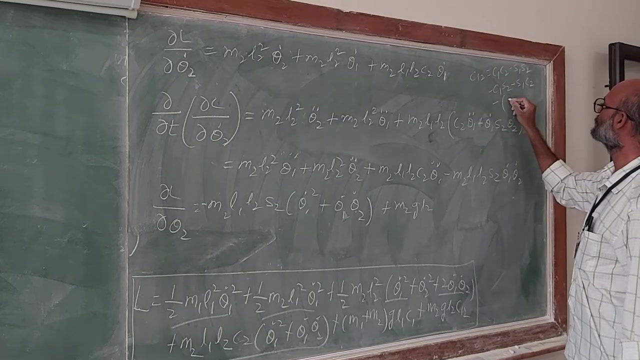 written: c1- 2 is c1, c2 minus s1- s2.. You differentiate with respect to theta 2, this becomes c1 minus s2.. Definition of c2 is minus s2.. We have taken minus out. This will be c1- s2 plus s1- c2, which is nothing but s1 with a. 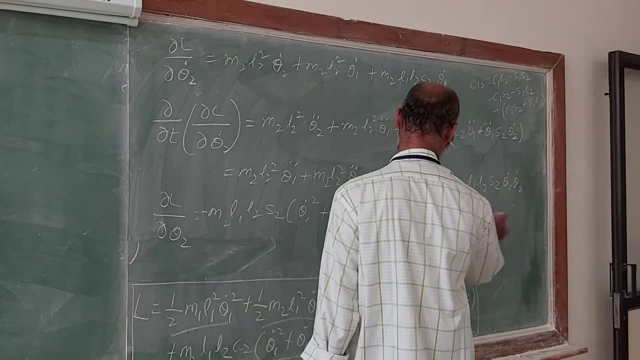 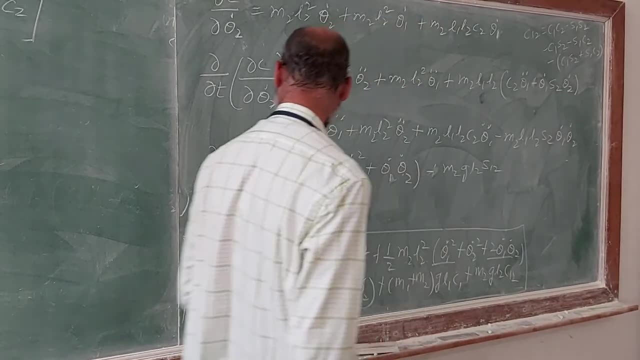 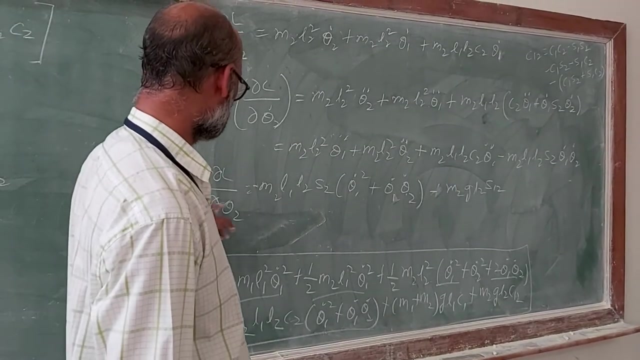 minus here. So that minus I will take here. This is minus s1.. So this s1, 2 I have written here, but the constant from this is s1.. So now you can write the total final equation, t2 equation which I have written here. So del by del, t2 is with a minus. here I have written: 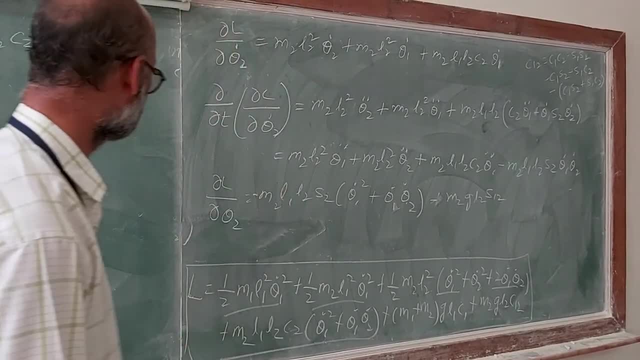 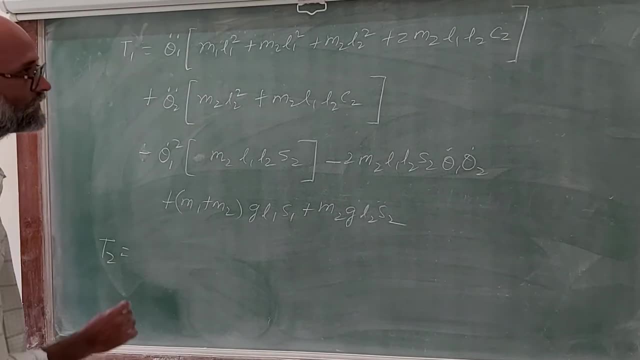 and I will get this equation. minus this equation will get 2.. What is this? T2.. So we write here: T2, this is equal to what is that? one First term: M2, L2 square and theta 1 double. 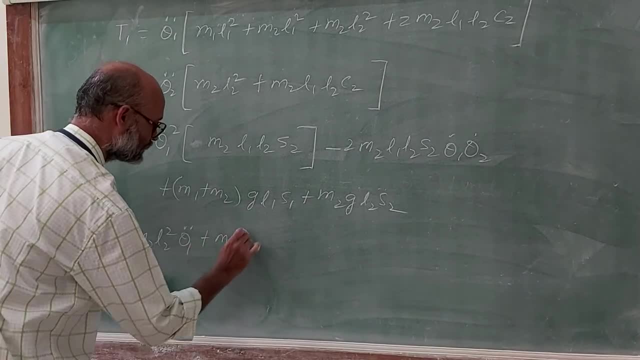 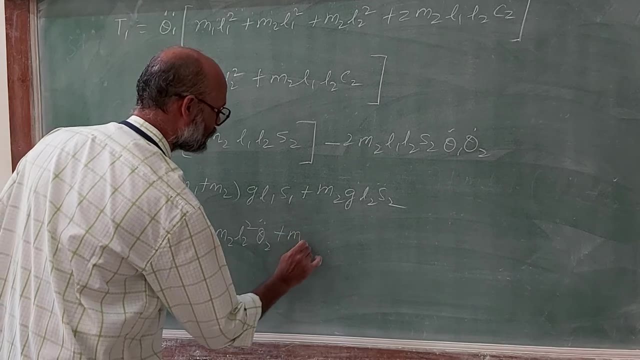 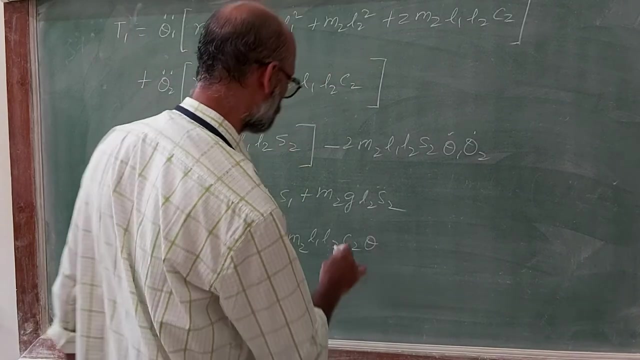 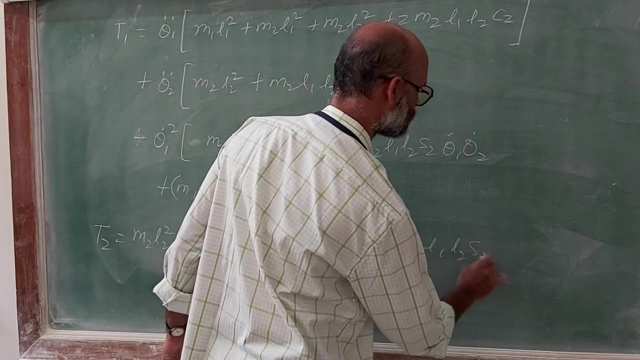 dot term plus M2 L2 square. theta 2 double dot plus M2 L1 L2 C2. theta 1 double dot minus M2 L1 L2 S2, we have theta 1 dot into theta 2 dot, That is. 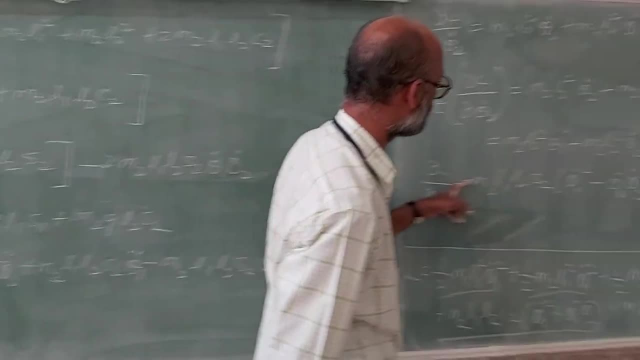 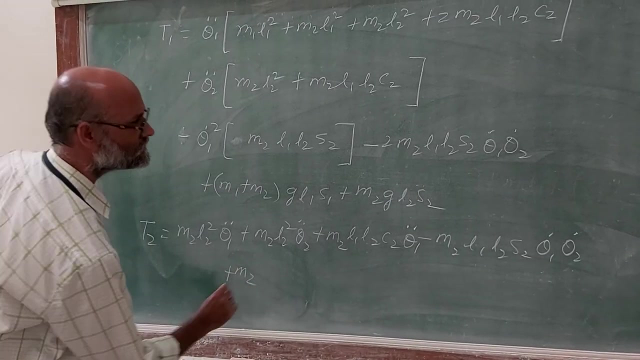 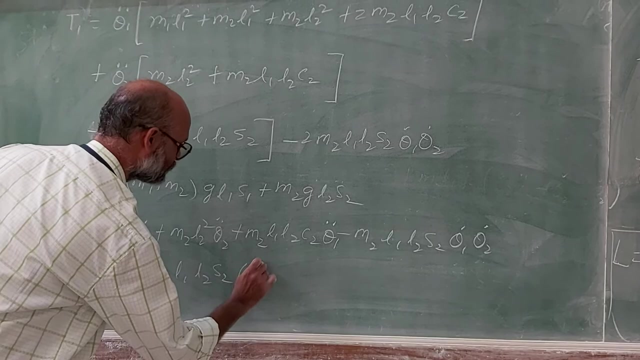 That one Minus of this is equal to minus. this becomes plus, that becomes plus because this is minus. that This is plus M2, L1, L2, S2.. So we have that theta 1 dot square plus theta 1 dot, theta. 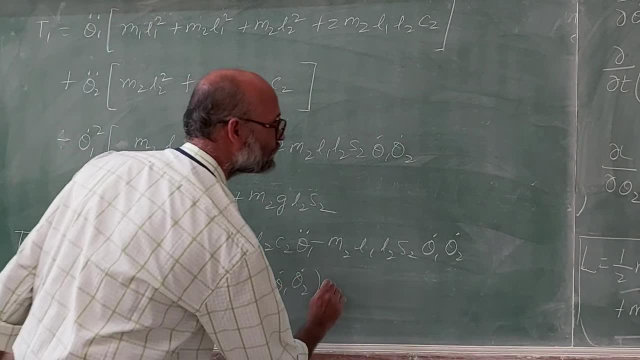 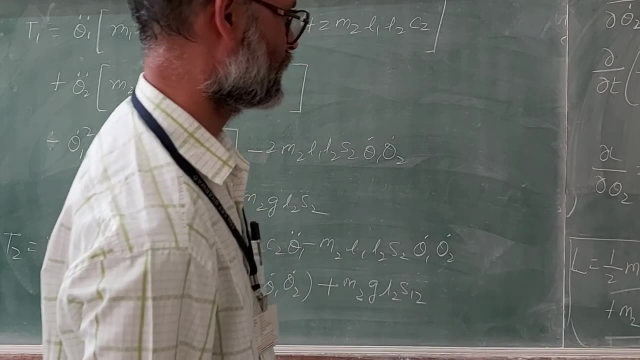 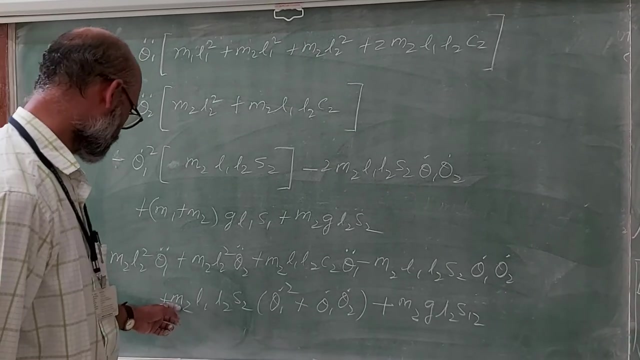 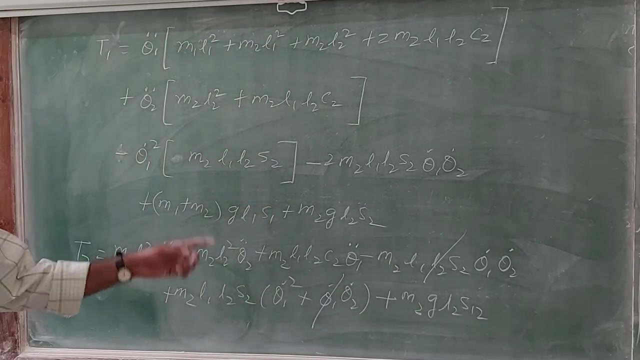 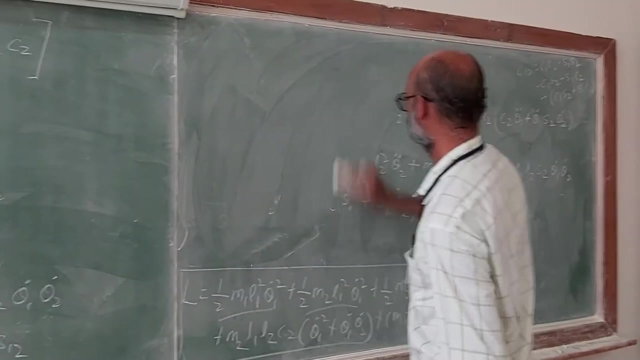 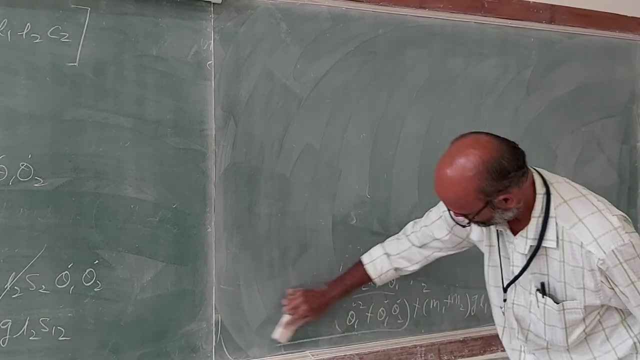 2 dot and we have plus M2, G, M2, L1, L2, S2, theta 1 dot. this is minus this term and this term will vanish. remaining thing. I will just rewrite and finish it out. So what is the T2 log here? Hope you have understood what I have done here. This is minus. 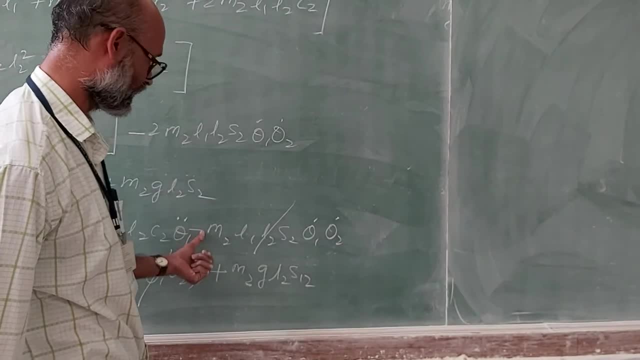 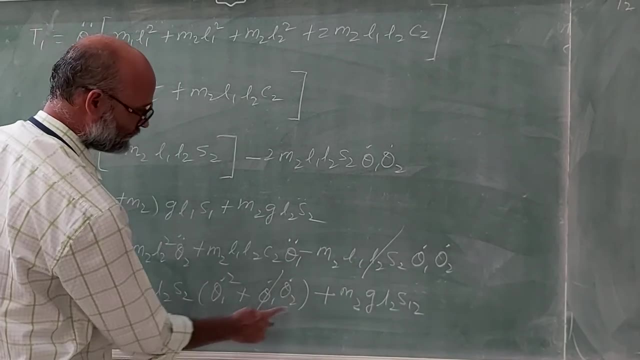 M2, L1, L2, S2, theta 1, dot, theta 2.. This is the minus sign. If you expand this, you can see here: M2, L1, L2, L1, L2, S2, theta 1, dot, theta 2 dot. this is plus, this is minus. so I have. 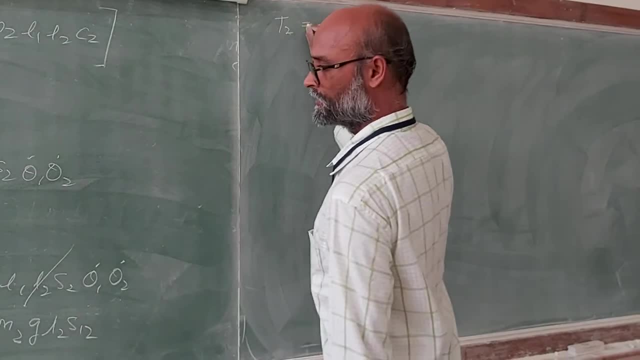 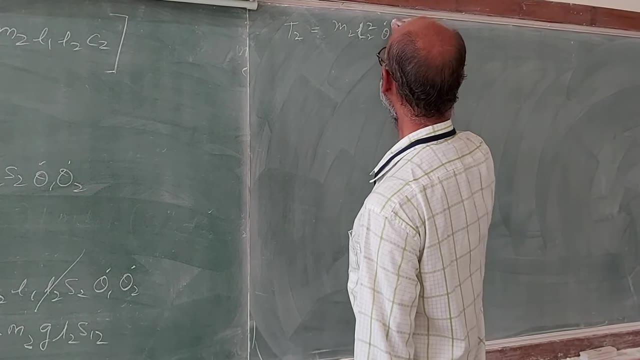 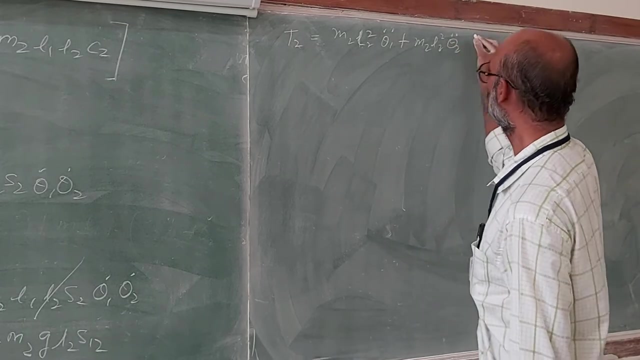 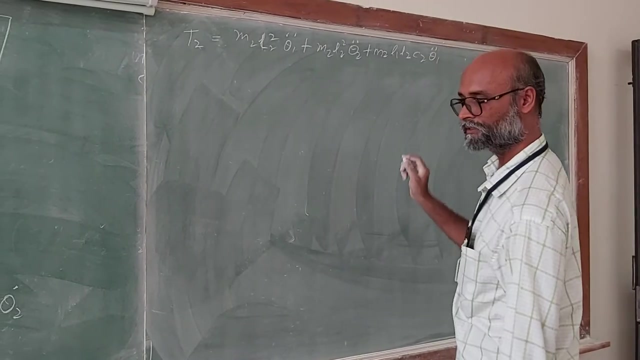 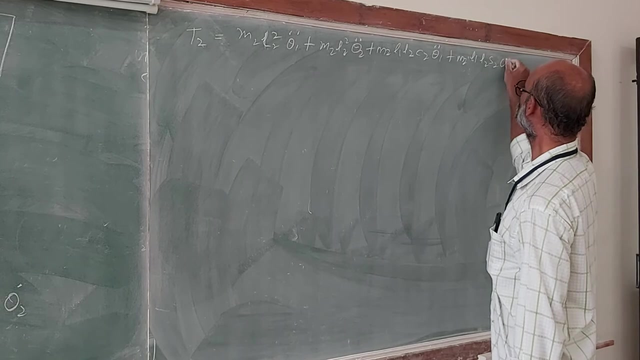 just eliminated. What about P2?? So we have M2 L2- square- Theta 1- double dot, plus M2 L2- square- theta 2- double dot, plus M2 L1- L2- C2- theta 1- double dot, and that vanishes out. Plus we have M2 L1- L2- S2- theta 1 dot square. that is from this. 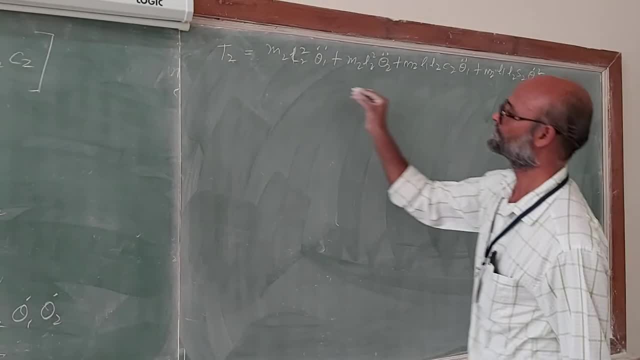 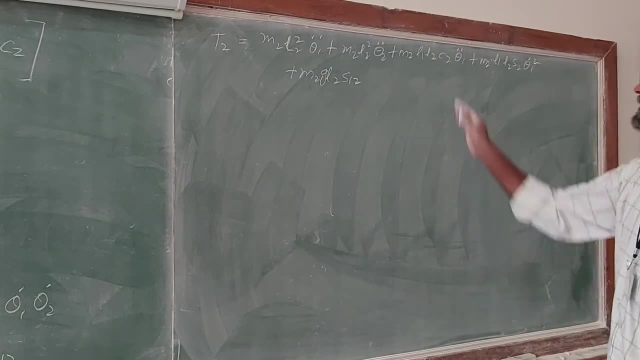 term S2.. Similarly, you have that I just write here that is plus M2 G, L2, S1. So that is this equation can come by like terms like what I have done there. So P2, you write those. 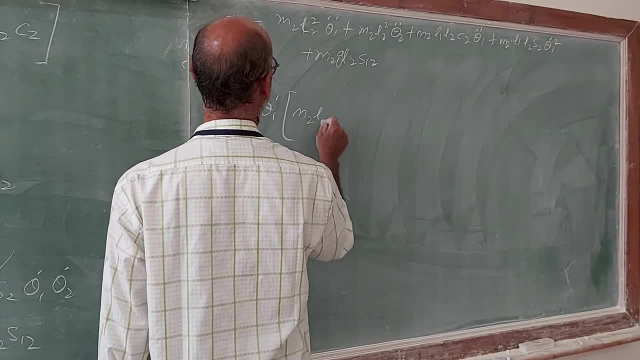 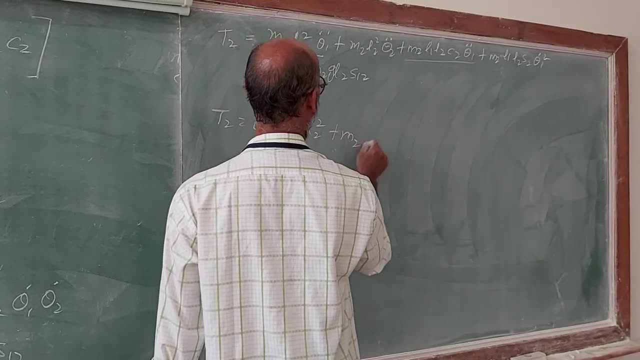 theta 1 double dot terms. so that is M2, L2 square. theta 1 double dot is here and here also is there plus M2 L1, L2, C2, I think you do not have here. so that is your theta 1,. 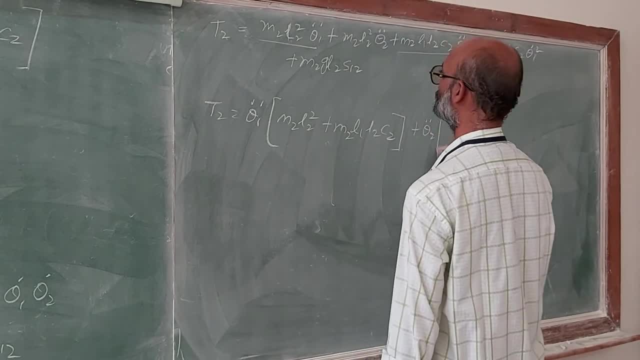 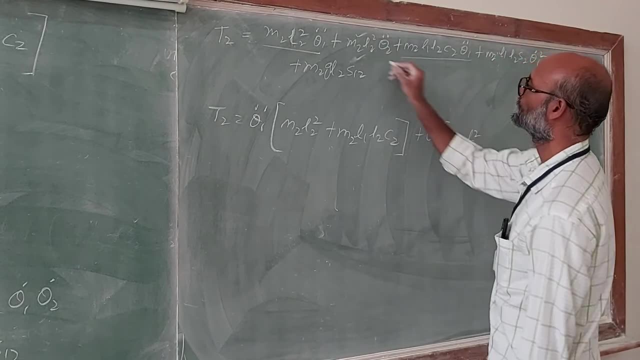 theta 2 double dot terms plus theta 2 double dot terms, you have this one top one. sorry, this is M2 L2 square. So, other than that, you do not have any theta 2 double dot terms plus, you have this so. 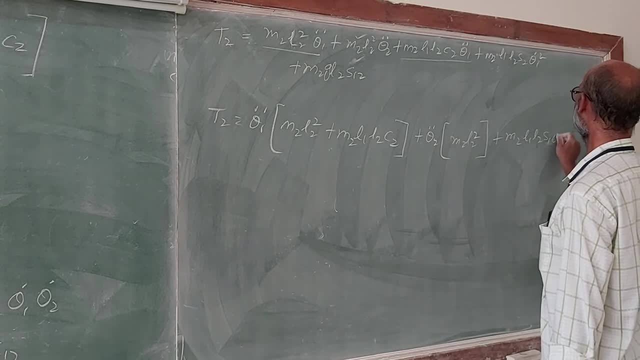 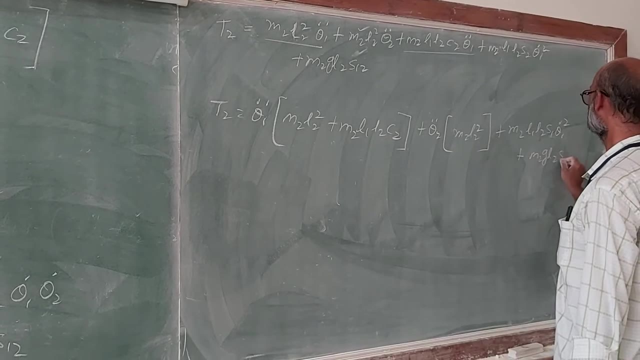 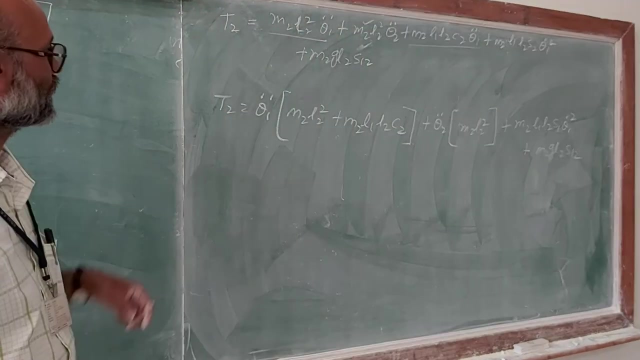 to put it like that, by taking terms M1, L2, S1, theta 1, dot square plus I take it here this term M2 G, L2, S1.. So there are two coordinates, theta 1 and theta 2, two systems, two degrees of freedom. 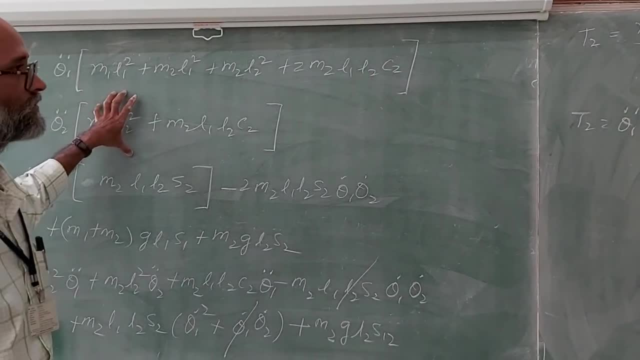 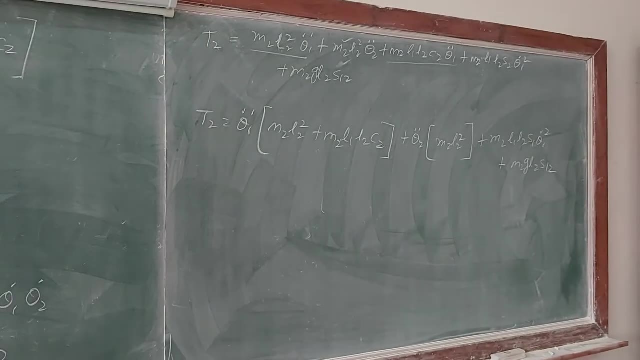 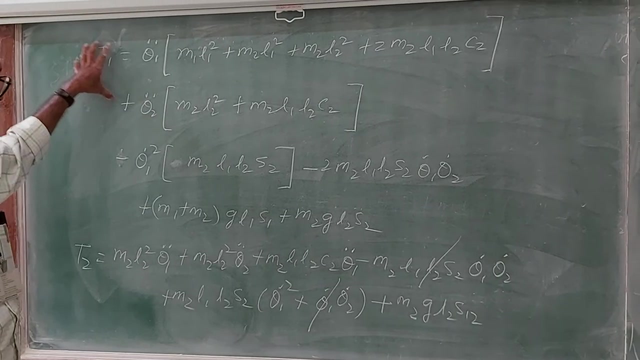 so we know two equations. one equation is defining equation of motion of the first pass. this is the equation of motion, defining the motion for your second pass. you need to write these two equations in a matrix. we need to write this equation and theta equation. we 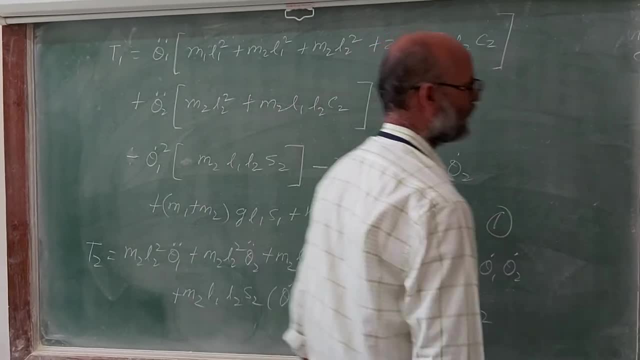 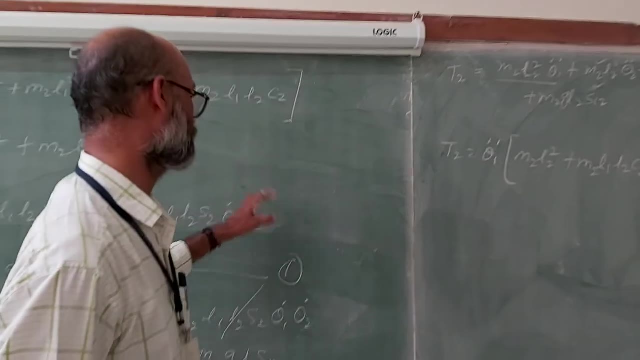 will call this as equation number 1.. and this is equation number 2, so right, we need to write these two equations in a matrix form. so this is little bit bigger one. let us write on the LHS. we need to write your. 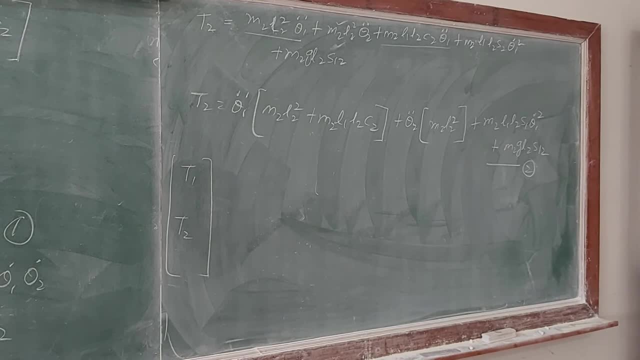 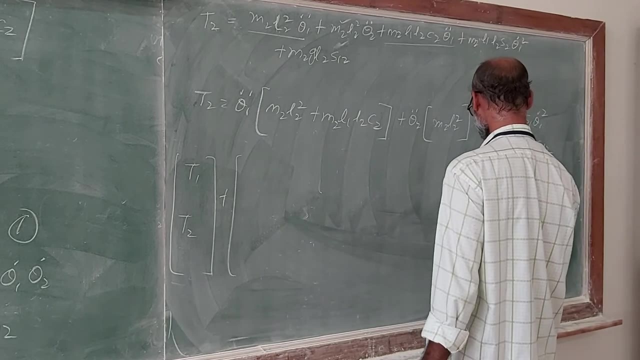 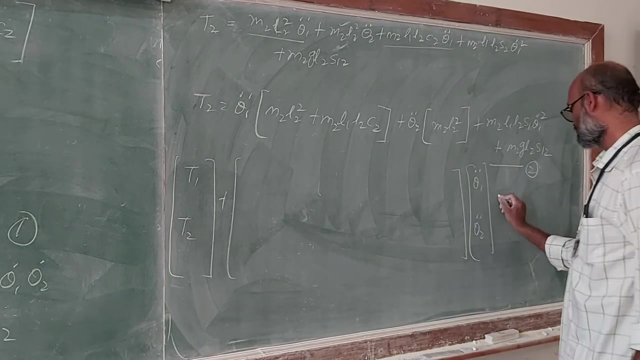 star terms, this is LHS plus some matrix. whatever the matrix you get here into: theta 1 double naught, theta 2 double naught. this is what we need to write plus. so first we will finish up this equation. so I think, hope you can write that I will give it as an assignment. 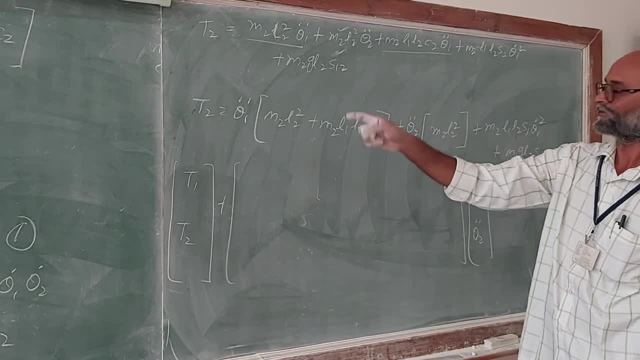 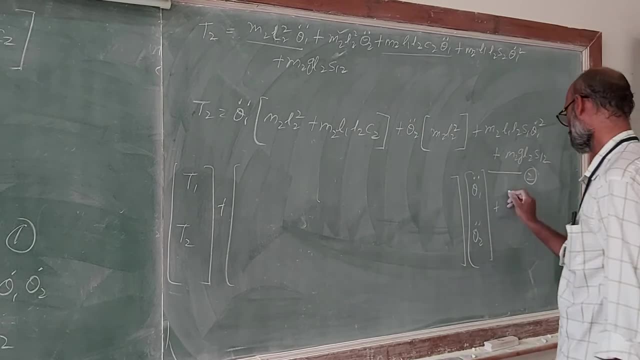 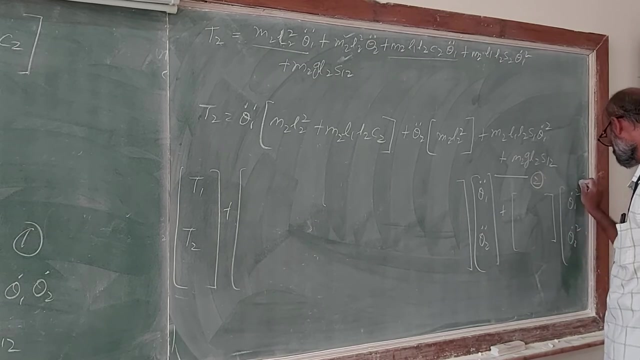 writing this because you already studied in FEM and you can even write equations into matrices, matrices into equations. but I will write the format in which you want to. you need to write it in. so first you have theta 1 dot. theta 2 dot- square. this is the second. 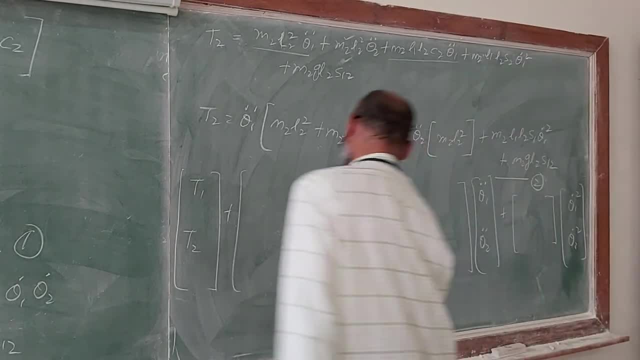 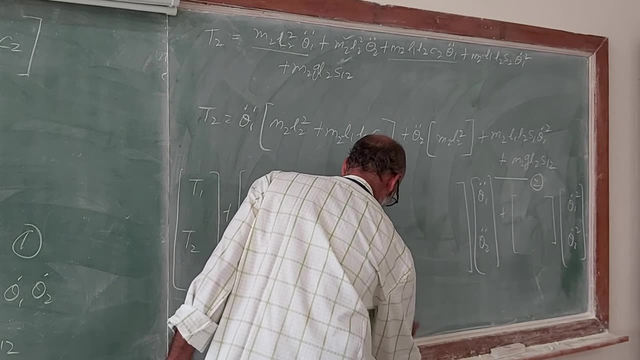 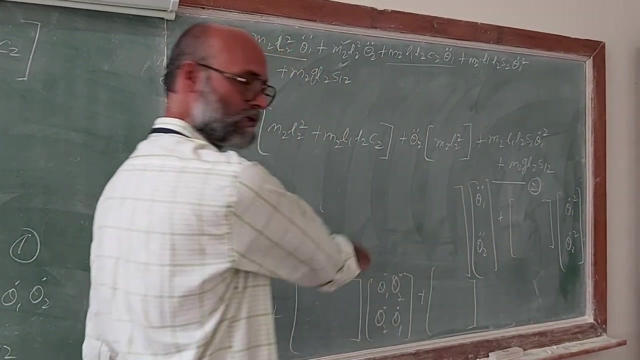 part. this is how you have to write that in two equations plus current matrix. into you have theta 1 dot. theta 2 dot. current matrix should be that plus you have potential terms. so you put it in one matrix. this I will give as an assignment for you. you can just write. 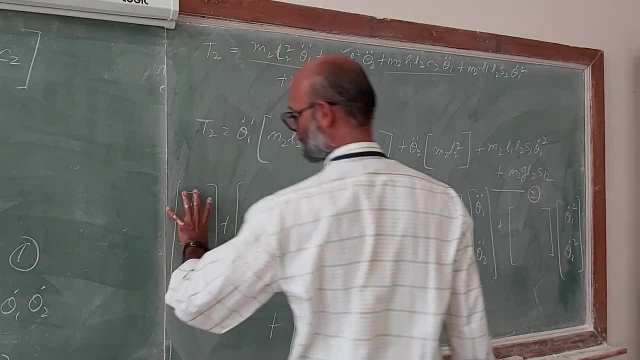 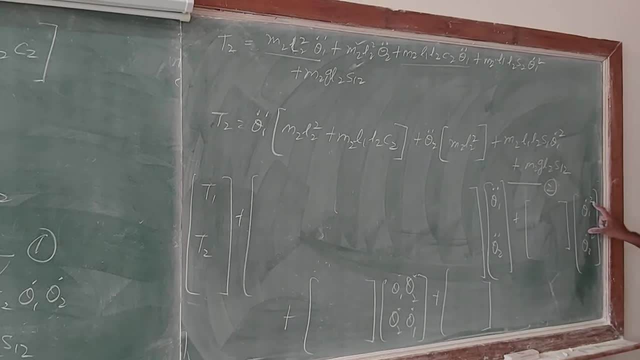 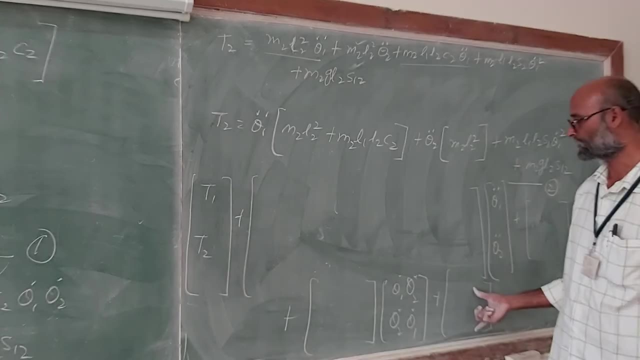 1 double dot. theta 2- double dot terms. next, it is theta 1- dot. square terms. this is theta 1- dot. theta 2- dot. and finally, whatever the terms you need due to the potential energy you have to write here, if you look at this equation carefully, this first one represents: 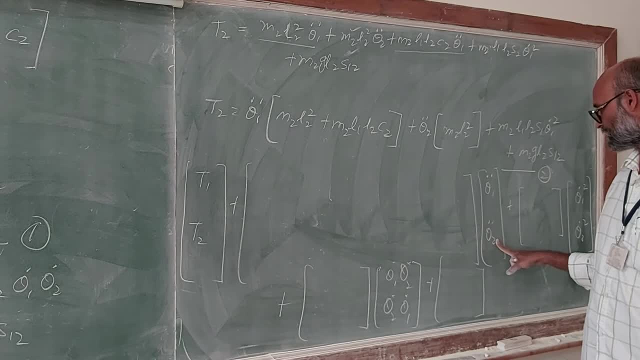 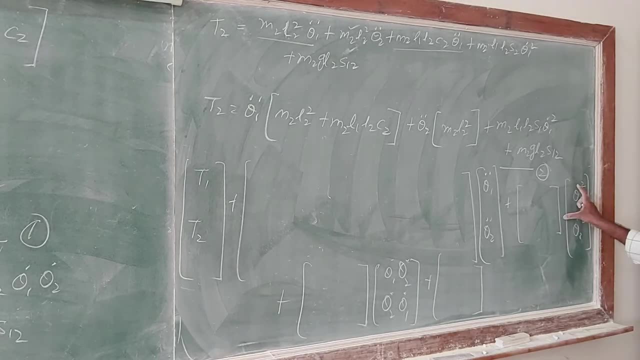 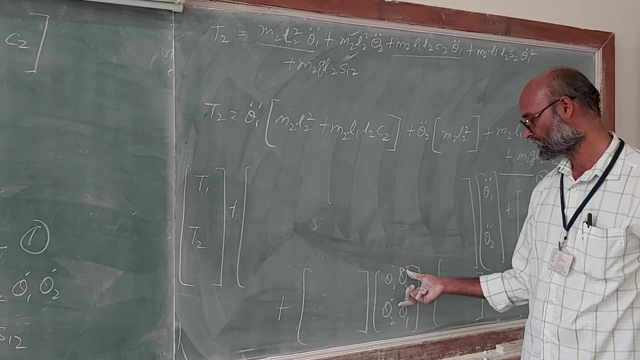 angular acceleration terms. theta 1- double dot. theta 2- double dot represent angular acceleration terms. theta 1 dot square. theta 2 dot square. this represents centripetal accelerations. this term represents centripetal accelerations. if you look at this third term, theta 1 dot. 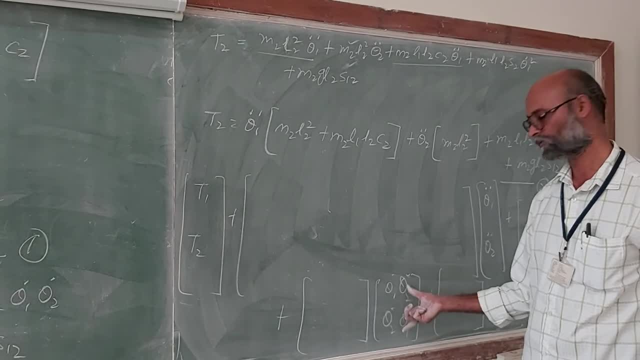 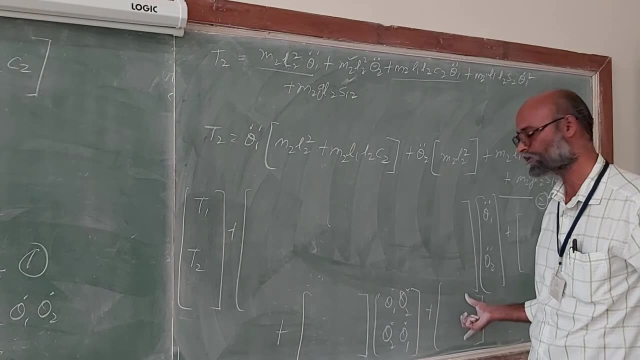 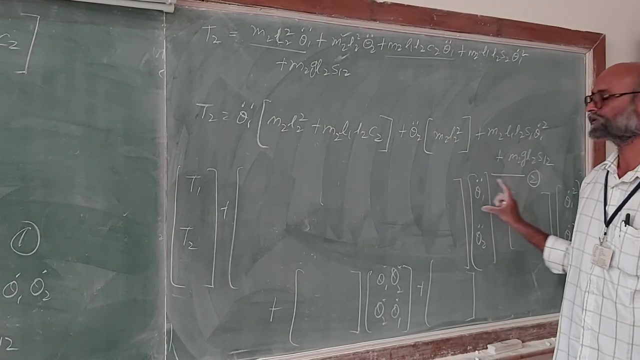 theta 2 dot. this represents Coriolis acceleration. so we have discussed what is Coriolis acceleration in our last class. so this will give you Coriolis acceleration. this is terms due to potential, so you need to write whatever the equations of motion in this form, only first angular. 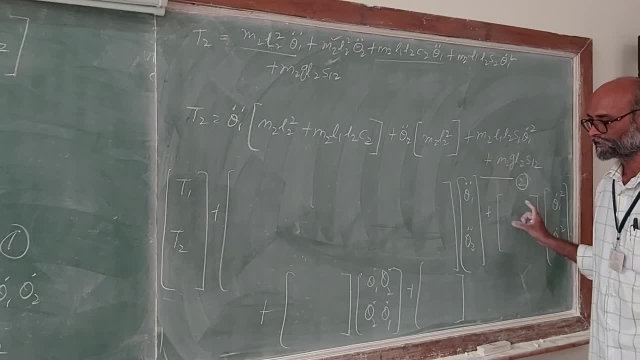 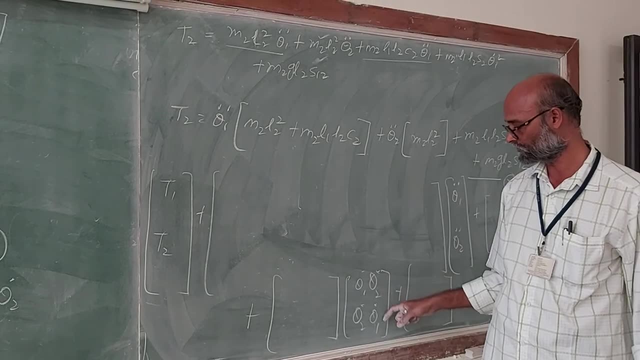 acceleration should come, then centripetal acceleration, then Coriolis acceleration, then your potential term, please note: Coriolis acceleration has come because there is a relative motion between two masses. if mass 1 is here and mass 2 is here, mass 2 is affected by the acceleration. 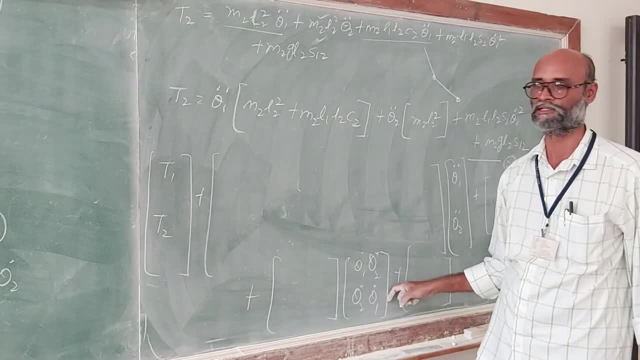 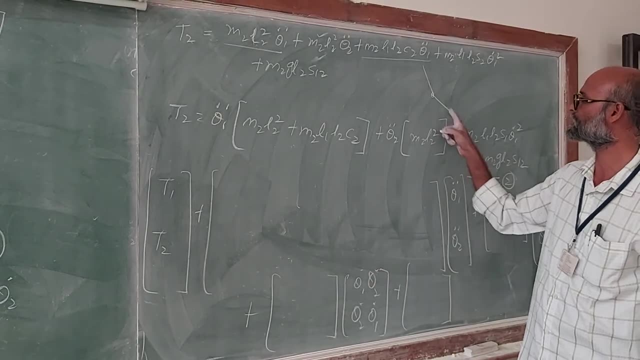 of mass 1. that is why we get this Coriolis acceleration. in our previous example, which I have done in the class, we did not get this type of terms. so we get here because you have a relative motion between two masses. so we will stop here, we will continue in another.